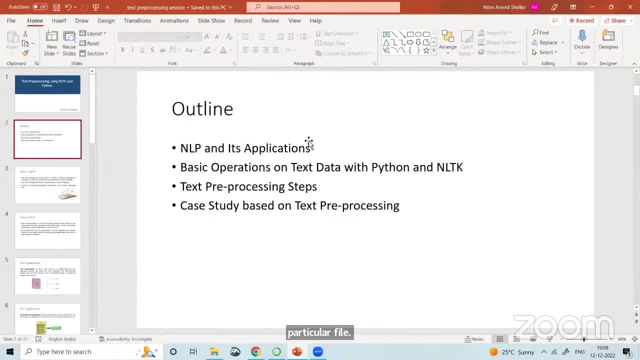 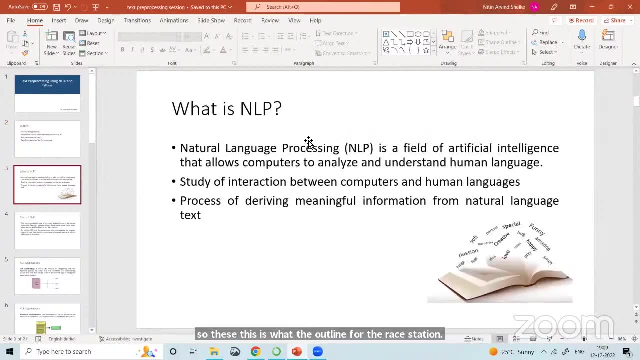 on the particular file. Okay, so this is what the outline for the today's session. Now let us start with the first thing, that is, NLP. So NLP, it is a natural language pre-processing or natural language processing, which is a. 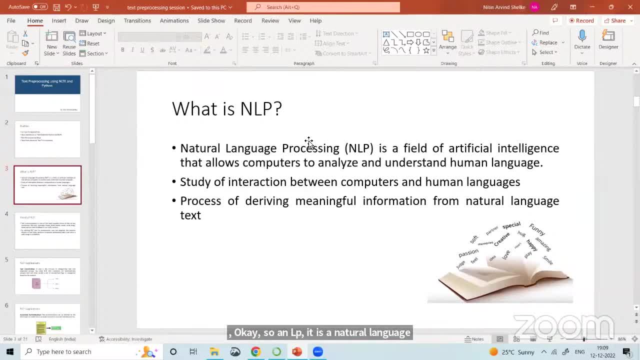 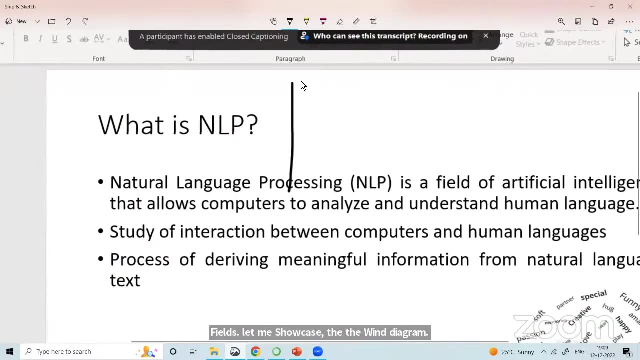 field of artificial intelligence, The broad domain is AI, under which we have several fields. Let me showcase the Venn diagram. So when we consider the artificial intelligence, the broad domain is artificial intelligence. Under that we have machine learning, deep learning. 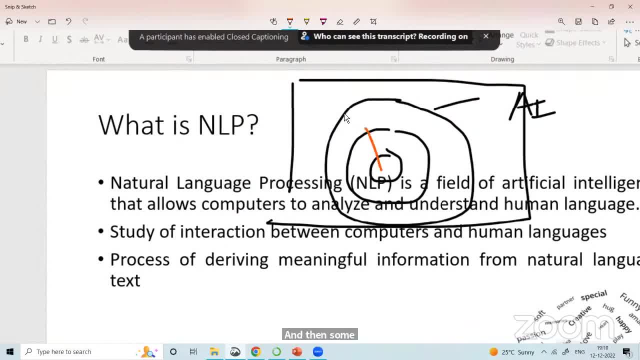 And then some components. Some components, Some other fields, like natural language processing is get attached with the AI, like image pre-processing, image processing is get attached. So this is our NLP, which we can say that is included under the AI: machine learning. 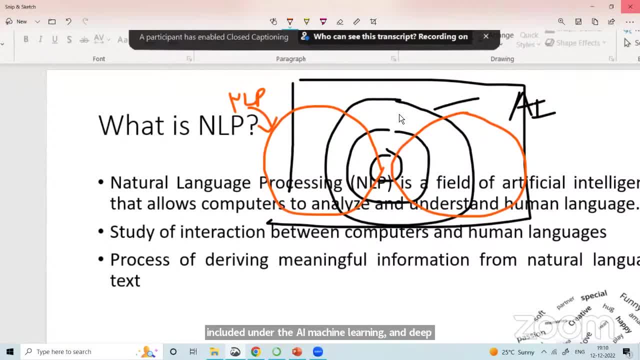 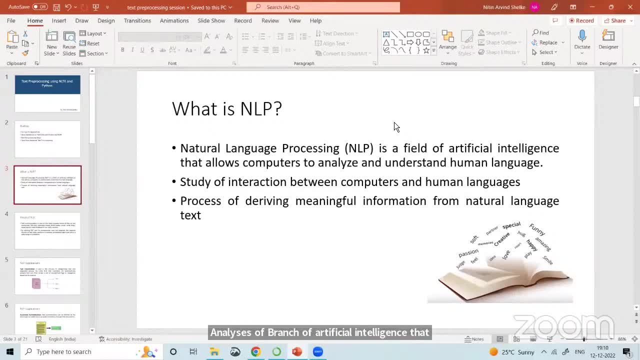 and deep learning association with all these fields. So NLP is a branch of artificial intelligence that allows the computer to analyze and understand the human language. So we can say it is an interaction between the computer and human language And with the help of this NLP, it is a process of deriving the meaningful information from. 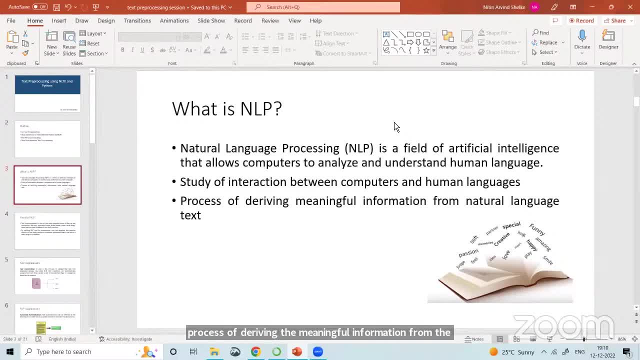 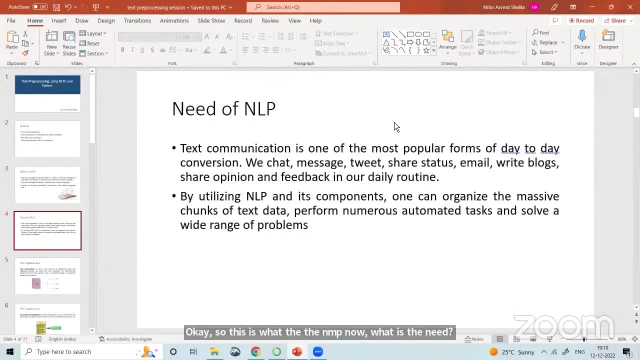 the natural language text. Okay, so this is what the NLP. Now what is the need? So nowadays, we know that everyone is going to post the message, chat regularly, share the status, write the email, write the blog. So what is the need? 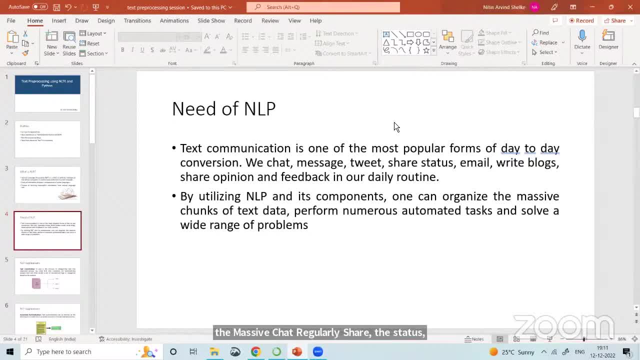 So nowadays, we know that everyone is going to post the message chat regularly, share the status, write the email, write the blog. So what is the need? So nowadays, we know that everyone is going to post the message chat regularly, share. 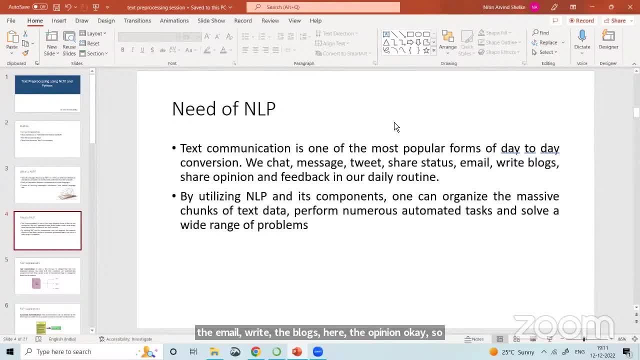 the blog. share the opinion? Okay, So the text communication is nowadays one of the prominent form of the day-to-day conversion. So where there is the involvement of the text data, there we require the natural language processing, Even for the speech recognition or the human language in the form of audio or video. 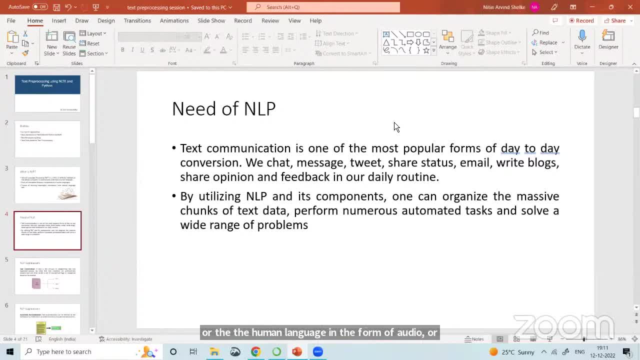 Okay, So that time also, they required the use of NLP in order to convert the language into the text and then perform certain operations. By utilizing the NLP and its component, we can organize the massive chunk of text data and perform the several automated tasks. 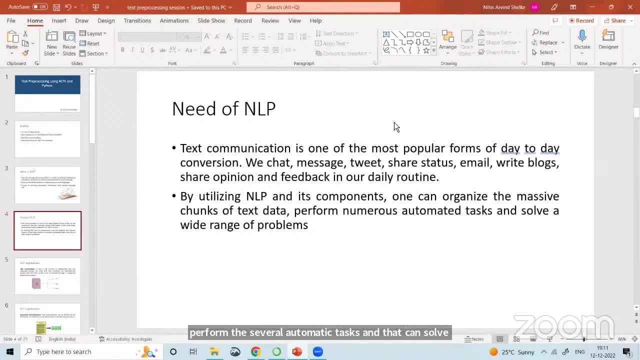 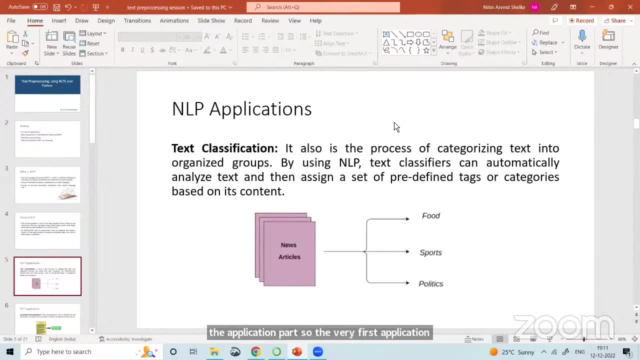 And that can solve the wide range of problem that we will discuss under the application part. Okay, Okay, So the NLP it is text classification, So it is the process of categorizing the text into the organized group. Okay, So say, suppose you have the collection of text data, okay, 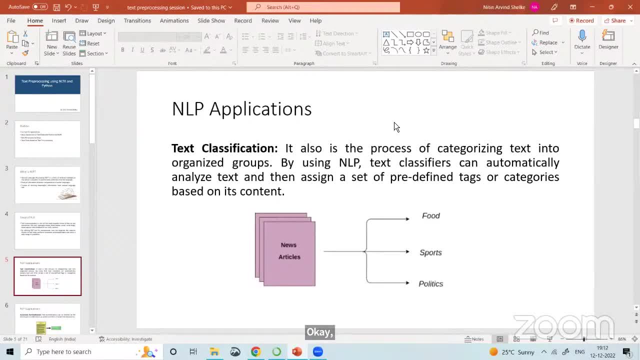 And, like news article, we have under the news article there are several types of news. Okay. So with the help of NLP and the AI, you can classify the different text Okay From the news under the food domain, under the sports editorial board: politics, entertainment. 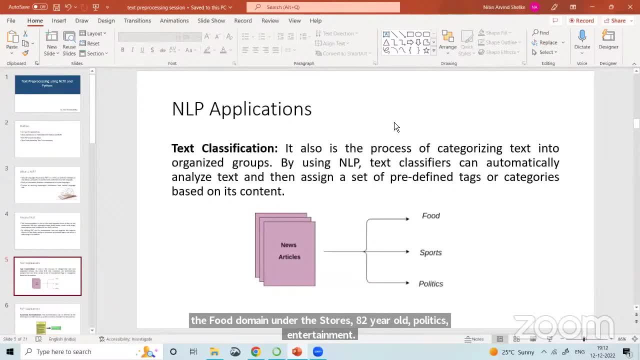 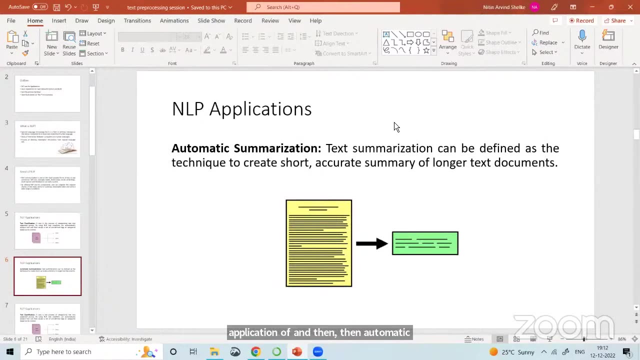 So we can make a group of different text format, different text categories. Okay, So the text classification and text categorization is one of the application of NLP. Then automatic text summarization is another applications where we can summarize the large text into the short. 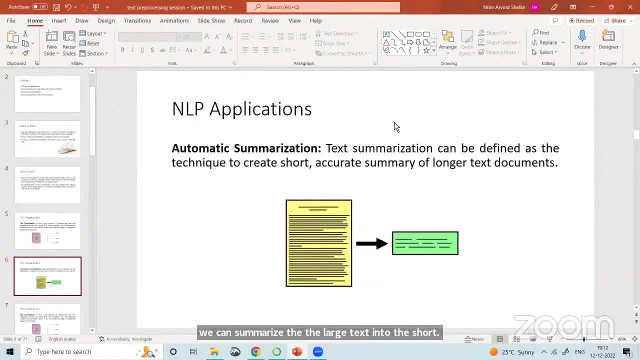 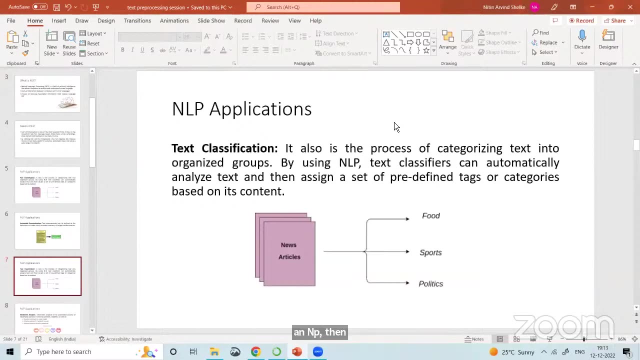 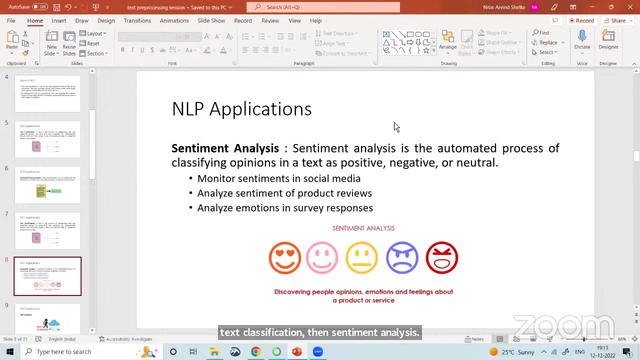 Okay, Longer text document. you can convert it into the shorter text or you can say the kind of abstract. you can get it from the longer text with the help of NLP. Then next application, so that is repeated text classification. Then sentiment analysis is one of the useful application nowadays. 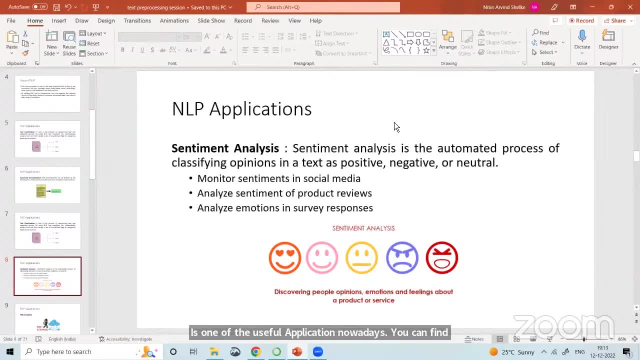 You can find the use of sentiment analysis in a lot many. I mean sentiment analysis is also one area and under that we have several sub domain. like you can apply it in the movie reviews, Then you can apply it in the hotel reviews. 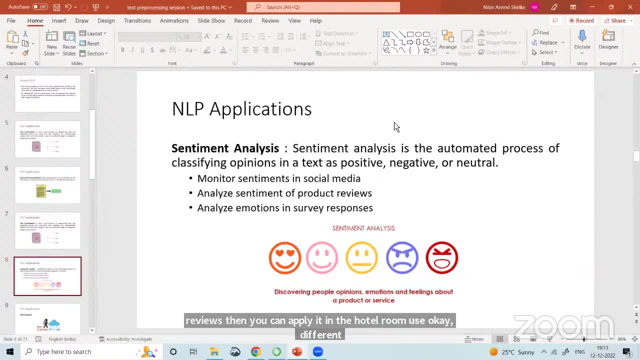 Okay. Different reviews section: e-commerce reviews: Okay, So at different review sections you can apply the sentiment analysis. It is the automated process of classifying the opinion from the text, whether the text is positive, negative or neutral. So we can monitor the sentiments from the social media or we can analyze the sentiment. 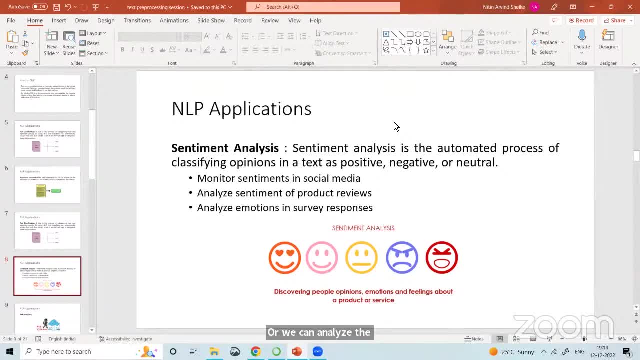 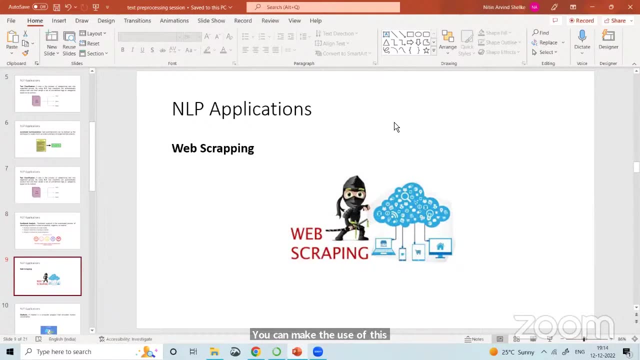 from that, As I said earlier that the broad domain it is again sentiment analysis. We can apply it in the social media: product reviews or survey response and many other places. You can make the use of this sentiment analysis then web scrapping. 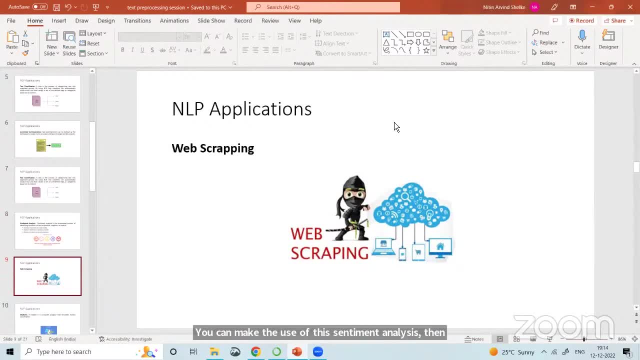 So web scrapping is the extraction of the text data from the web website And then perform certain further, then perform further analysis, whichever you want. So further analysis means you can go for the sentiment analysis, You can go for the information, or you can go for the classification plus stream or the. 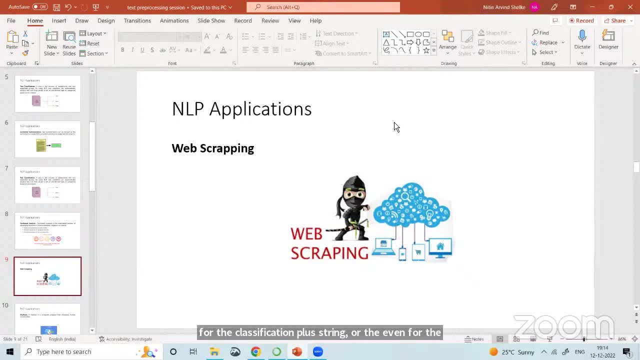 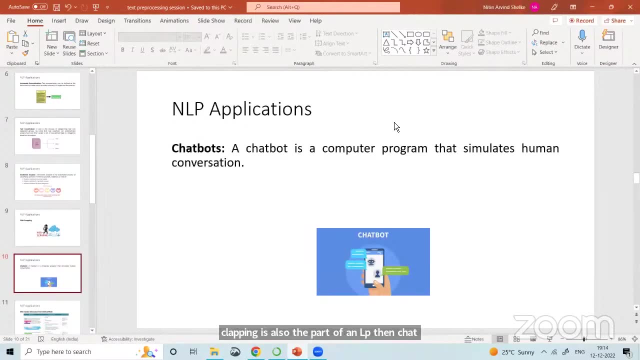 even for the extracting the specific information. Okay, So web scrapping is also the part of NLP. Then chat mode. So you, you all know the chatbot, the importance of chatbot. nowadays we want to replace the human being and with the chatbot and that chatbot can answer the- uh, the questions. 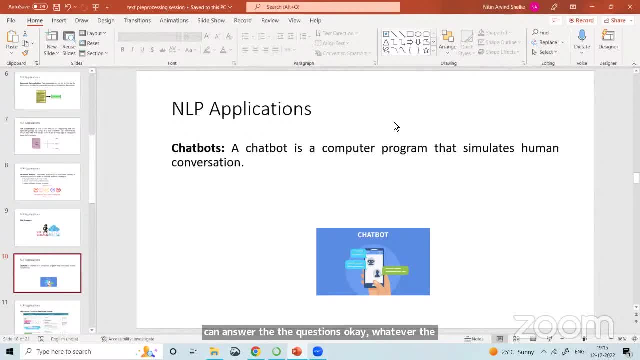 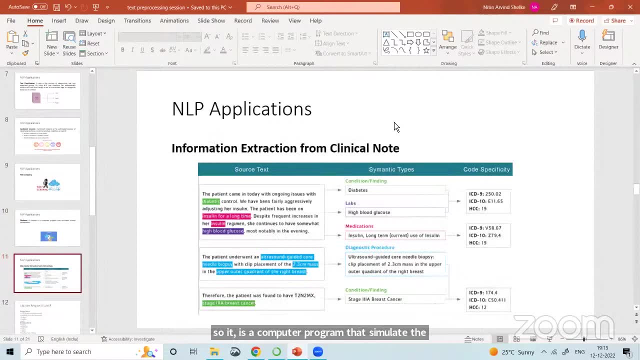 Okay, Whatever the query that you can fire, your chatbot can answer it. So it is a computer program that simulate the human conversation. Then next thing is information extraction from the clinical node. So basically, uh, when the information is placed, uh, as a huge document or in a complex 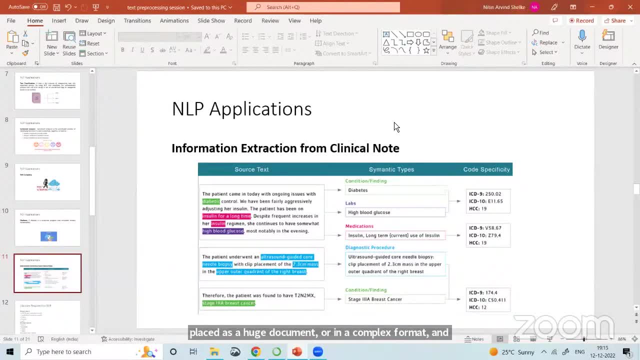 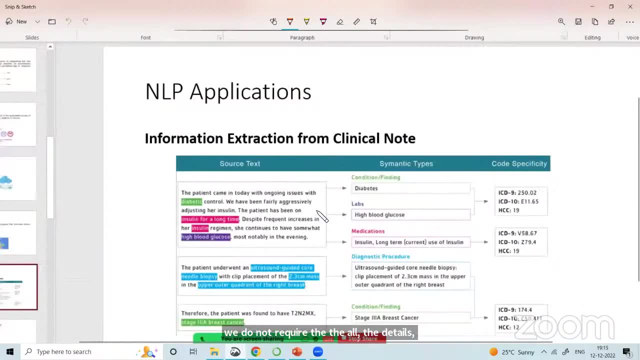 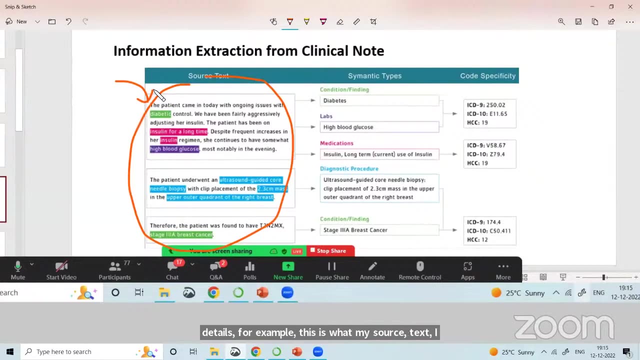 format and we do not require the the all the details specific and we want the specific details. For example, this is what my source text and it is a complicated information, So okay, And we just need the systematic information. 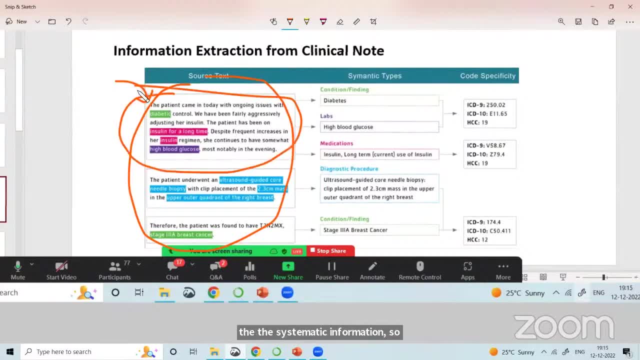 So systematic information means what So say? suppose this is a blog that is related with the medical patients. So what disease it is? So the diabetes? specific information, Okay, So diabetic because of this? uh, worse, we can identify the diseases diabetes and other. 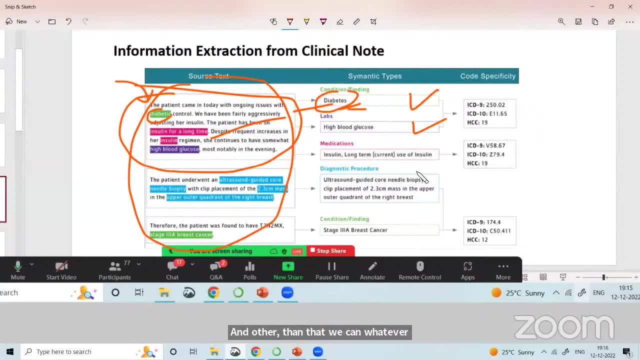 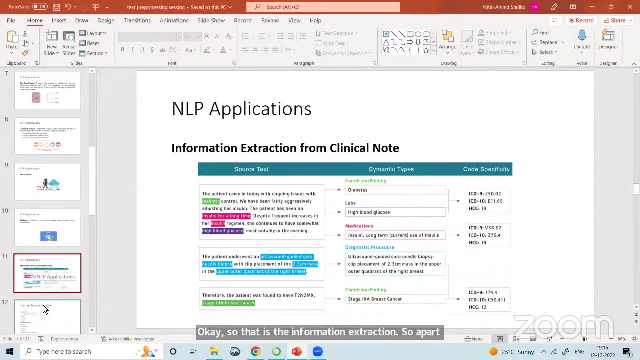 than that. we can, whatever the the parameter that we said, so it can extract the important and useful information from the huge amount of text. Okay, Uh, the information extraction. So apart from that, there are many other users? Okay. 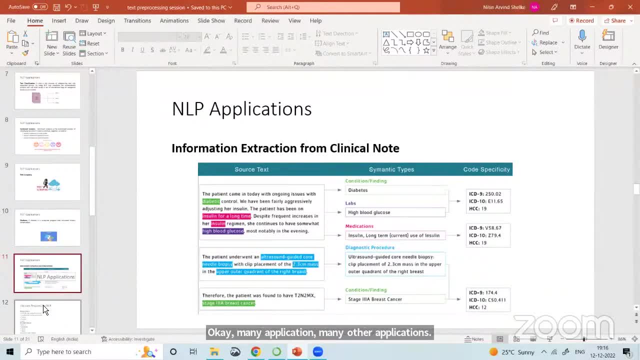 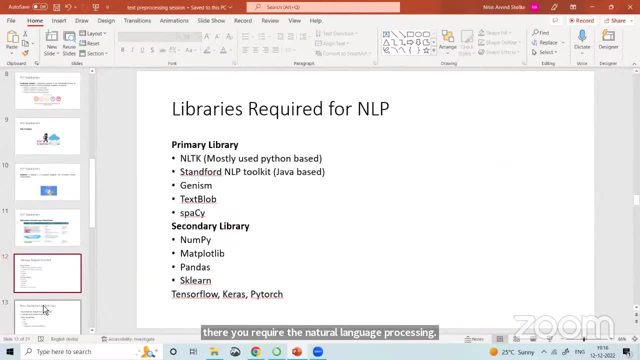 Many applications, many other applications. Okay, So where there is an involvement of the text, data, there you require the natural language processing. Okay, Now the libraries that we required for the natural language processing. there are two libraries for the primary libraries and secondary libraries. under the primary library we have 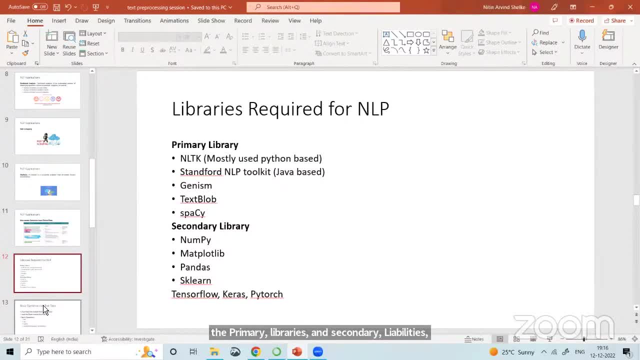 NLTK, which is most commonly used Python based library And that we are going to cover under this session. Other than that, we have another library, Stanford NLP toolkit, which is Java based: Gensim TextBlob- spaCy. 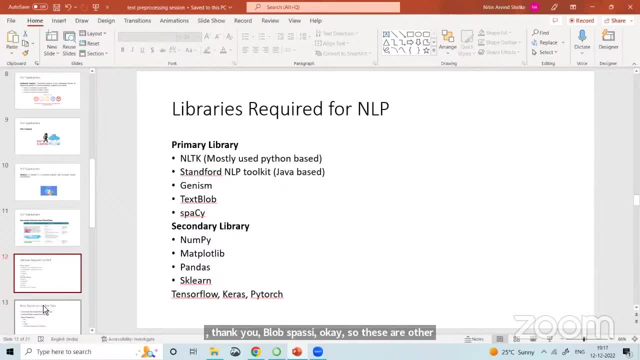 Okay, So these are other libraries that you can consider uh for uh doing the NLP projects, but NLTK is one of the most commonly used library nowadays. Okay Then secondary libraries that we required, So secondary libraries, Nrmpath. 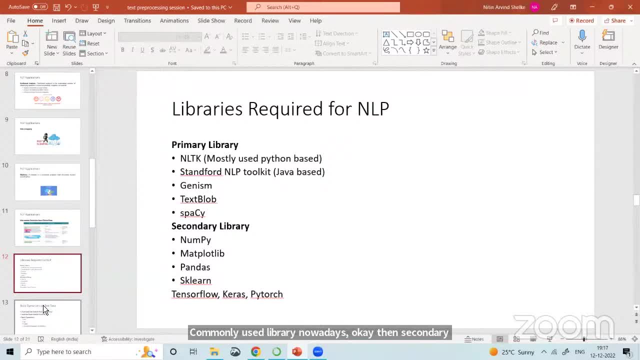 For handling the multi-dimensional headache because, as we know, whatever data that we are going to consider, whether it is a text data, whether it is an image data, whether it is the audio data, whichever the type of data that we have, at the end the processing- 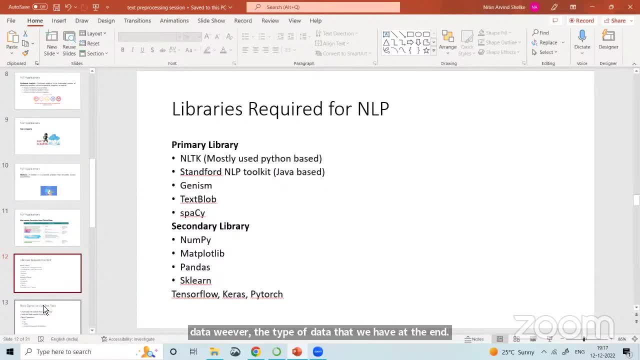 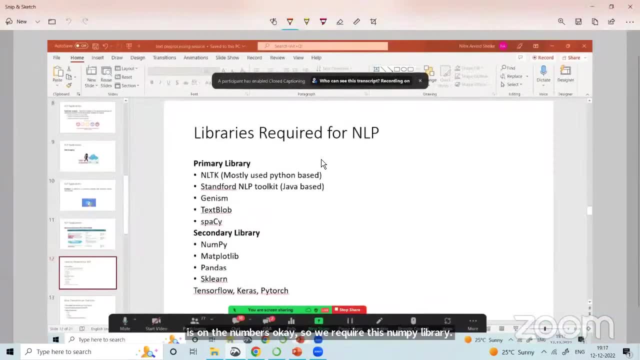 that get performed in the background. it is on the numbers, Okay, So we require this Nrmpath library. Basically, if we have a text data, we can understand it, Okay. Human can understand the text data, but machine cannot understand image, video and audio. 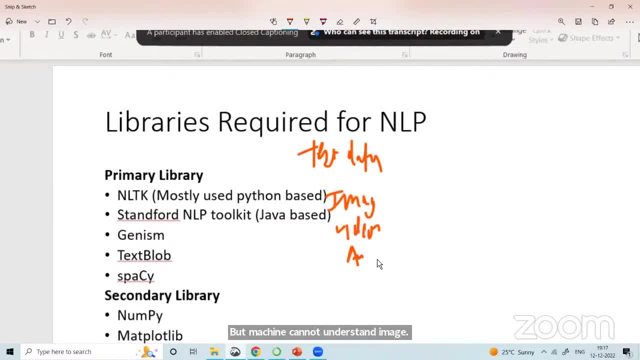 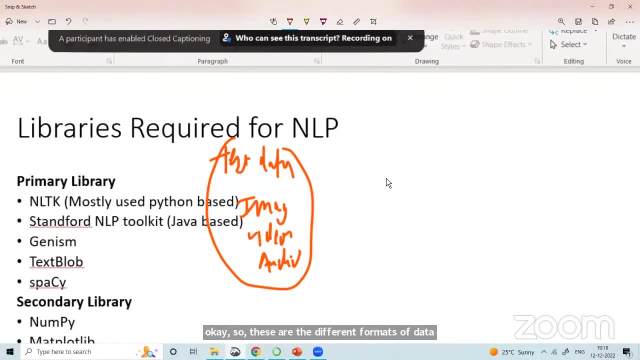 Okay, So these are the different formats of data, but when we want to perform or when we want to give this data to the machine, machine cannot understand this text data, image, video and audio. It can only understand all this data in the form of matrix or a vector in number format. 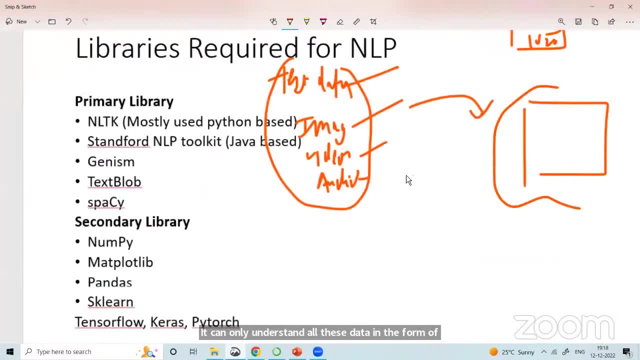 basically Okay. So in order to do this pre-processing internally, we require this Nrmpath library. Then matplotlib library is for the data visualization. Apart from that, you can take the use of CBON also, Then pandas library. it is for data manipulations. 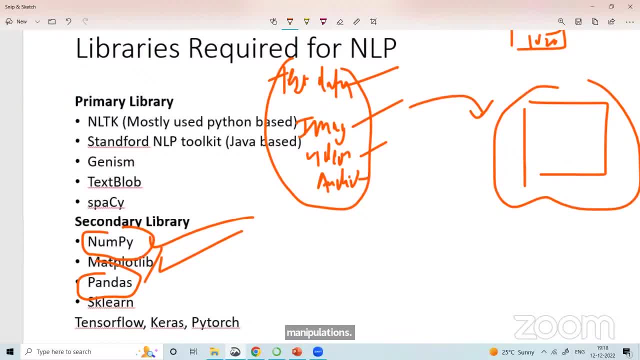 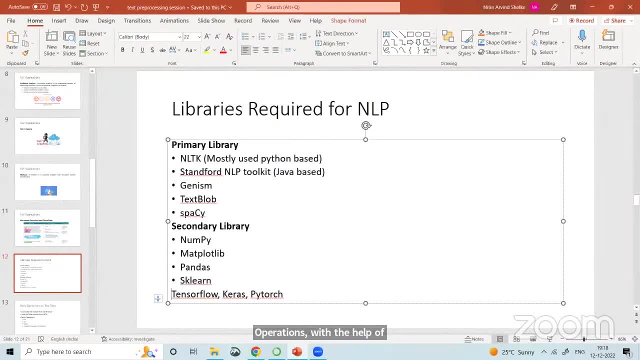 You can apply, you can read the files and perform several operations with the help of pandas library. Other than that, we require sklearn. So under sklearn we have several machine learning, the models, like classification, whether you want to go with the classification or the string on the text data. 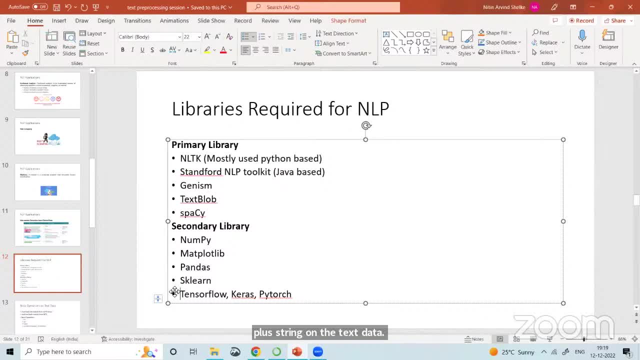 Okay, So you get random forest classifier or the decision tree neobias, all these algorithms are. these classes are present in the sklearn library and the tensorflow keras pytorch for the deep learning purpose. Okay, So you can apply the recurrent neural network, RNN, LSTM by LSTM, okay, GRU by GRU or the. 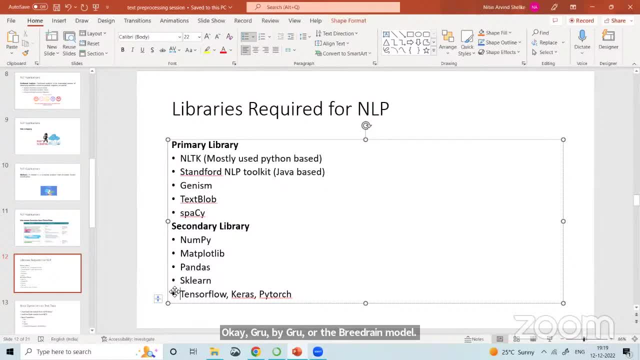 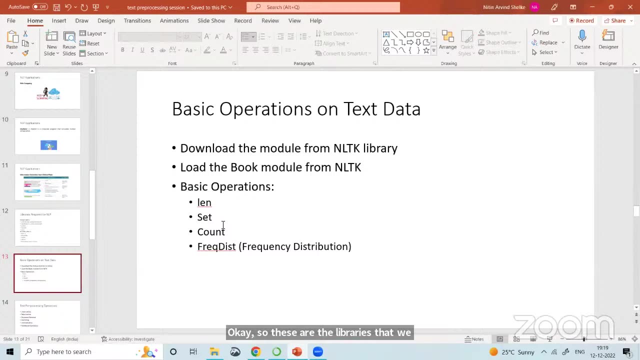 pre-trained model. then your embeddings transformer: Okay, So for that purpose we require these things: tensorflow, keras and pytorch. Okay So, these are the libraries that we require. Now. let's start with the hands-on part. now. 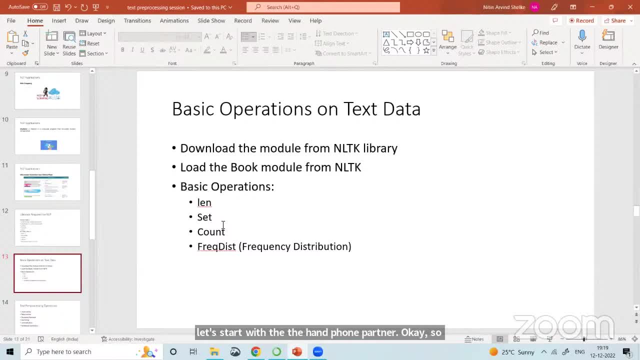 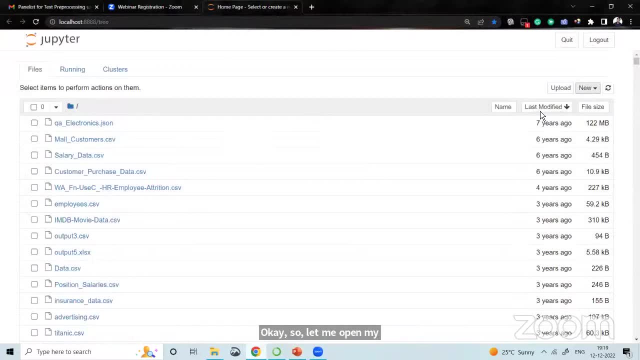 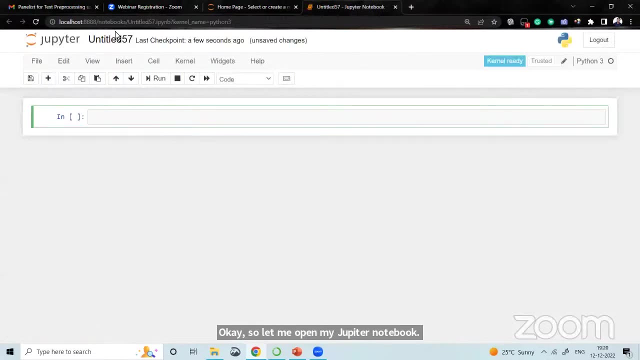 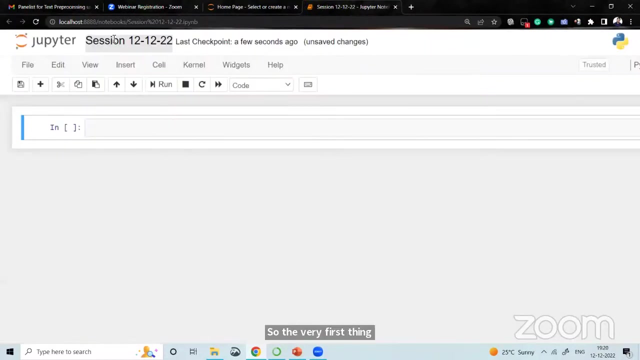 Okay, So we'll start with the very basic operations And then after that we'll go for the some complex operations. Okay, So let me open my Jupyter notebook. So the very first thing, the very first thing that we require it is analytical library. 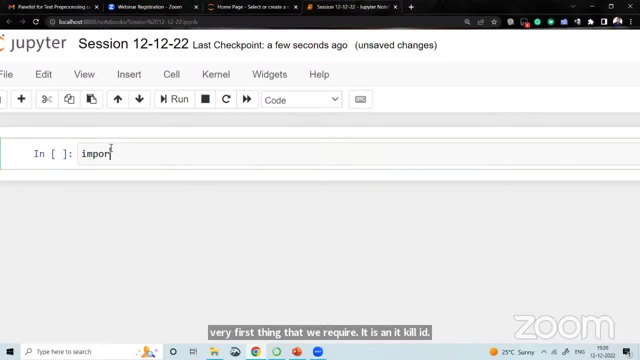 So, in order to use the analytical library, you need to write this line of code. Okay, So when we write this code and I have executed, It will take some time. Okay, It is successfully executed. Okay, That means this analytical library is present in my anaconda module. 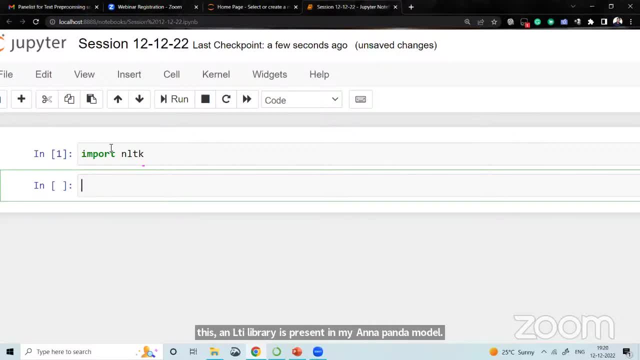 Okay, In anaconda Previously means last, uh, before the means back five years. okay, we need to install this nltk separately. but nowadays this nltk library is come up with the anaconda so you don't need to install it separately. so if you go with the anaconda, then you do not require to download or to install using pip. 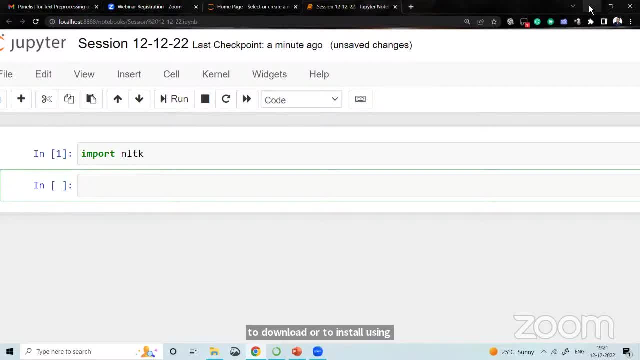 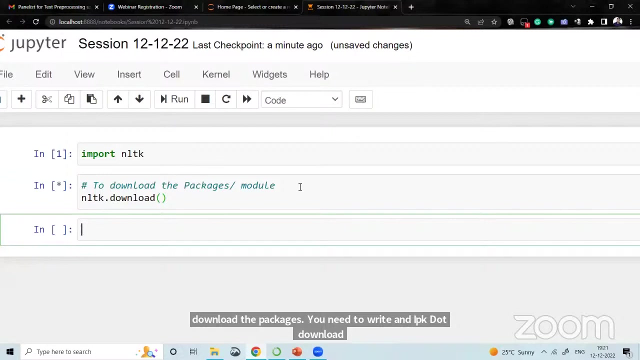 command. okay, automatically, you get it. okay. so this is how you can import the library now. after that, the next step is: you need some resources, okay, so you need some packages or modules. so to download this, to download the packages, you need to write nltkdownload. so with the help of this line, nltkdownload. 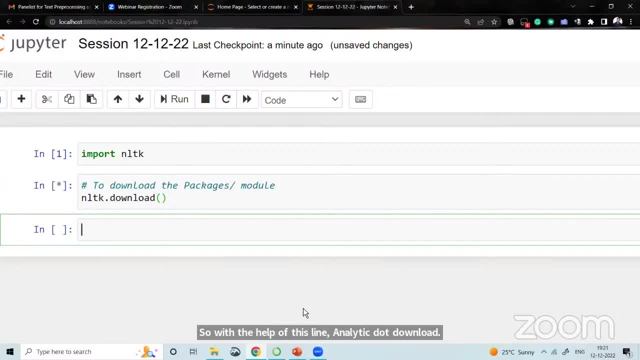 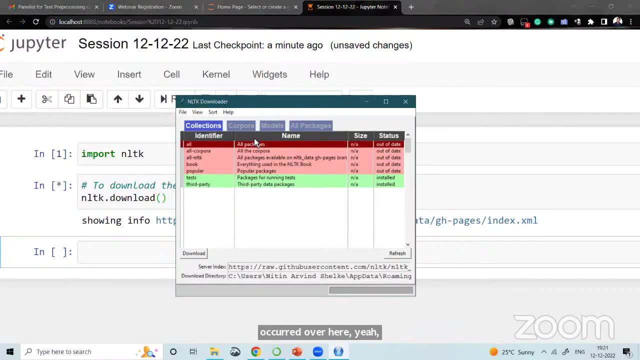 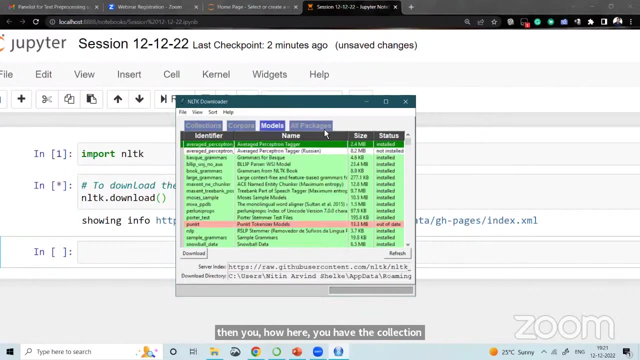 you get one screen automatically pop-up window data code over here. uh, yeah, this one, okay, so this is this, uh, the screen nltk downloader that you get and then you have here. you have the collections, corpus, models and all packages, so you just need to click on the download and all the packages. the book module. 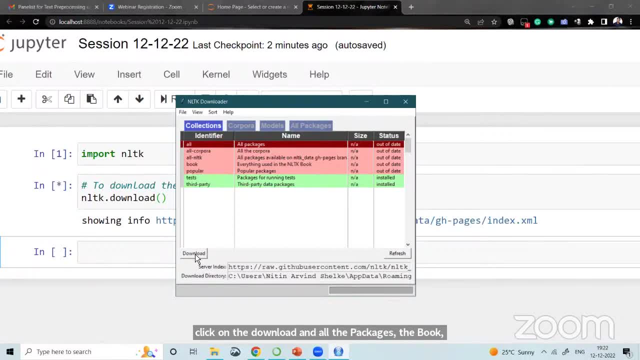 the different corpuses, like gutenberg web text- okay, there are a lot many corpuses that you can get, okay. other libraries, like stopwords, then your dictionaries, word net, everything you get it from here. okay, just in single click download. uh, you can download all the packages, which is which is to be required. 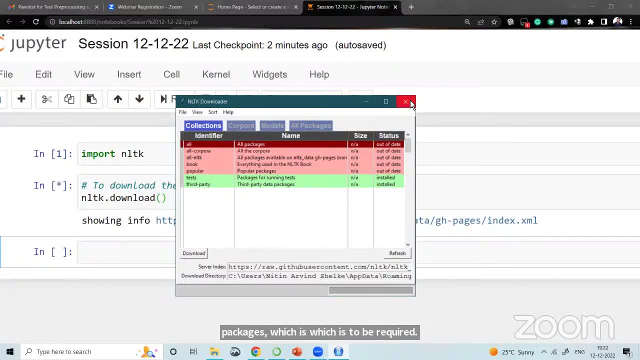 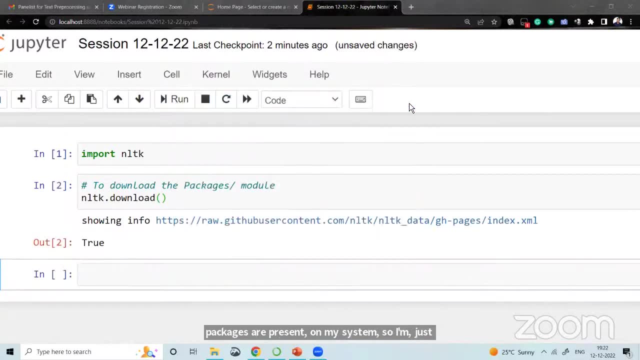 okay, uh, right now i'm closing this because, uh, all these packages are present on my system, so i'm just closing it, but you need to download all these things now. next next is: uh, let us start with the very basic operation, and for that you need some practice text. okay, so just the first module that you can load. 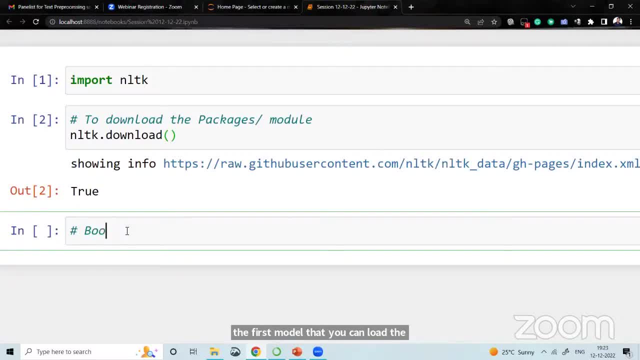 the book module. in the book module you get the several text file. in the book model you get the several text file, text one to text nine, on which you can apply some basic operations. okay, so just to download this book model. just give me second. okay, so the question is: how do i download this book model? 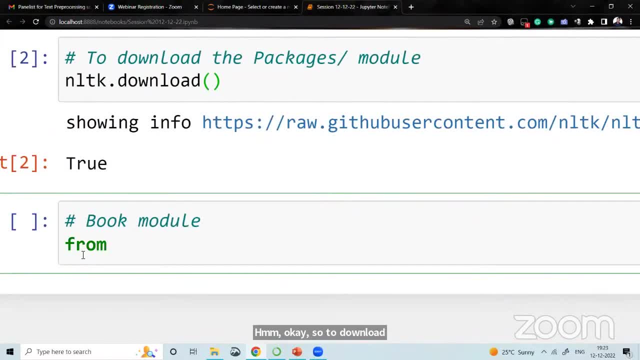 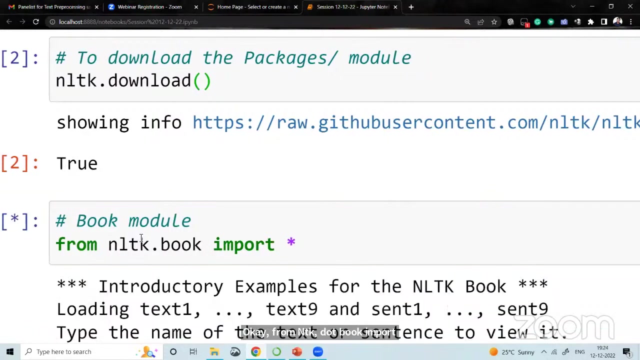 okay. so the question is, how do i download this book model? to download the book model so you can, okay. so to download the book model so you can right the from right, the from an ltk, you can. you can, okay, from nntkbook import star: okay. so with this line you can download all the text file. 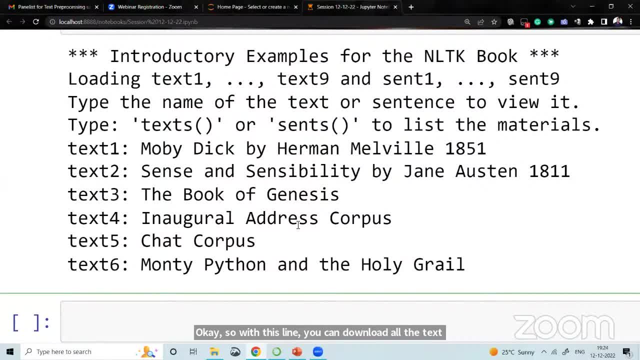 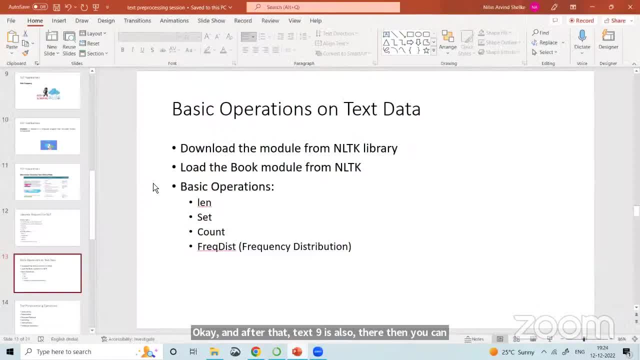 text 1, text 2 and text 3 and text 4. okay, and after that text 9 is also there. then you can go for the, the basic operation. okay, these all are the very basic operation. alien method: the. you get the length of the, the text, then set method to get the duplicate words from the text file. 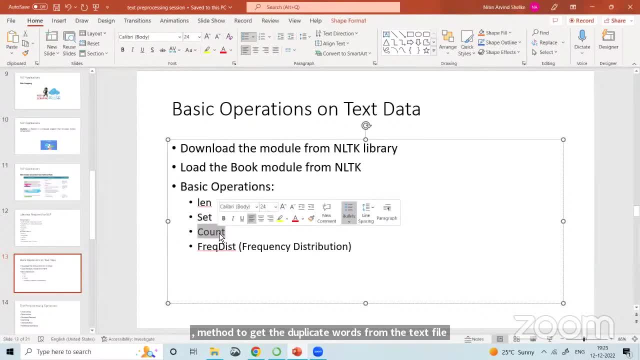 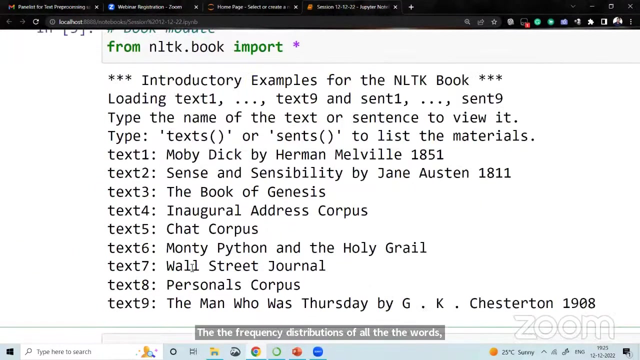 count method is used for getting the, the specific uh, specific uh word count and the frequency distribution. with the help of this distribution you get the, the frequency distributions of all the, the words. okay, so let us start with the alien method first. so i'm going to use the text one. so text one, i'm going to find the length of text one. it is. 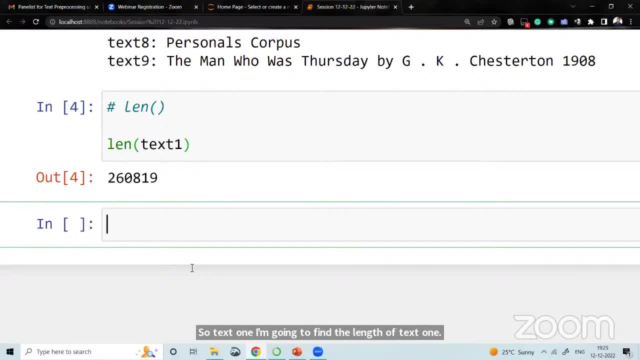 very basic method. so these many words are present in the text. one file. okay, then set that we have uh. through the set method you can eliminate the, the duplicate word. so if you want to find the, the length of the unique word, then you can write the length of set of text. one, okay. 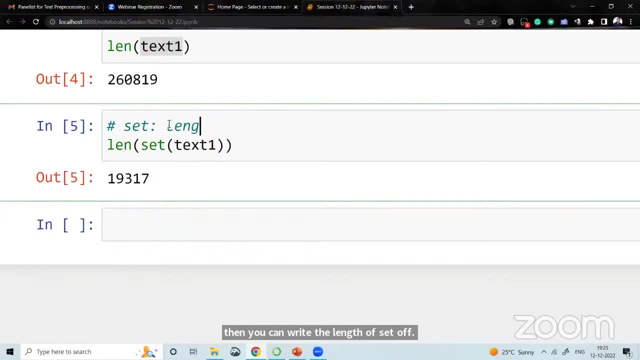 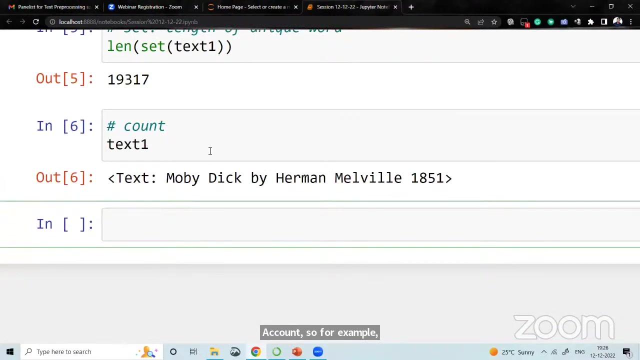 so with the help of this you get the length of unique word present in the text, one file. okay, then count method. with the help of count method you can count the length of the text, one file, the specific word count. so, for example: uh, let me write here text one, so under the text one. 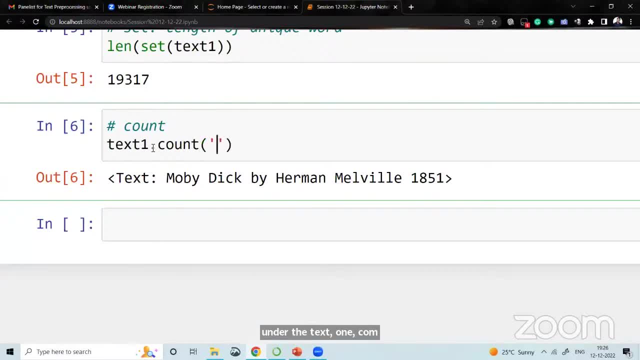 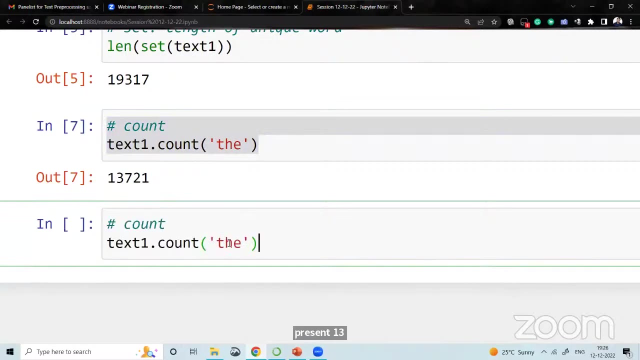 dot count and i'm typing the word. okay, i want to count the specific word, like, though i want to count the. how many times the word is present in the text. one file, so the is present: 13721. let me take another one, like while. okay, so the while word is present under the text one 216 time. okay, so this is very basic. 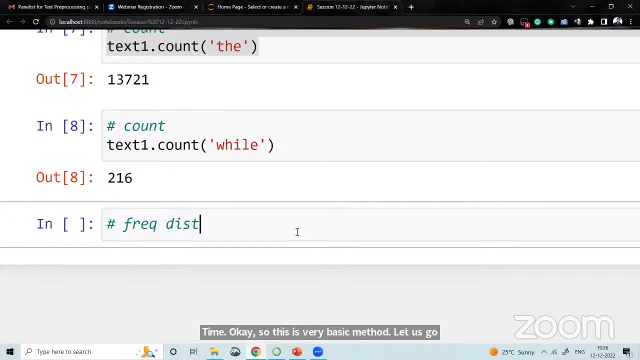 method. let us go for the frequency distribution now. now, this is important one, the frequency distribution now. if you, if you would like to get the frequency distribution for all the words, then you need to first import the, the frequency distribution class from the nltk library. so let me import this one. so from 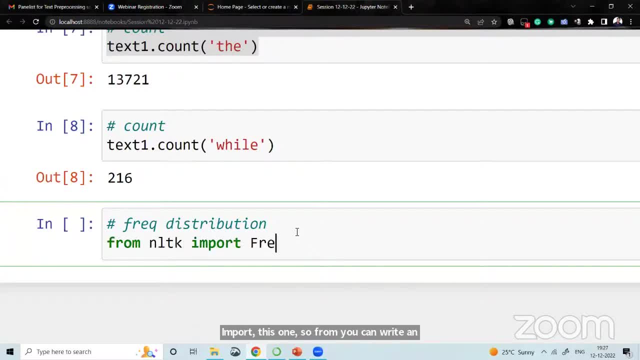 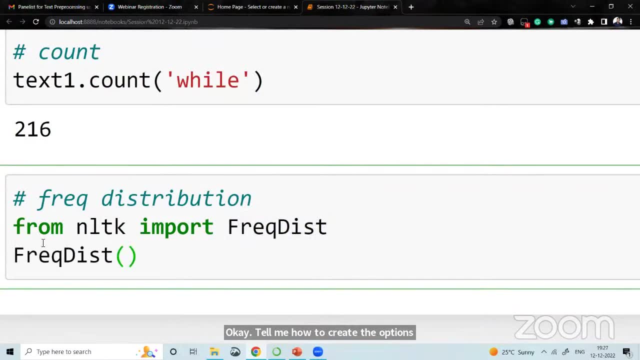 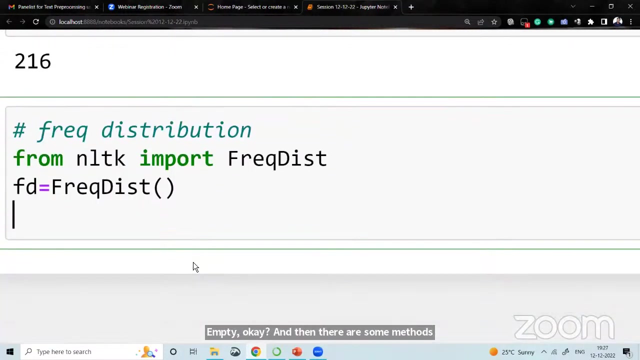 you can write nltk. you have to import the freekdist. okay, then you have to create the object of rick, this class. so this is my object of my 30 stars, md, md, okay. and then there are some methods. okay, there are mini methods, like if you would like to find the- uh, the most common words, okay then. 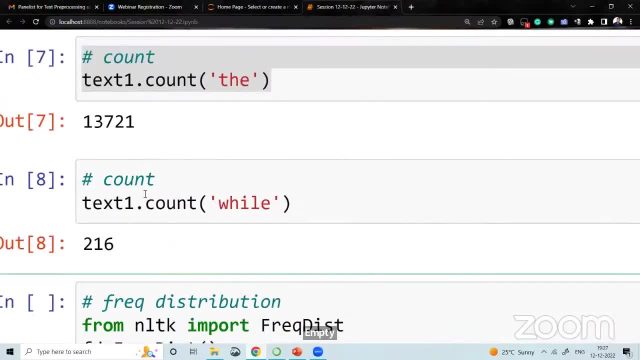 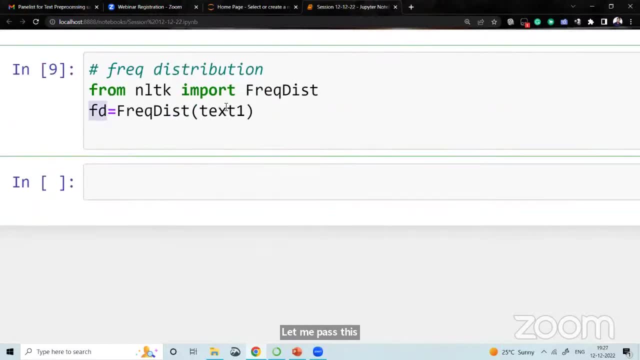 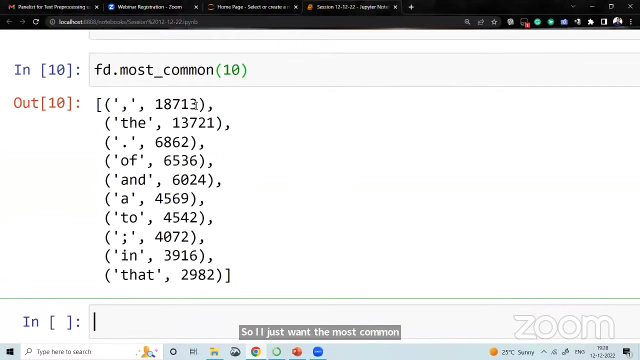 empty. let me pass this text one over here, okay, and then this is my object: empty. i have passed the text one now: fd dot. most common 50 words. so i i just want the most common 10 words. okay, so these are the 10 words, okay, comma. these many times the is present. these many times off is present. these: 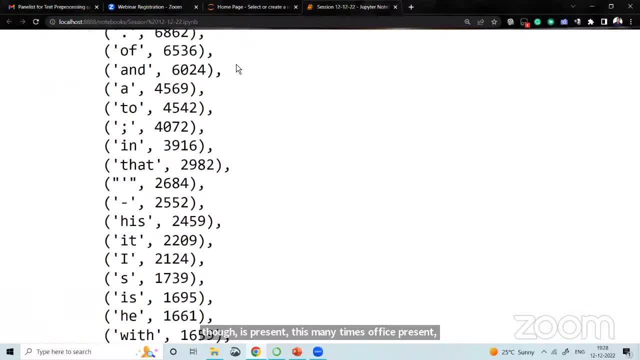 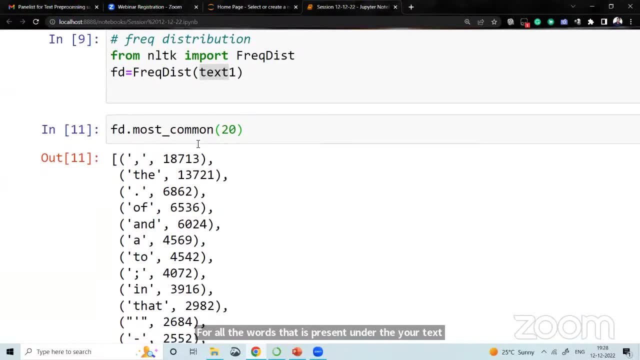 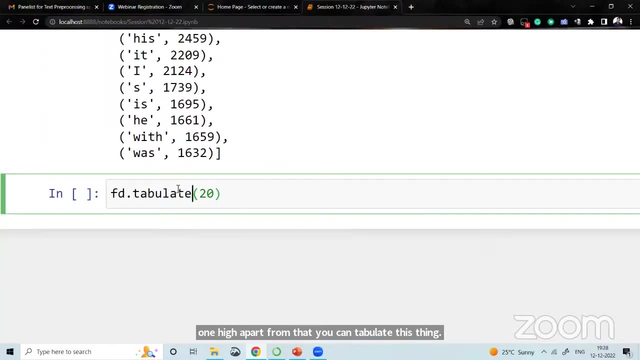 many times. okay, so you can pass any number. okay, you get the distribution for all the words that is present under the uh, your text, one part apart from that, you can tabulate this thing. okay, let me show you the tablet representation, tabular representation, with the help of this tabulate command, so you can tabulate. um, let me tabulate. 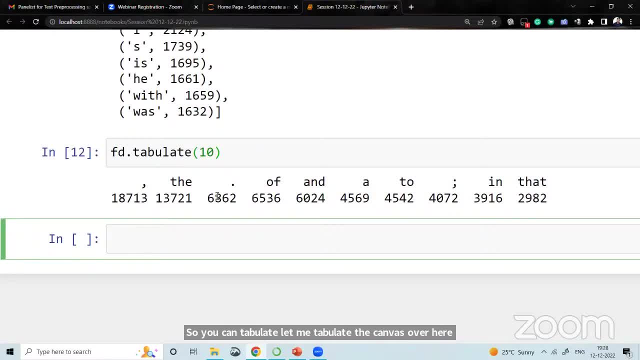 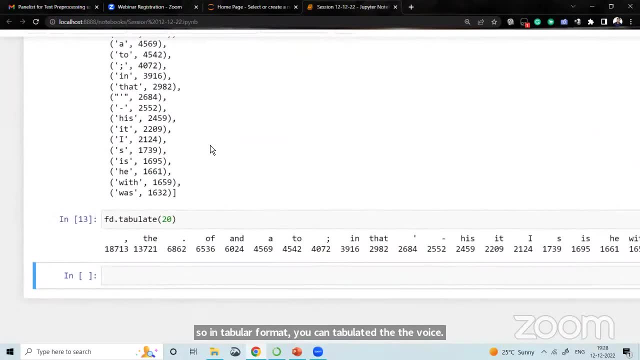 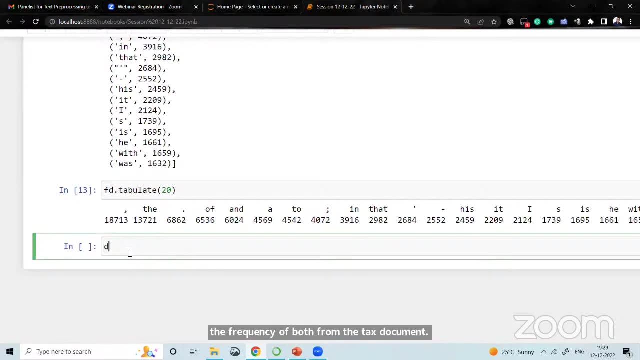 the 10 words over here. so in tabular format you can uh tabulate the the words. okay, 20 words, okay. so this is how you get to know the frequency of word from the text document. then you can also plot fd dot. you can get the frequency of particular word okay. so, for example, uh your fb and frequency. 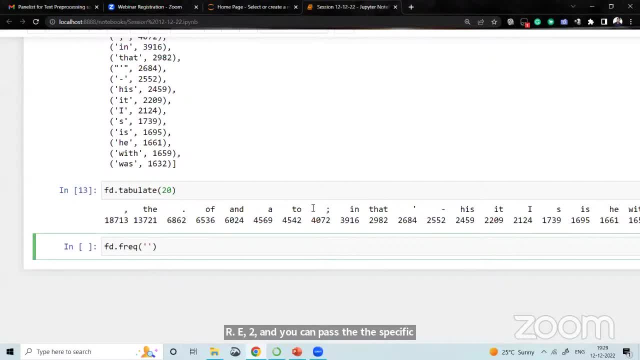 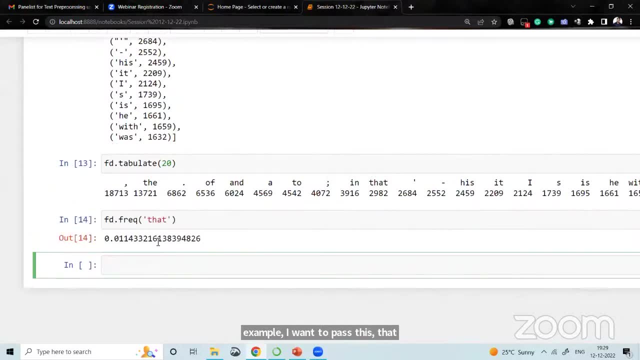 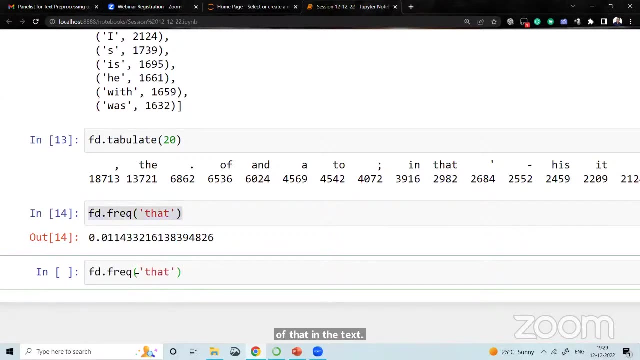 is the method, freq, and you can pass the, the specific word. so, for example, i want to pass this, that word. okay, the frequency. i would like to know the frequency of that in the text. one, this is the frequency- and directly pass this that you get the count. you'll get the count at the end. i'm going to share this. 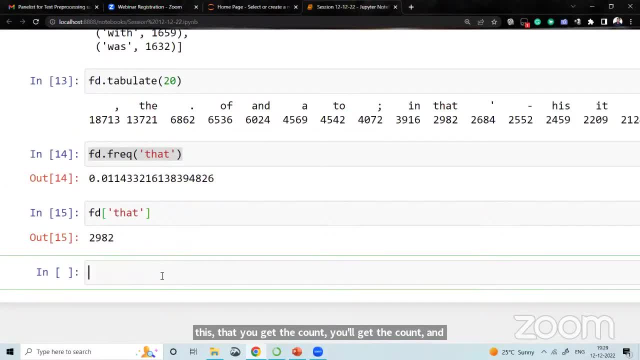 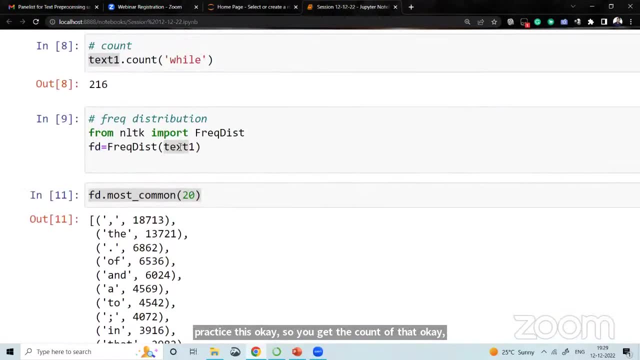 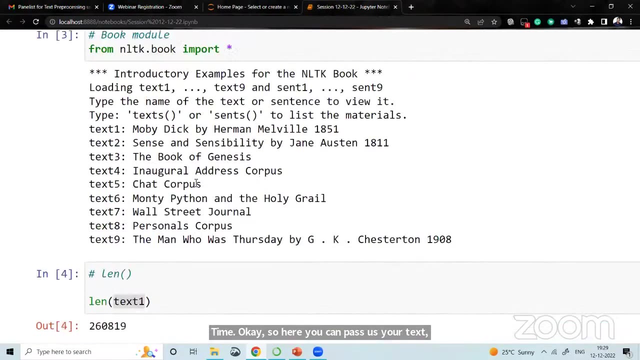 ip1 file with you to practice this. okay, so you get the count of that. okay, it's the specific count of that from the text. one file. okay, so here you can pass your text also. okay, uh, now this is what i implemented: all this method on the, the, the text file that is present under the book. 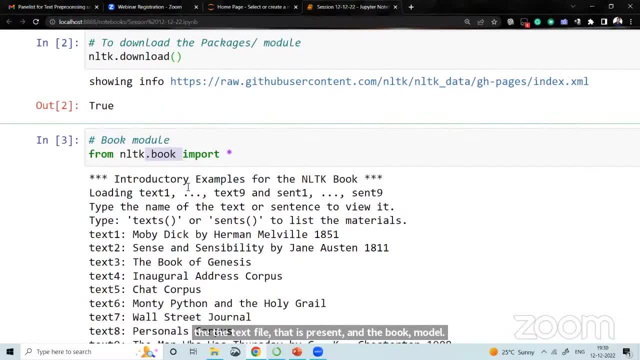 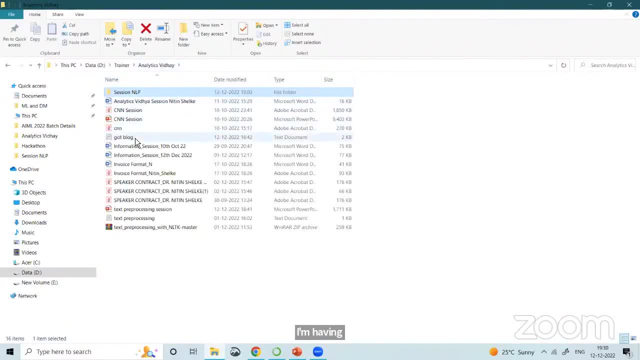 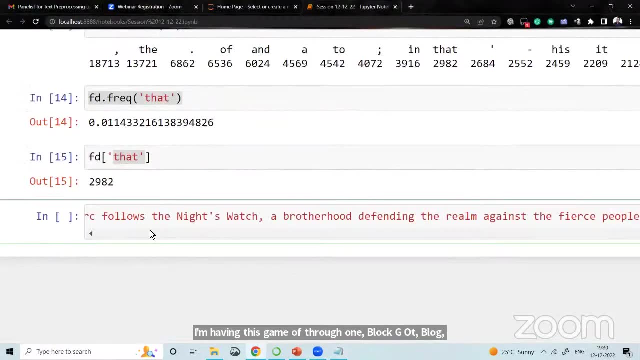 model, but you can apply all these things on your data also. for example, i am having this game of throne blog. got blog. okay, this is my input text and i would like to find the frequency distribution for this. okay, so this is my game of throne block, and. 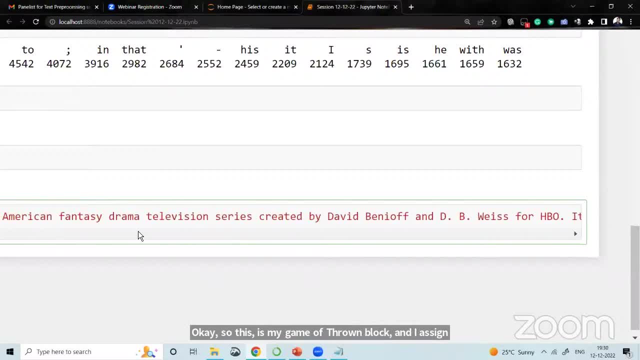 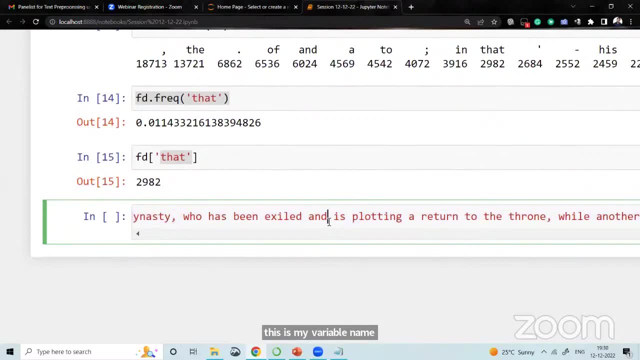 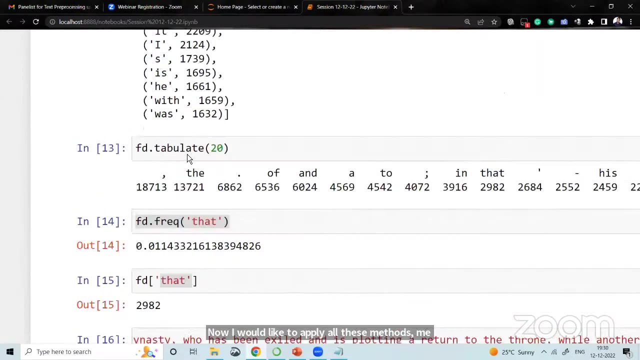 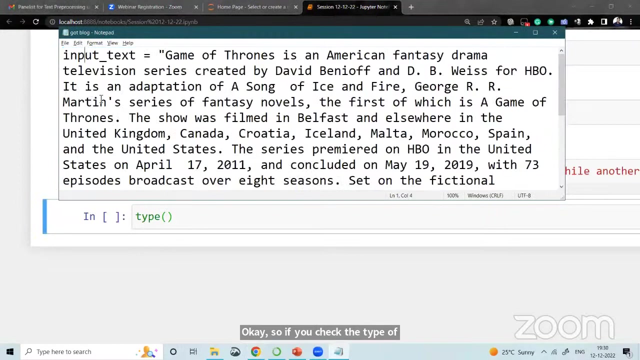 i assign all this text to my variable name input text. okay, this is my variable name input text there. i assign the the game of drones block. now i would like to apply all these methods, whichever we discussed. okay, so if you check the type of my uh this input text, it is string, but 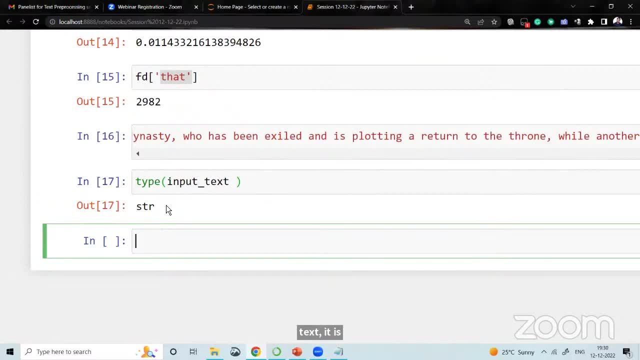 when we want to go for a string type of my variable name input text, it is string. but when we apply the, the frequency distributions and the method associated with the nltk, then you have to typecast the, the things you have to typecast- the, the input. okay, so you need to convert this string to the nltk dot text data. 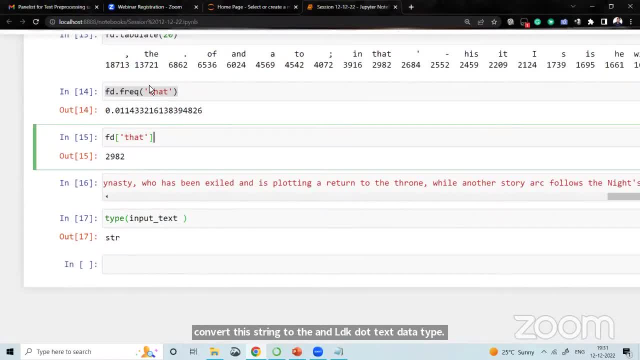 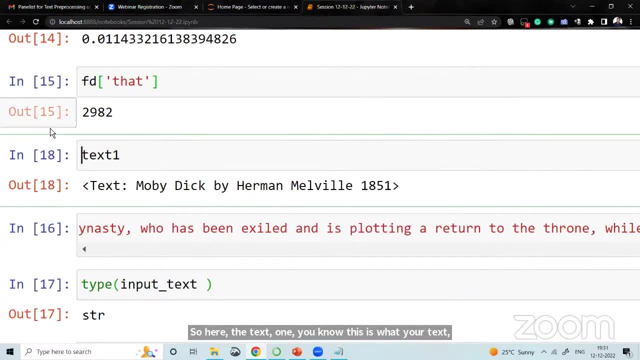 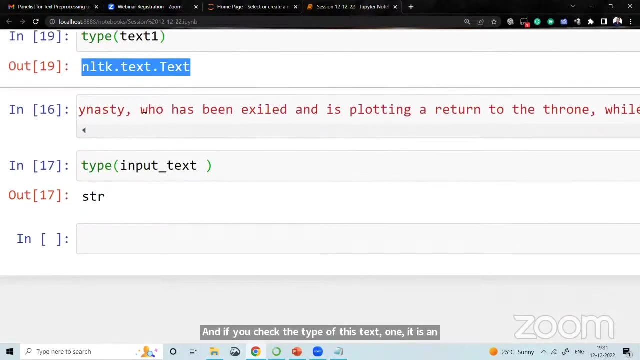 type. let me show you what exactly is what i'm seeing. so here the text one. you know this is for your text, one which is present under the book model, and if you check the type of the text one, it is nltk dot text, dot text. okay, and we also need to convert the string to this: nltk dot. 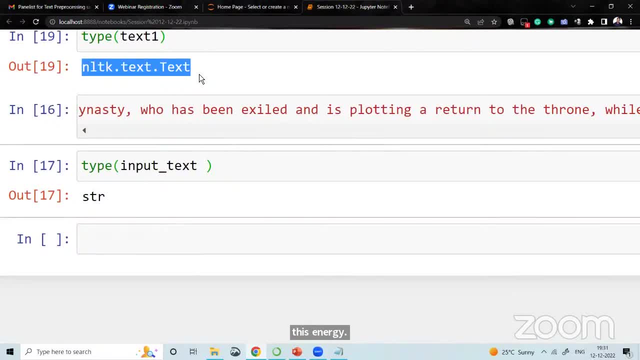 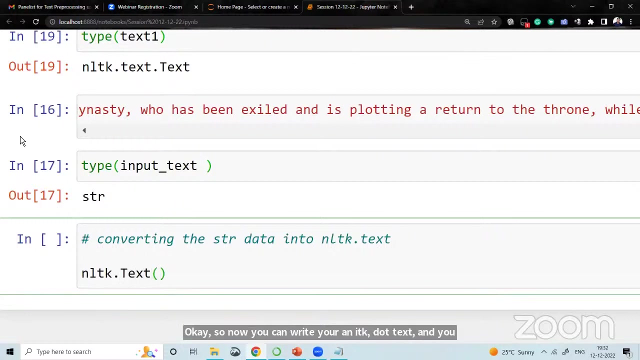 text, then only you can apply the methods, whichever we discussed earlier. so in order to typecast this, one line of code is required, converting the string data into the nltk dot text. let me copy this. okay, so now you can write here nltk dot text and you can pass your input text. 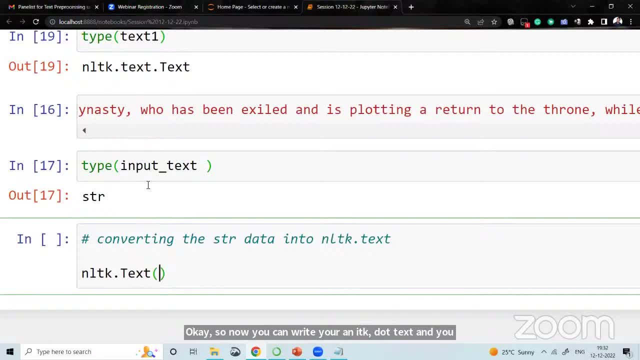 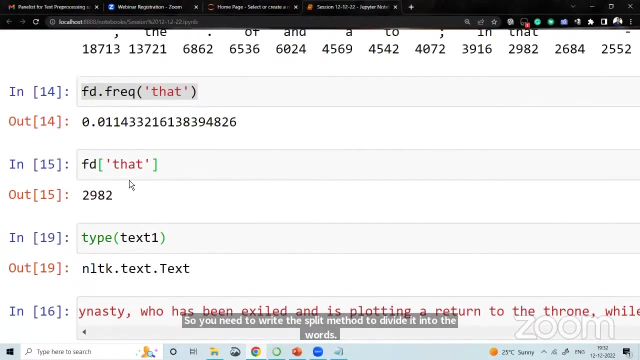 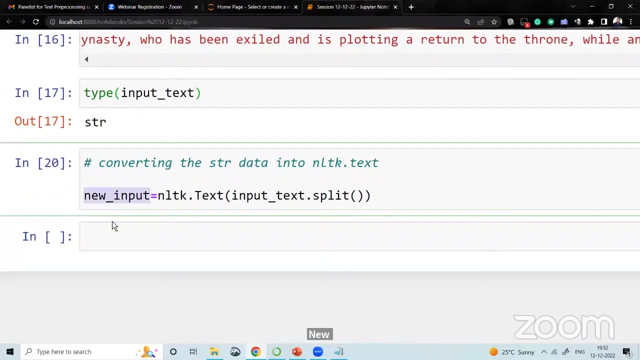 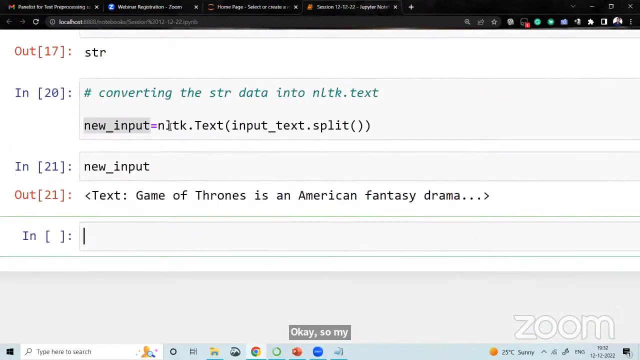 okay, so input text be also. you need to divide it into the, the tokens also. okay, so you need to write the split method to divide it into the words. and this is my new input, new input. okay, now let me show you my new input. okay, so my new input is now converted into the nltktext format. okay, nltktext format now you. 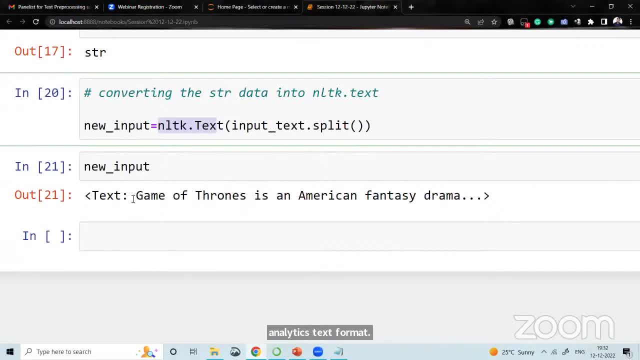 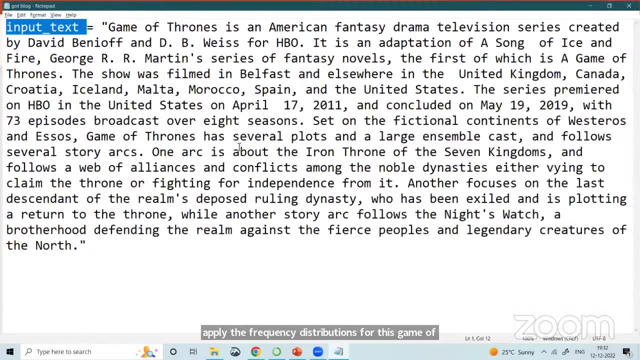 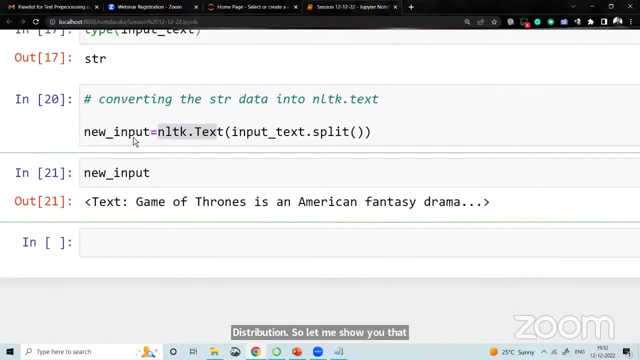 can apply the frequency distributions for this game of thrones blog. okay, this is our game of thrones blog on which we are going to apply the frequency distribution, so let me just show you me, show you that thing. so the same thing. already we have created this, so i'm just copying it and 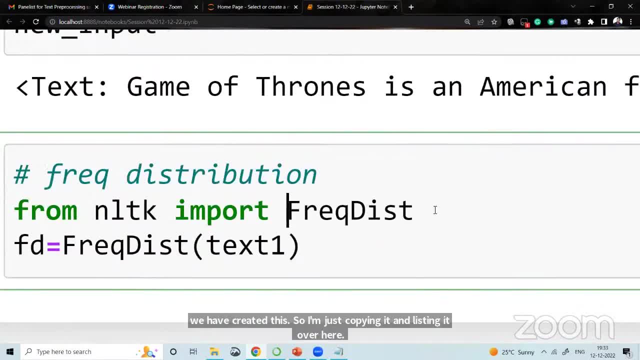 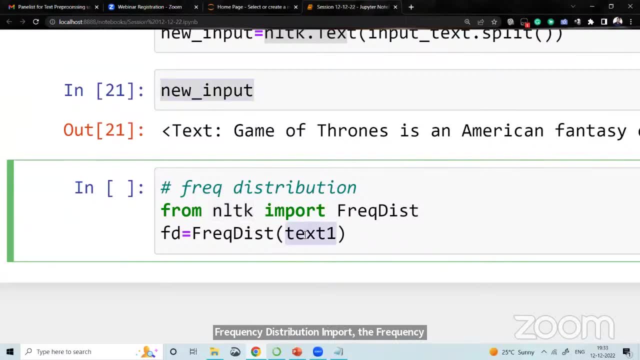 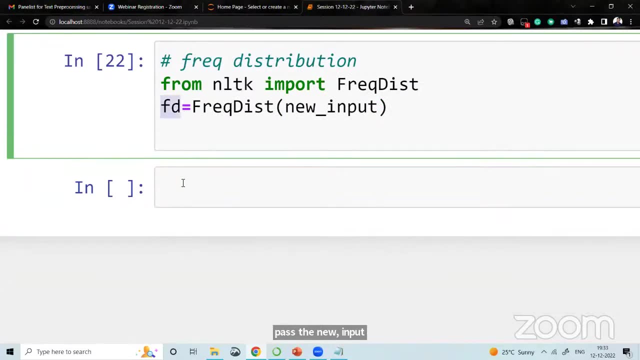 pasting it over here. frequency distribution. first you have to download the frequency distribution, import the frequency distribution from nltk, then create the object. now you have to pass instead of this text one, you have to pass the new input. okay, then you can use the most common word, most common. 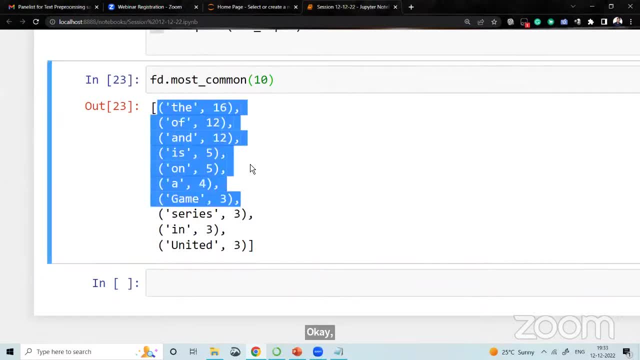 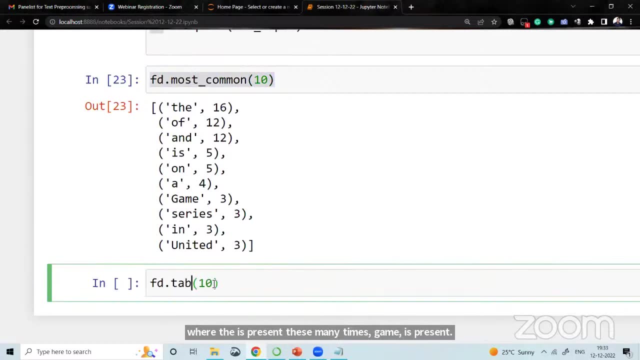 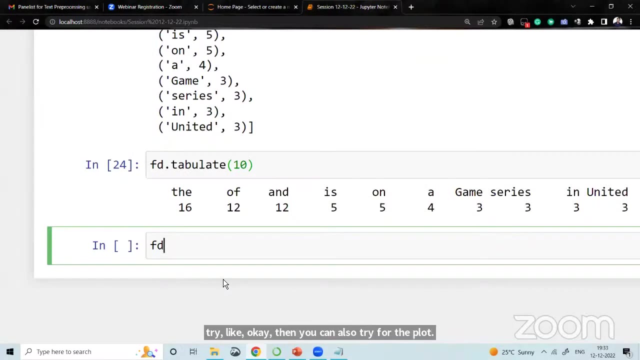 okay, 10 words from the block. okay, this is our block, where the is present these many times, game is present these many times. okay, so remaining all method. you can try the tabulate. okay, then you can also try for the plot, also. okay, there is one more method that is called as. 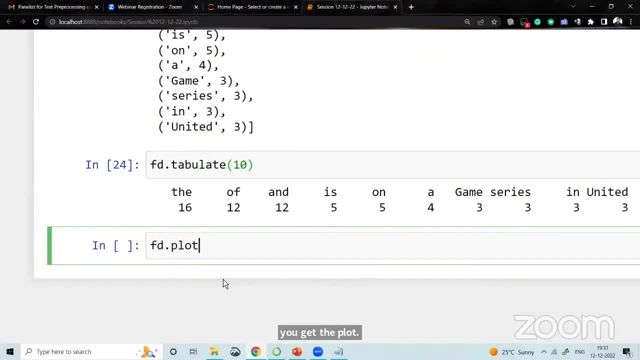 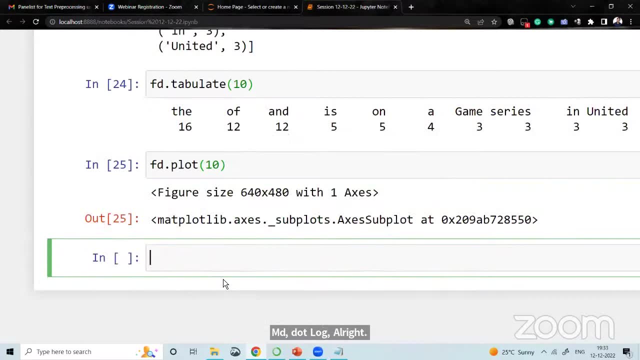 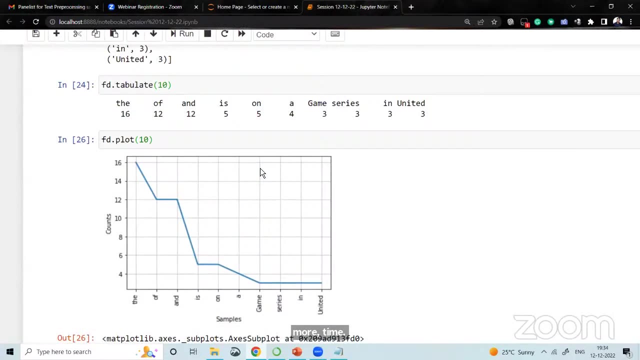 you get the plot, empty dot plot and the 10 words for 10 words. okay, so let me execute one more time. yeah, this is what the plot that you get. okay, so plot is one another method that you can use for under the frequency distribution. frequency distribution is a class. 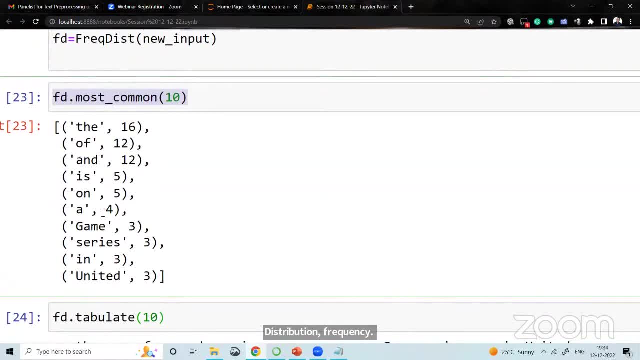 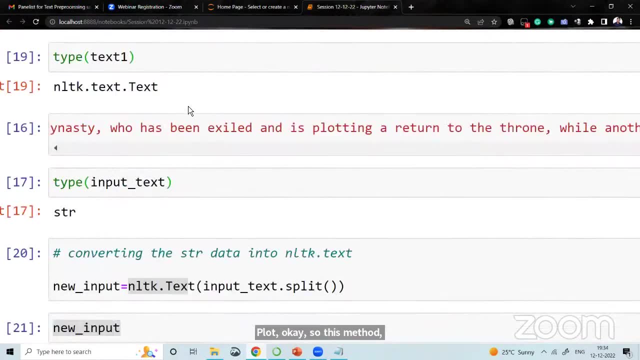 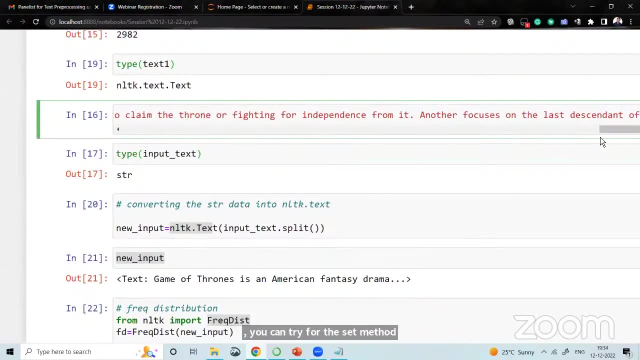 okay, this is your class. under that we have several method, most common tabulate plot. okay, so this method we have already discussed, which we have applied on the this input text. similarly, you can try for the set method, then length method on this game of thrones blog. okay, so these all are the basic operations that you can. 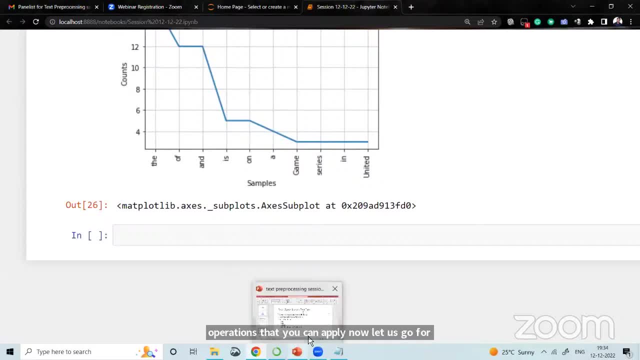 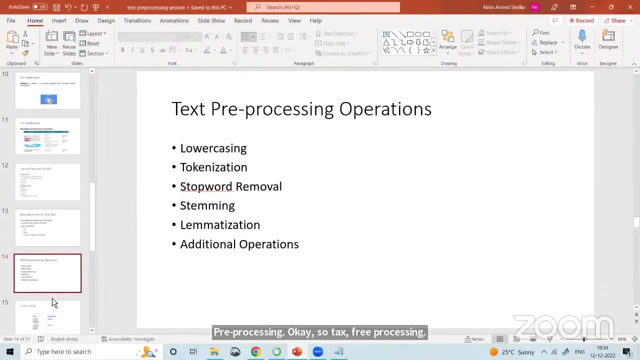 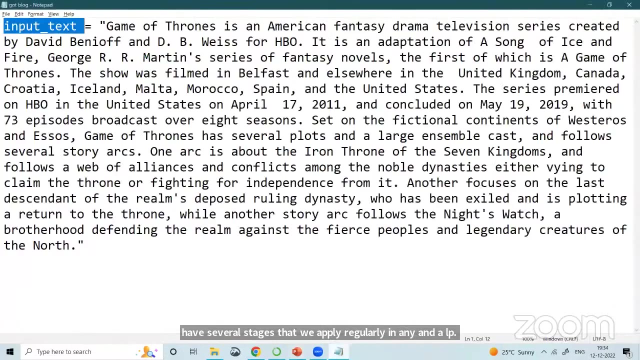 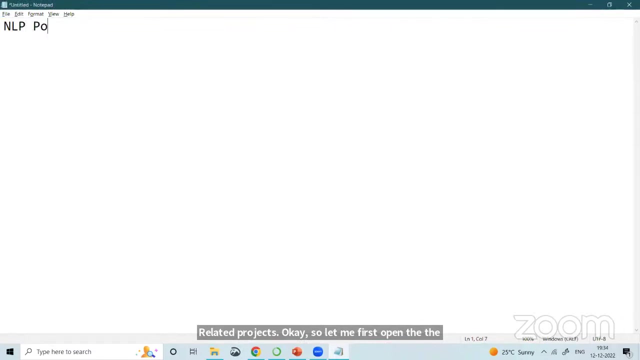 apply. now let us go for the: the text pre-processing. okay so, text pre-processing. we have several stages that we apply regularly in any nlp related projects. okay so let me first open the: the life cycle, nlp life cycle, nlp project, life cycle, life cycle: okay so, generalized life cycle. that we have the first stage is the problem. 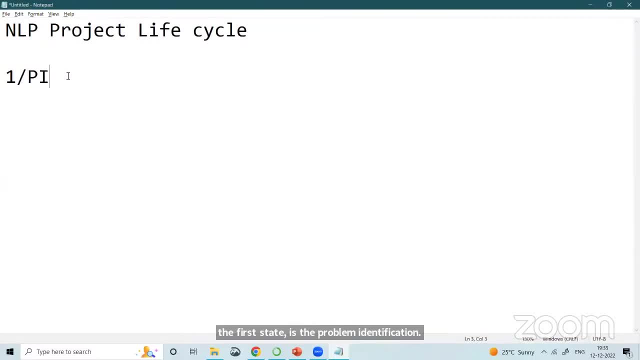 identification. okay, it is same under the deep learning also, machine learning projects also ai projects also, even for image pre-processing. image processing also the problem. identification is the first phase where we identify the problem. your problem may be a text classification problem. your problem may be a sentiment analysis. your 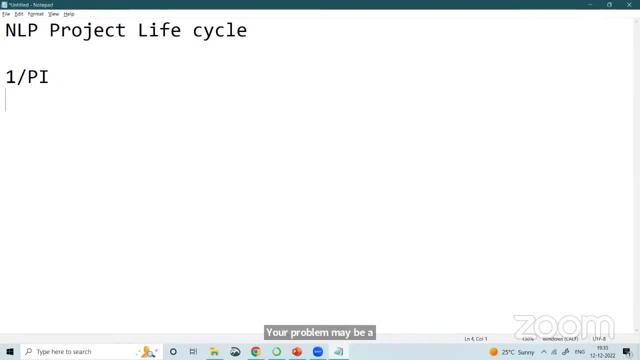 problem may be a text summarization, whichever you want and on what data set you want. so this is our problem: identification phase. then second phase that we go for, that is the data collection based on, based on your identified problem. say, suppose you identify that you want to go for the sentiment analysis on the the news: okay. on the political news: okay. 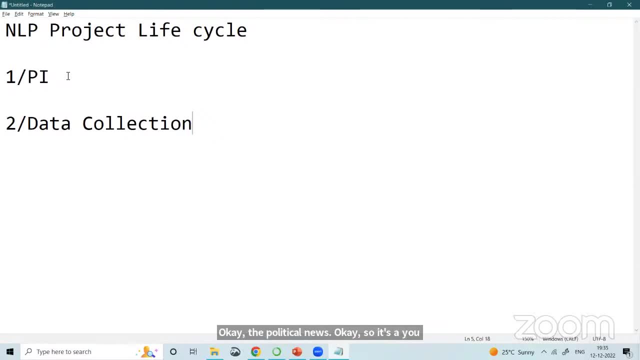 say, suppose you want to go for sentiment analysis on the political news, so you need a data. okay, you need, you need to collect the data that is related with the political news, which you can collect it from the different websites. okay, like from kaggle, from uciml and google. data set search. 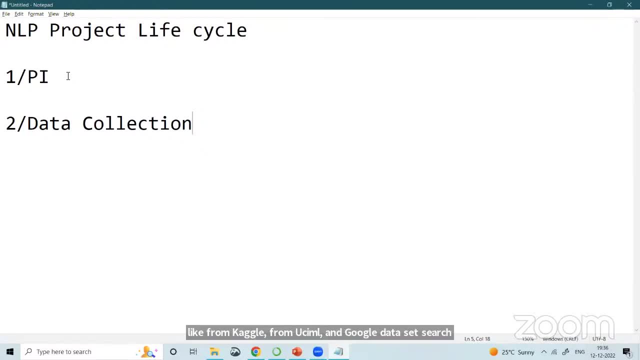 engine. there you can download the text data. okay, for your project purpose. okay, data collection is the second stage. then, under the third stage, we have text data pre-processing. as we are talking about text data today, we are talking about the text data, so that's why it is not a normal data. 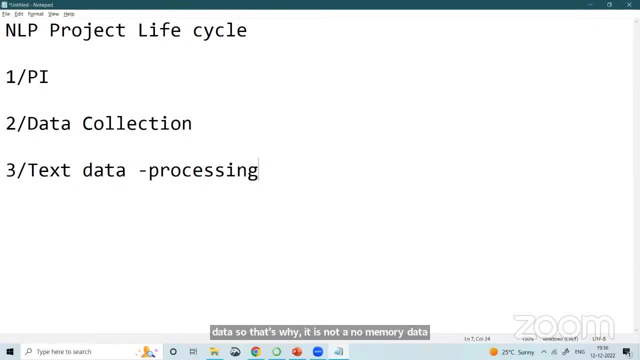 pre-processing. it is a text data. let me write here text data pre-processing. okay. so third stage is the pre-processing. so whenever we go for collecting the data from the real world, that data is having some issue. okay, that data is not a design, that data is not in the desirable format, that is to 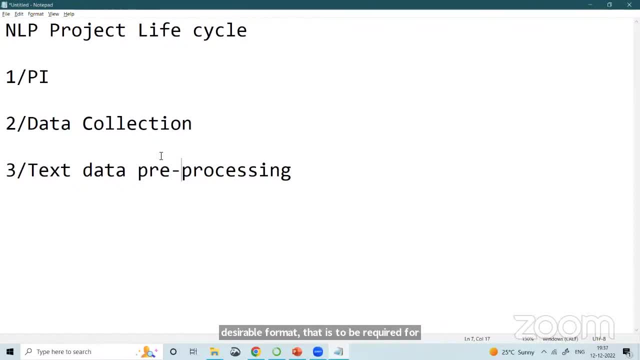 be required for further analysis. further analysis means what we want to create: the sentiment analysis, a model with the help of deep learning or with the help of word transformer. okay so you, you have to convert the raw data into the useful form. so under the text data pre-processing, we have several stages. okay so. 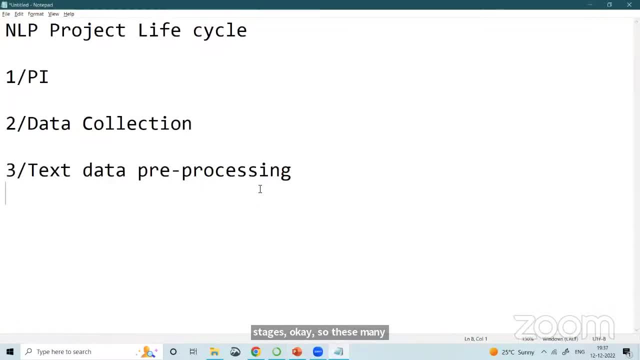 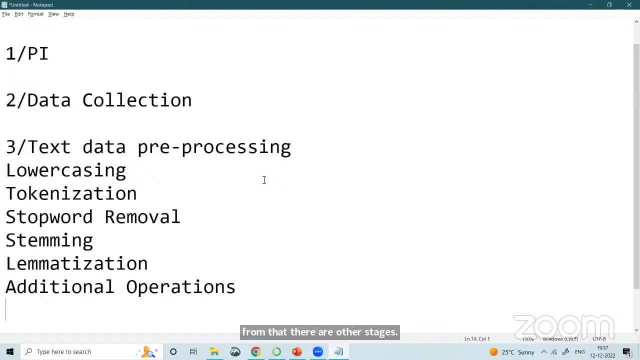 these many stages we have under the text pre-processing. apart from that, there are other stages also. other stages means, uh, removing the unnecessary columns, removing the duplications, and then, uh, splitting the data, scaling the data, okay, apart from that, there are certain other things also, but these are the most common stages that include under the text, data pre-processing. so 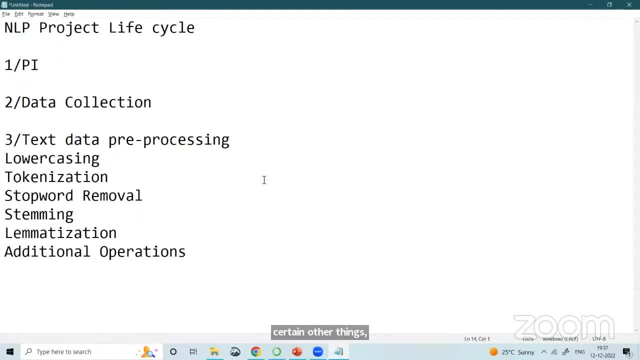 text data pre-processing. so whenever we say, uh, the NLP project life cycle, your 50 percent of work is going under the the pre-processing part, then once we get the useful data- means the conversion of raw data to the useful form- then we go for the model creation. model creation before that. 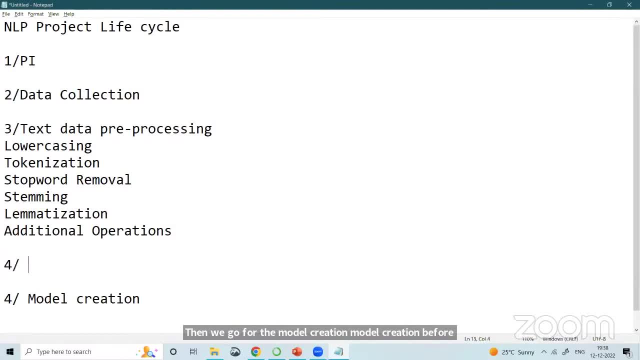 we have feature extraction also. let me write feature extraction. so under the feature extraction part, uh, we need to convert this text into the vectors or the array. so for that purpose you can go for the, the different embeddings or some feature extraction technique like bag of words: pow, then tf, idf, okay, word to back, then there are other embedding these. 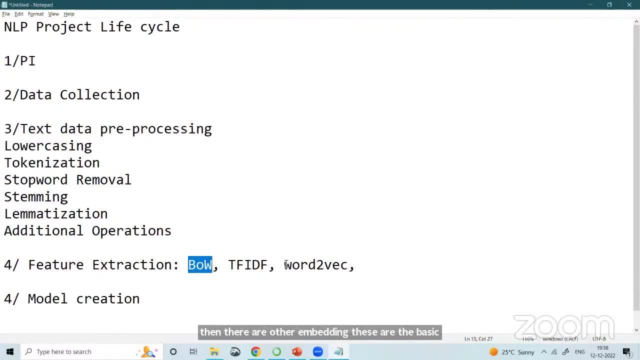 are the basic feature extraction technique for the text data bag of word, tf, idea word to bed and some advanced one like glow under the glow. also, you have several versions. okay, then pass text. okay, these are the the embeddings, word embeddings, and you can also go for the transformers also. 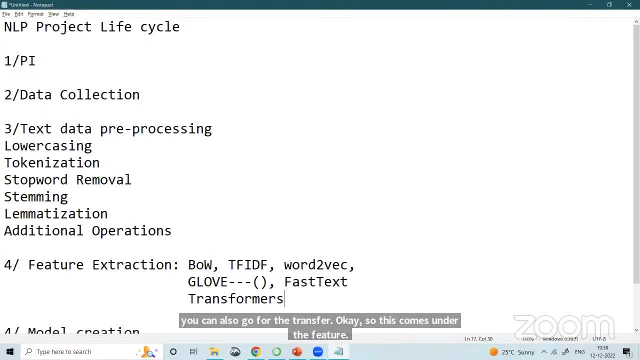 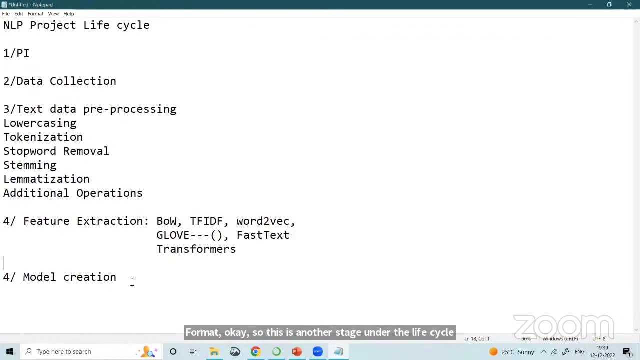 okay, so this comes under the feature extraction. that means the you can convert the text data into the vectors. okay, because machine cannot understand your text data as it is. word as it is, it creates the the vectors in Zero One format. okay, so this is, uh, another stage under the life cycle of NLP. okay, model creation, where you need to create the 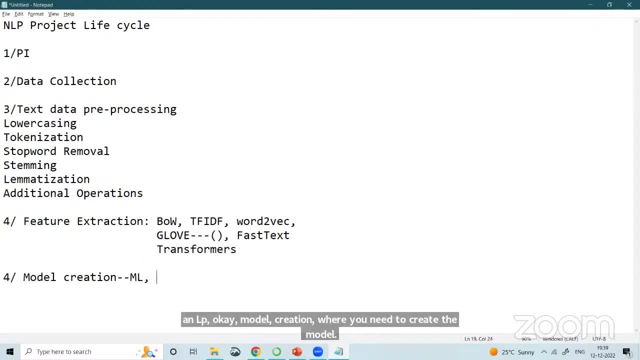 model. you can go for the basic model, machine learning model, or you can go for the DL model, can go for the part. okay, whatever you want. then next is model. i'm not going in detail of these things- model creation- because today's topic is text data pre-processing- but you should know. 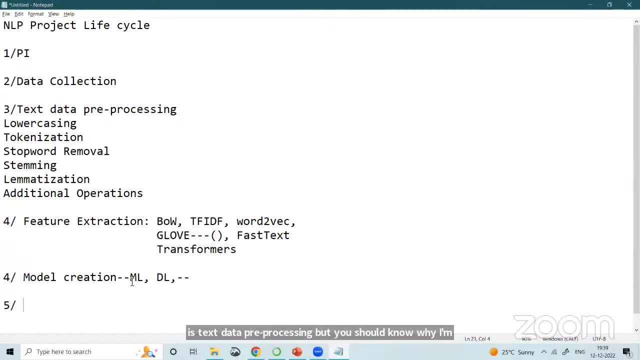 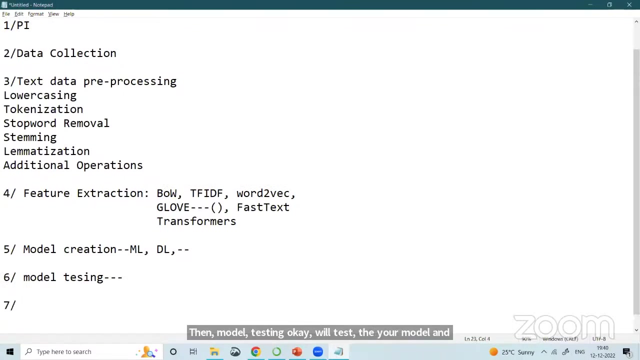 why i'm explaining this? because you should know why this third stage is important in order to proceed for the, the fourth, fifth and sixth stage. sixth, then model creation, then model testing. okay, we'll test the your model, and we evaluate the performance of the model. model testing, we test. 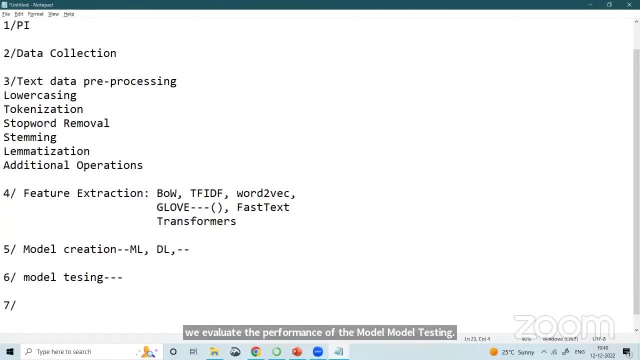 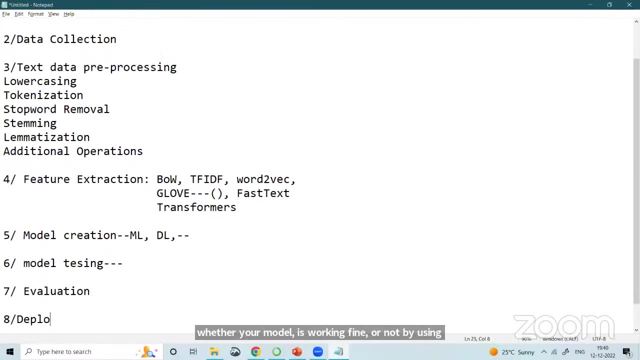 the model on the test data set, we create the model on train data set and evaluation. evaluation means you can evaluate the performance of your model- whether your model is working fine or not, by using the different performance metrics, and the last stage is the deployment. okay, so this is how the 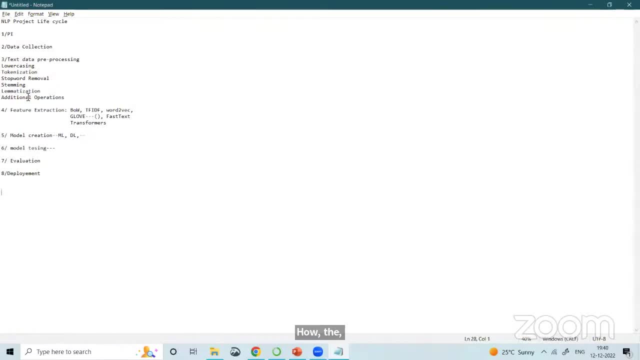 these. these are the stages that include the, the, the common stages under the nlp projects. okay, problem identification, data collection, text data pre-processing: there you require lower casing, tokenization, stop, word removal, streaming, lemmatization and additional operations. okay, and remaining all four: five, six, seven and eight. we are going to discuss this thing now. 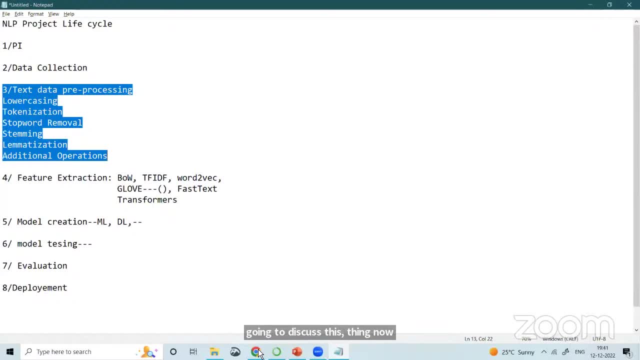 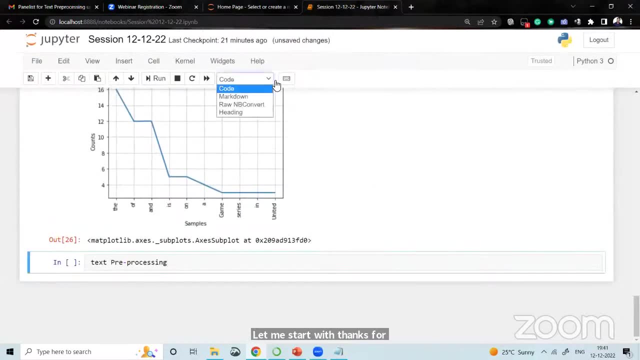 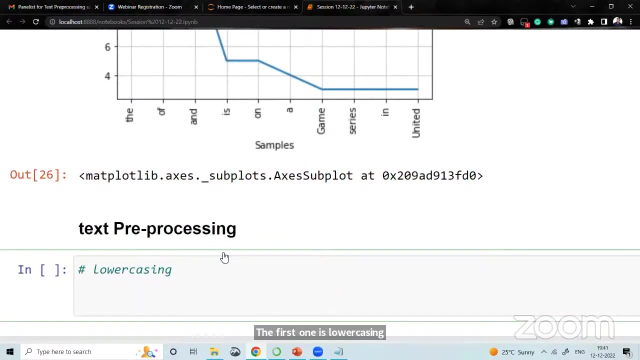 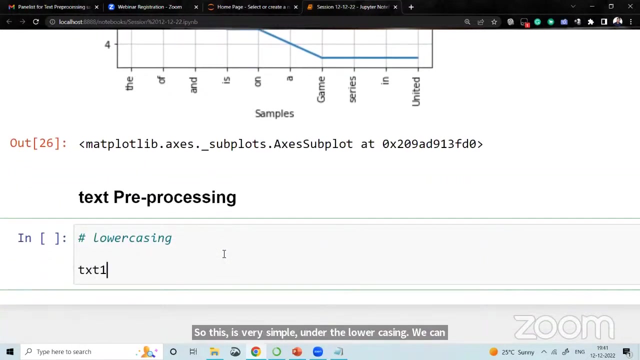 let me start with text pre-processing. we'll go for the. the first one is lower casing. so this is very simple. uh, under the lower casing, we can convert the, for example, i'm considering the txt one you all know. welcome to the world of nlp. okay, and if you would like to convert, why lower casing is important? because python is a. 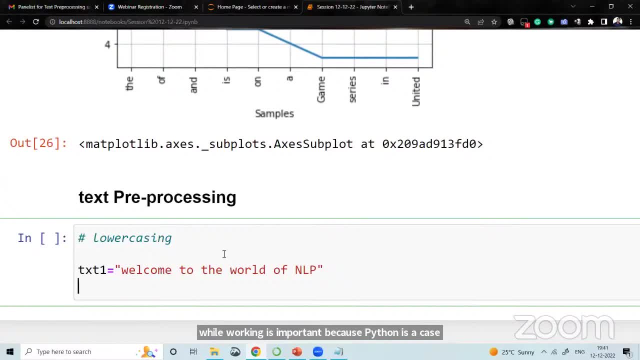 case sensitive language and capital w and small w is having a different meaning. okay, even in nlp also, the capital w and small w is having a different meaning. so in order to avoid the confusion, we go for the lower casing and it is very simple. this is with a very basic method, slower method with the help of this dot: lower key. wrong scaling method is beleza. 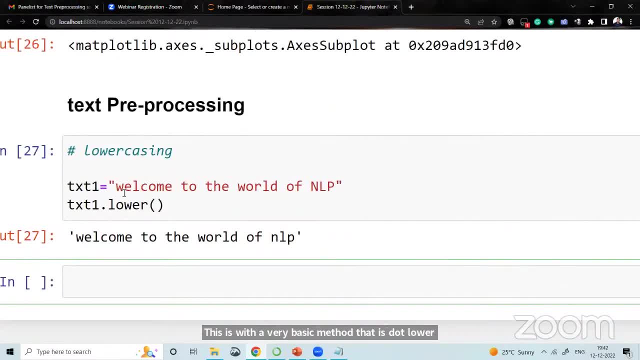 method is hello, lower method. we can convert all the text into the lowercase. you can see over here, with the help of this dot lower method, you can convert all the text into the lowercase. so whenever you want to go for the, the text pre-processing, the first stage is the. 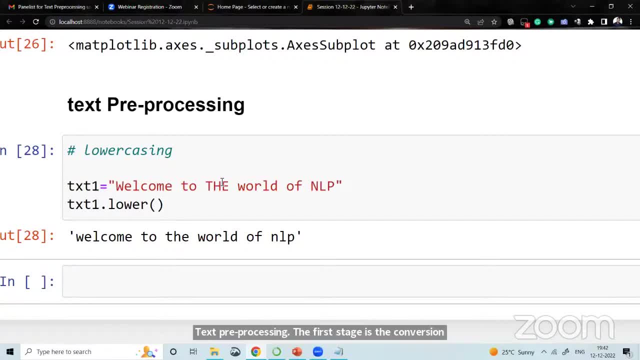 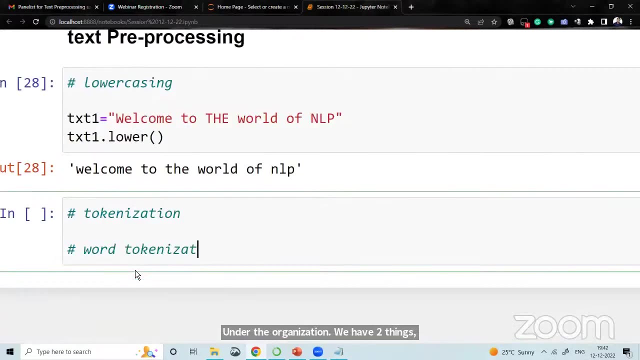 conversion of your text into the lowercase. okay, so that you can avoid the further confusion. next stage is tokenization. under the tokenization, we have two things. one is word tokenization, another is sentence tokenization. sentence tokenization- okay. so it is again based on your application, on which project you are. 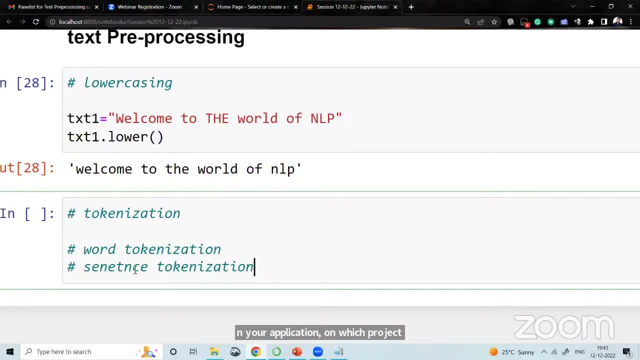 working- say, suppose you are working on the sentiment analysis- okay, then word is important for us. okay, That means the word tokenization is necessary. You need to divide the text paragraph into the words. If suppose you are working on some summarization, okay, and where the sentence is playing a very important role for you, 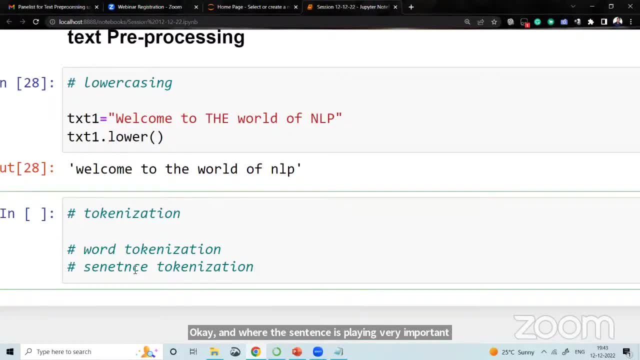 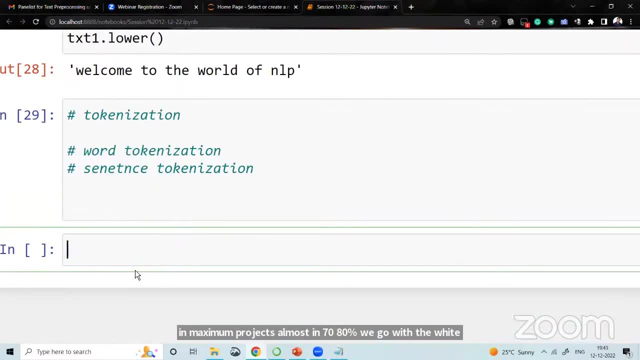 then go for the sentence tokenization. But in maximum projects, almost in 70-80%, we go with the word tokenization. Okay, let us go with the word tokenization. So right now I am just taking the input, normal input, okay. 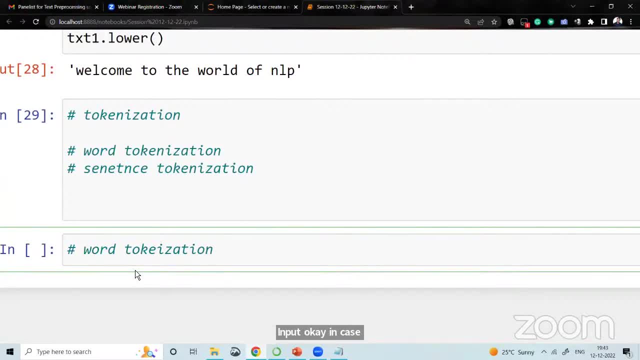 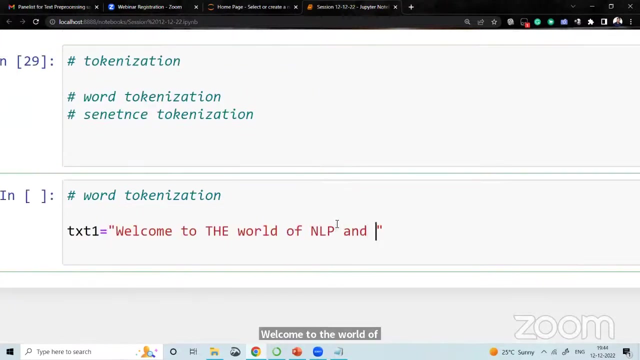 In case study. I will take the one text file, okay, import it and then apply all these steps. okay, So word tokenization, I will take the small sentence text one. Welcome to the world of NLP And hope you all are enjoying. 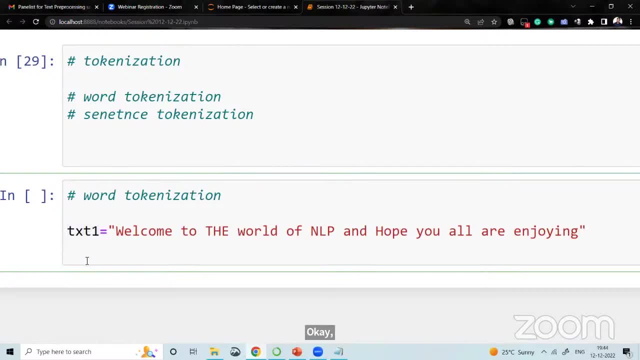 Okay, this is my text one. Now, in order to tokenize this using NLTK library, you have option that you can use the dot split method also, But we are going to discuss this thing with NLTK library, So from NLTKtokenize. 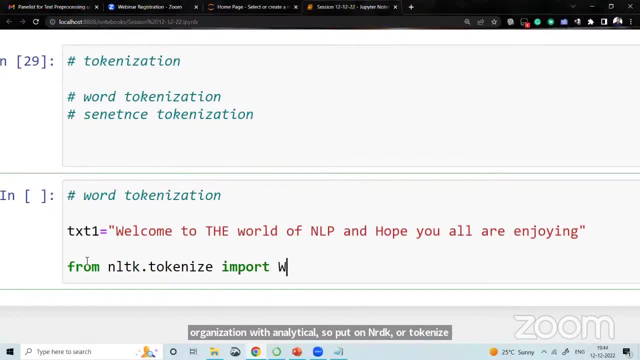 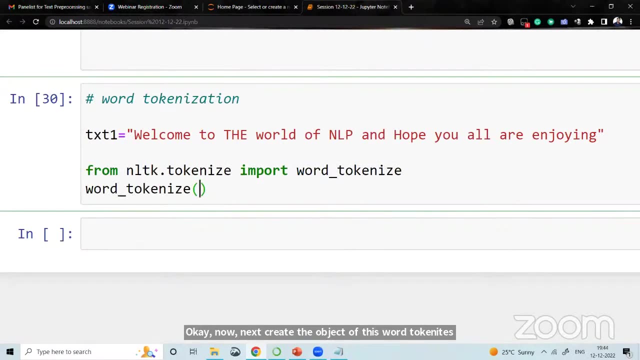 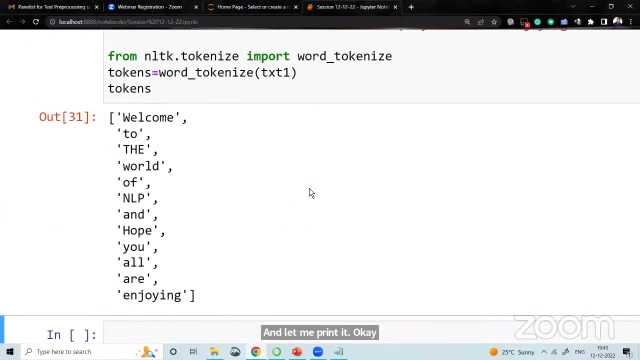 you can import word tokenize. This is class word underscore: tokenize. Okay, now next, create the object of this word tokenize, Pass your text- This is my text one- And you get the tokens And let me print it. Okay, so these all are my tokens. 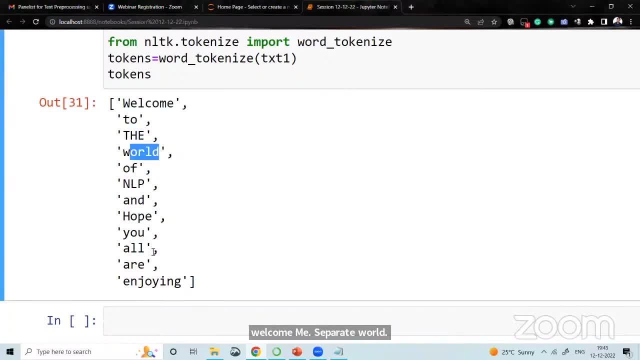 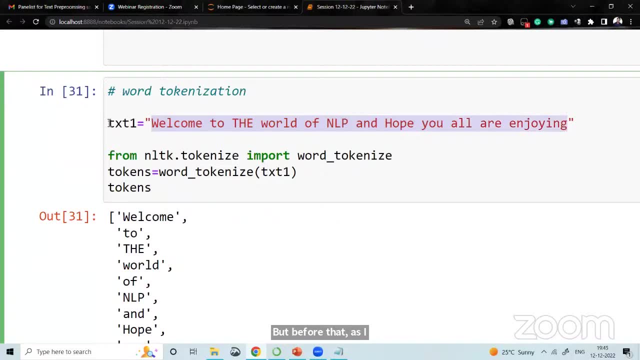 Welcome is separate word. two is separate. the is separate word is separate, all are separate. But before that, as I said, you need to convert into the lowercase also, The first step you have to convert it into the lowercase. 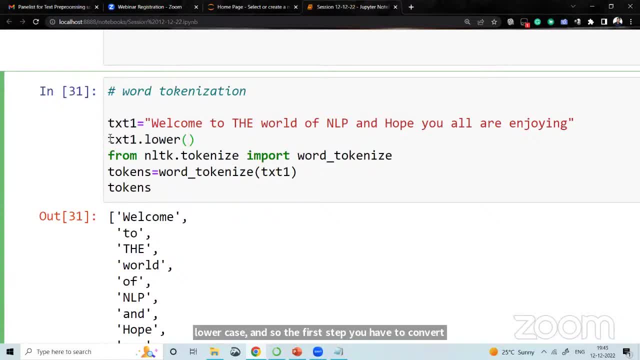 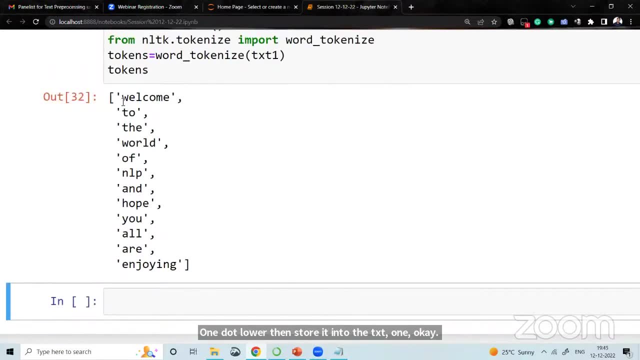 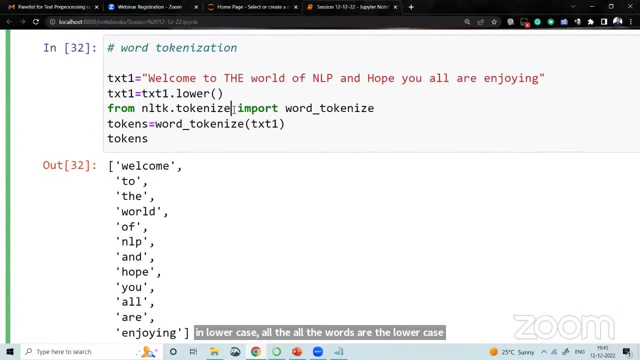 txt1.lower, then store it into the txt1.. Okay, and then go for the tokenization, So that all are in lowercase. All the all the words are in lowercase. Okay, so this is your word: tokenization. Let let's go for the sentence tokenization. 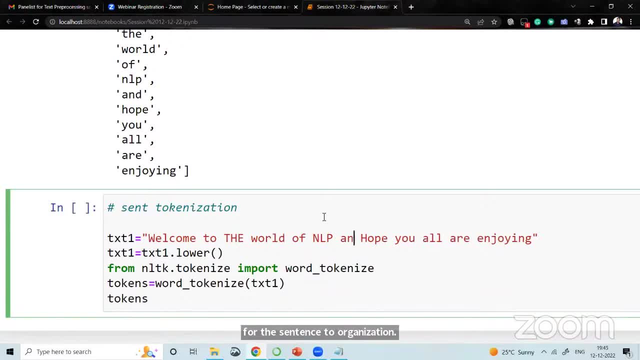 So for sentence tokenization, I'm considering the two sentence over here And now NLTKtokenize- you can use the sent underscore tokenize. Sent underscore tokenize. create the object of this sent underscore tokenize And you will get the sentence tokenization. 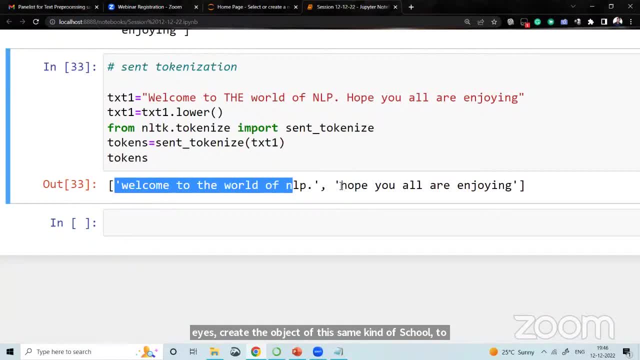 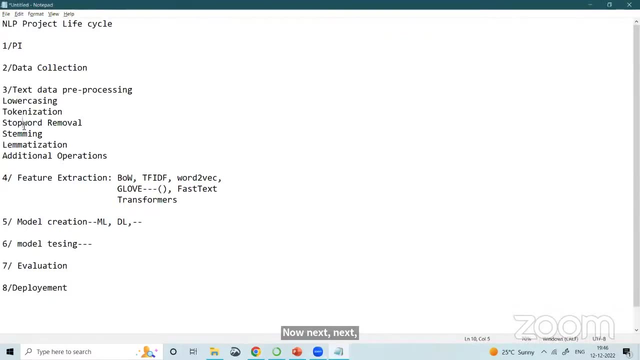 Okay, so this is my first and this is my second sentence. Okay, so this is how you can perform the sentence: tokenization Now, next. next is stop word removal. Okay, so lowercase tokenization is done Now. next is stop word removal. 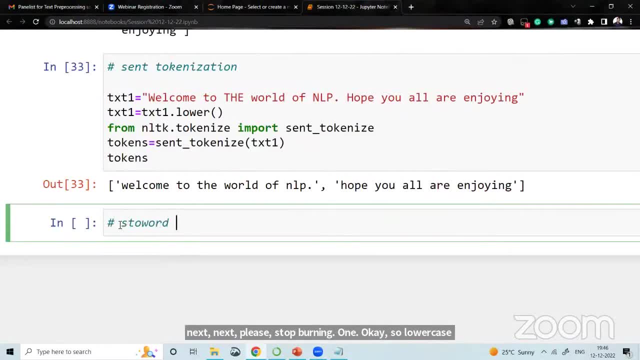 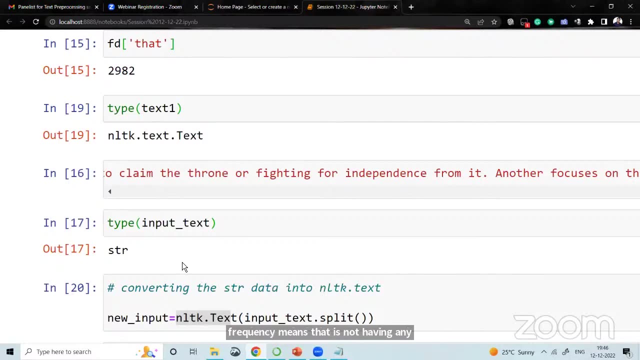 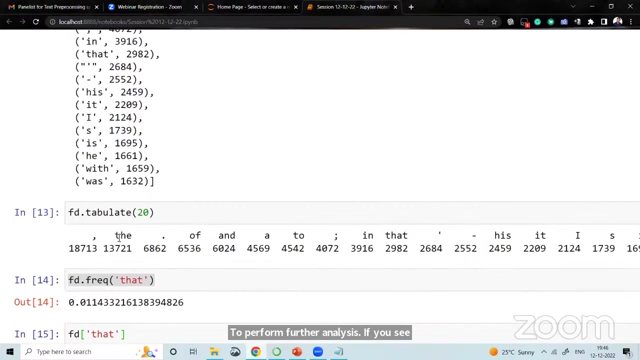 Stop word. Now, what do you mean by stop words? First, stop word means the high frequency words. High frequency, Okay, Means that is not having any lexical importance or significant significant importance to perform further analysis. If you see over here in this text you can find the frequency of these words. 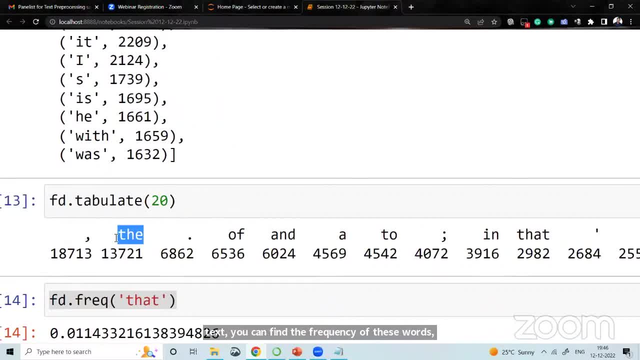 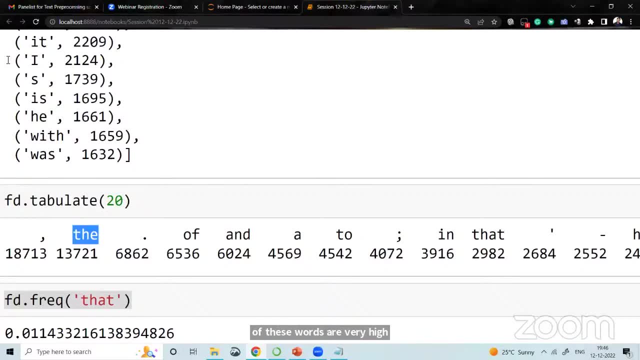 The and to. since then that: Okay, so the frequency of these words are very high. Okay, and when we worked on the NLP projects? Okay, So your data is very bulky. Okay, We do not want to provide the bulky data to your model. 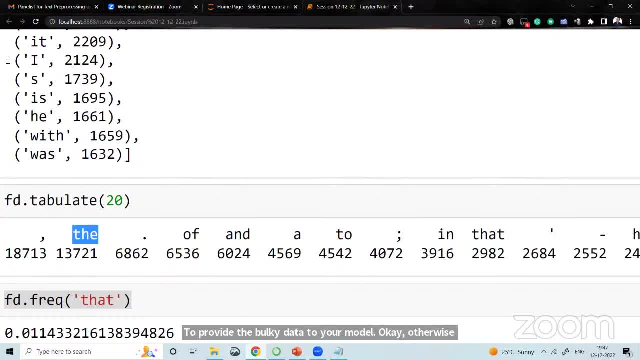 Okay, Otherwise your model will take a lot, much time and it gets confused. And because of that, we would like to remove this, all these unnecessary words, from the text, Because our focus is on the actual words. Okay, Like, the movie is good. 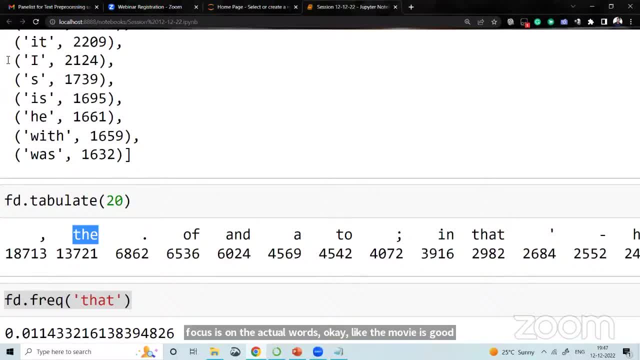 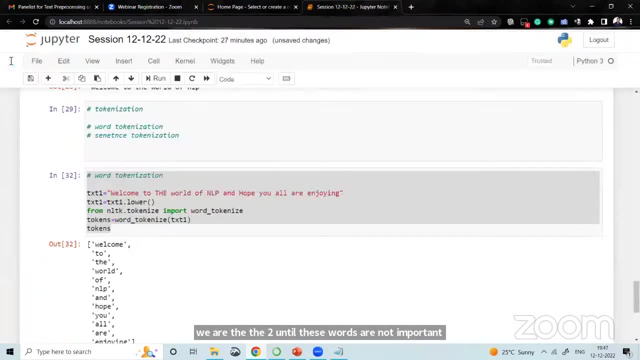 Okay, So we, we, we can focus on movie and good word. Okay, But the easy is not that much important for us, or the movie or the, the two until these words are not important for us. Okay, So stop. word means the high frequency word which is not having any significant importance for us. 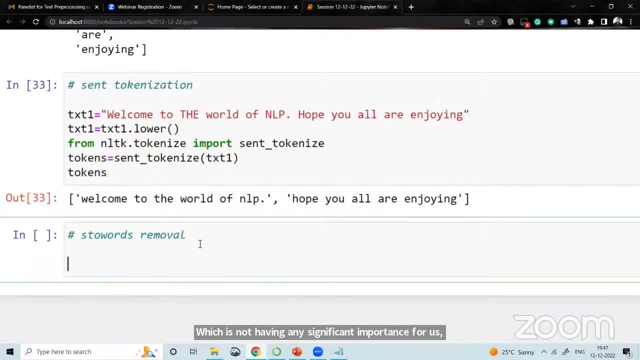 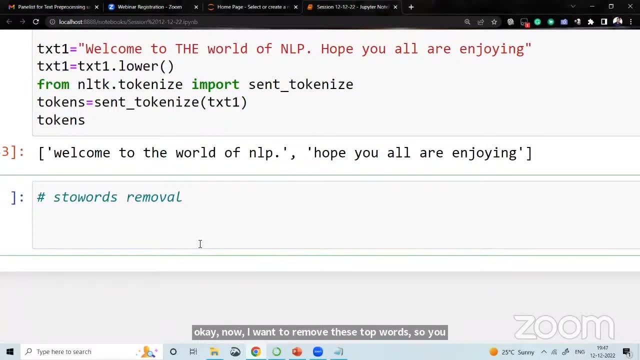 And because of that we go for the this stop word removal. Okay, Now I want to remove this stop words, So you should know what are the stop words. Okay, This: you need some text file where there, there, where you can. 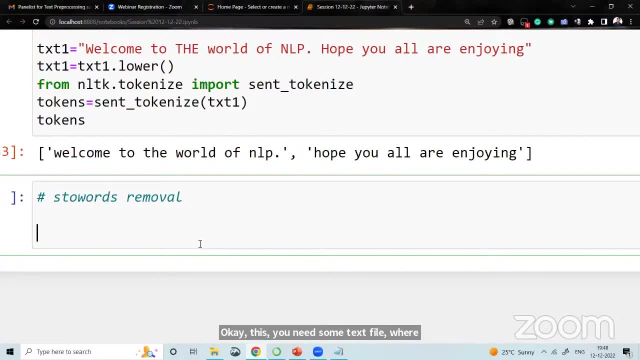 Okay, And where you can compare the stop words: Okay. So in NLTK library we have stop word file. So if you want to load this, you can use nltkcorpus. Okay, You can import stop words. Okay. So this is one purpose, where we have a list of files and under that files we have a set of words. 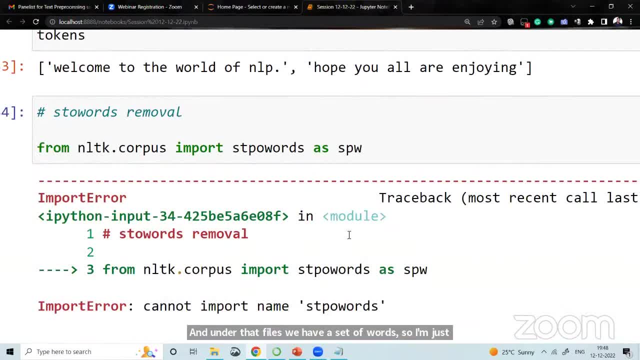 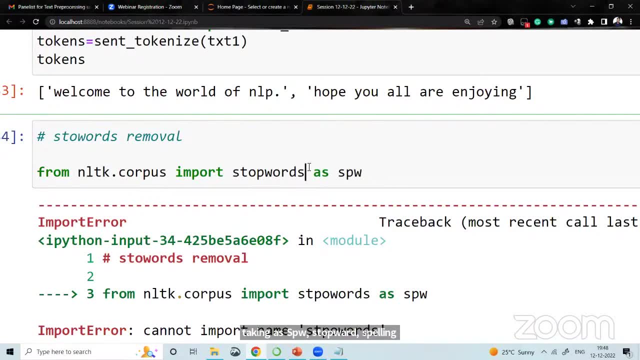 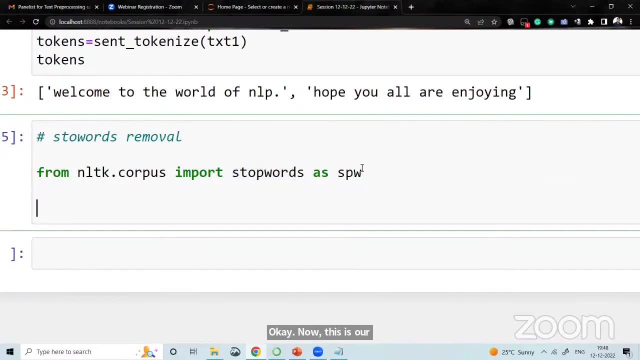 So I'm just taking as SPW. Okay, Stop word spelling, stop word. Okay, Now this is our corpus. under that we have different sets of files. Okay, So one method is there- file IDs, which is common method for all the corpuses. 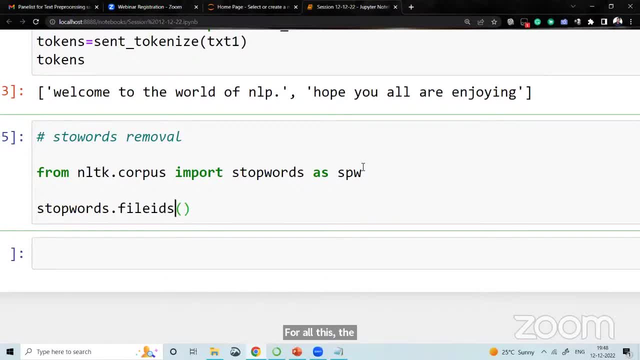 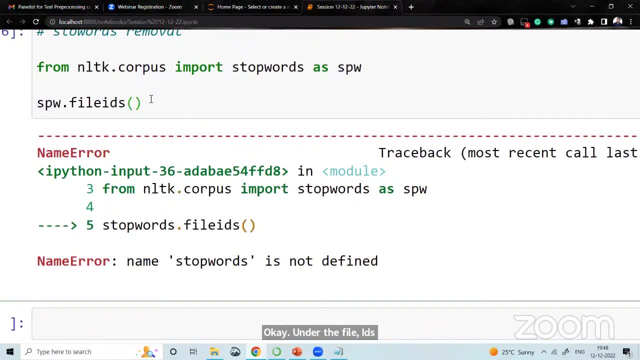 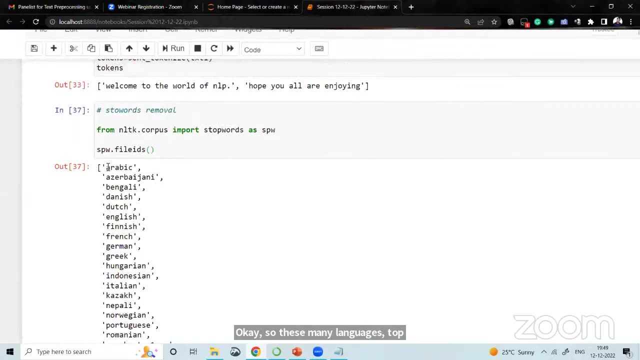 Okay, Under the file IDs: SPW, SPW. Okay, so these many languages stop words are present under the stop words, So you can get the Arabic language stop word. Bengali, Dutch, English. we are interested in English language purpose. 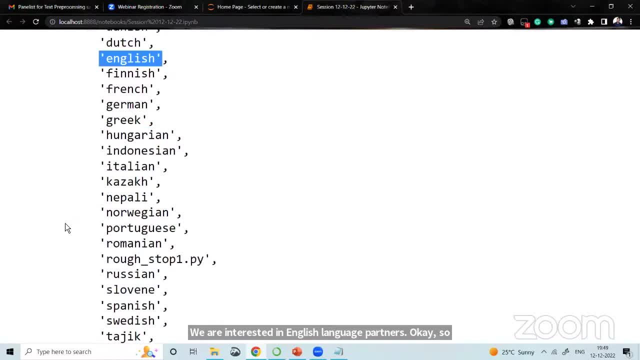 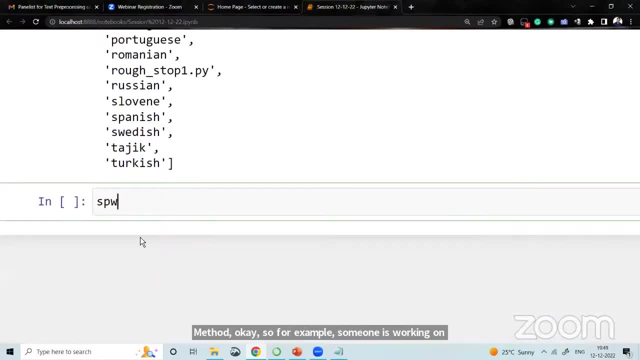 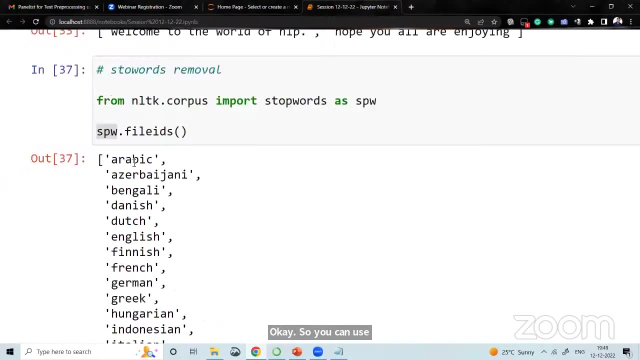 Okay. so if you would like to see this, you can use the dot word method. Okay so, for example, someone is working on Arabic project, Arabic language project. okay, so you can use words and you can pass the Arabic. 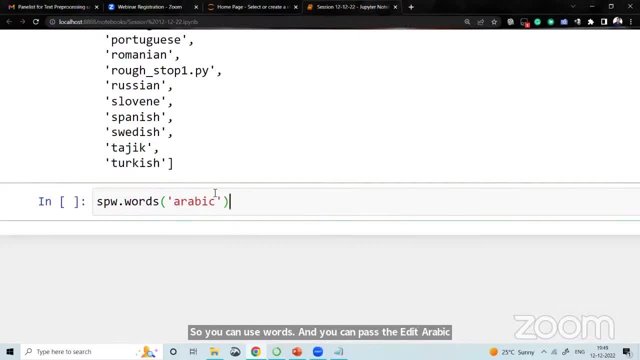 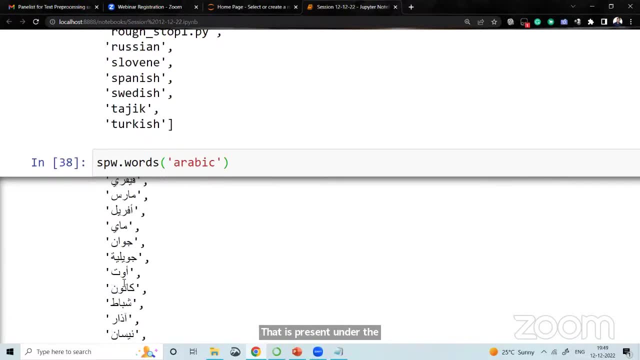 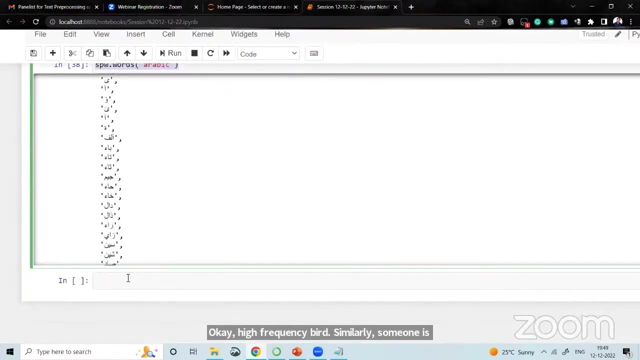 So you get the set of stop word. okay, list of stop word that is present under the Arabic: Okay. so all these are the Arabic words. Okay, high frequency word. Similarly, someone is interested in stop words associated with the Dutch. 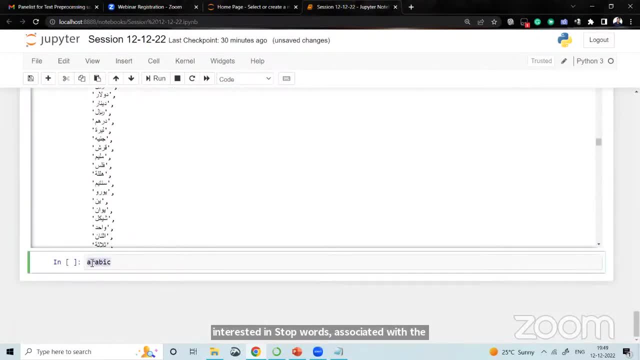 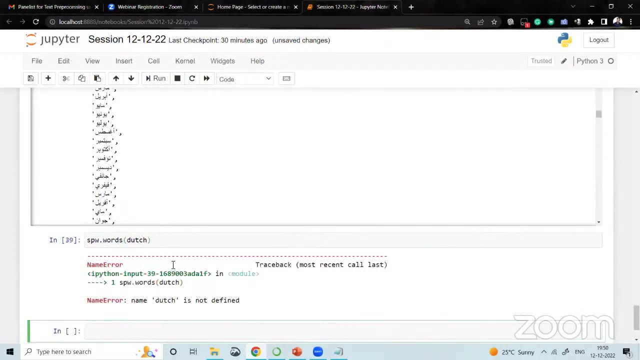 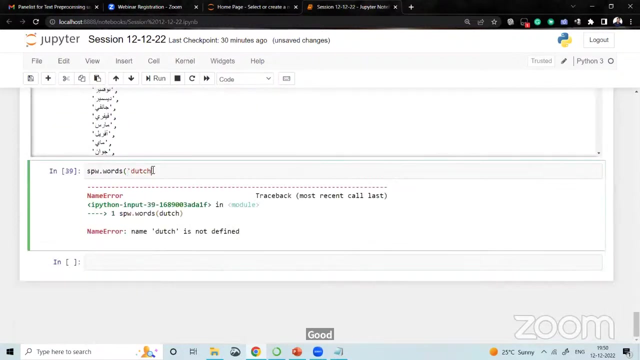 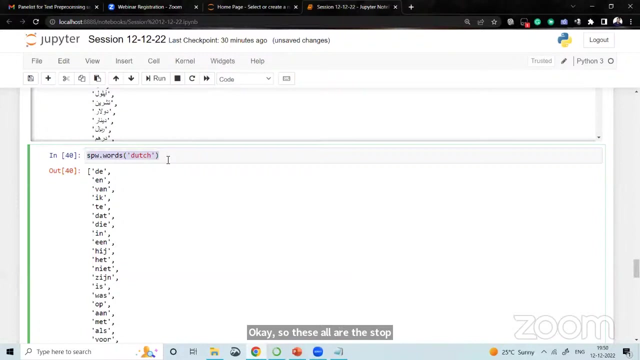 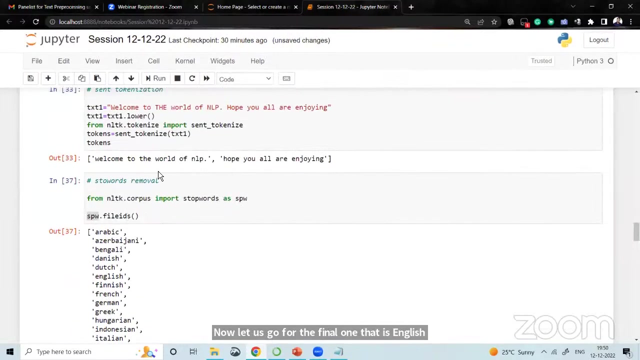 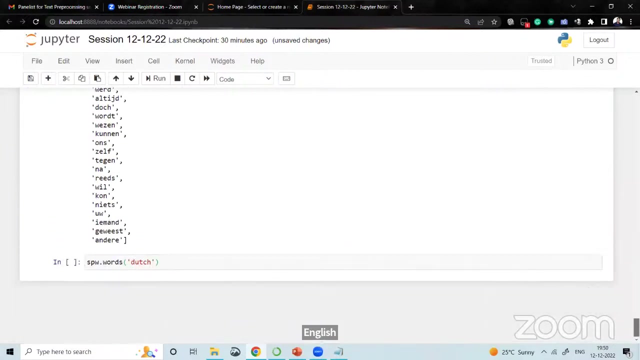 Okay, so you can write here spw dot words and you get the Dutch. Okay, so these all are the stop words. That is Okay, Under the Dutch language. Now let us go for the final one, that is, English language. English, okay, so all these words. 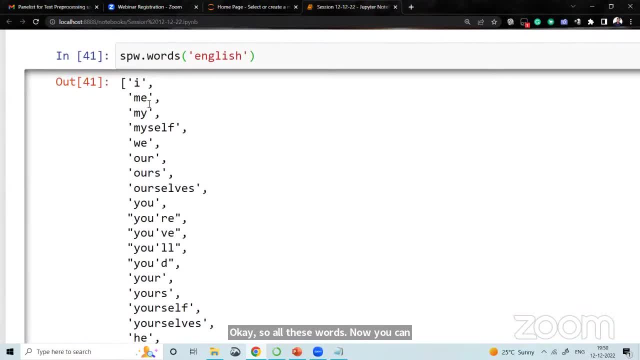 now you can find here, these all are the words: high frequency word: I, me, myself, our, you are, he is himself. Okay, so frequency of words: These words are very high in the text and you can find these, the frequency of these words, maximum. okay, maximum frequency. you get it for these words, okay. 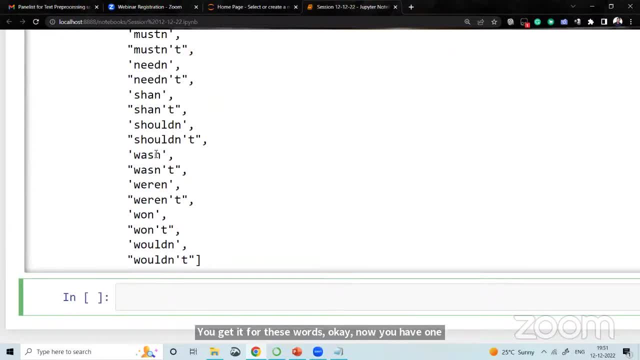 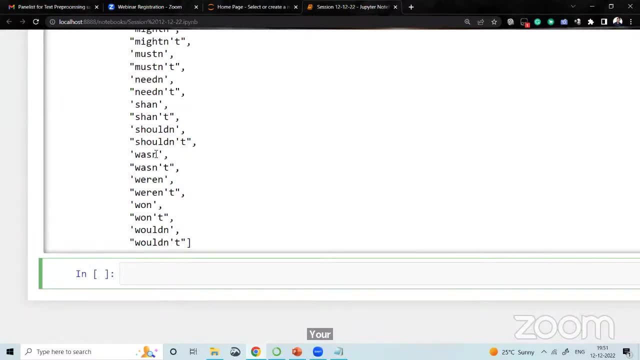 Now you have one reference file by which you can check your text file. okay, Now I would like to remove the remove my stop words. Okay, So let me take one line, PhD one. Okay, I'm writing here. Aman is one guy, guy from India, who will take care of people around. 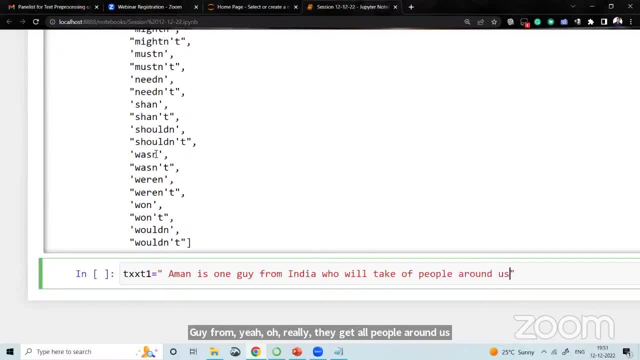 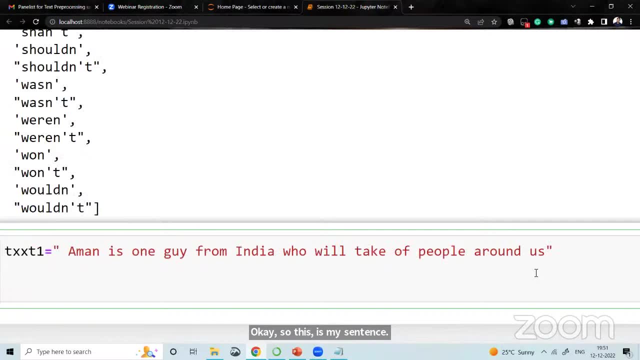 us. Okay, so this is my sentence. okay, And I would like to remove the stop words from this sentence. Okay, so this is my sentence. Okay, And I would like to remove the stop words from this sentence. Okay, so this is my sentence. 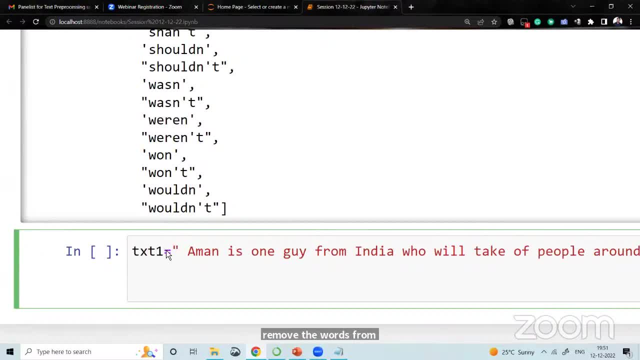 Okay, And I would like to remove this text file. Text one: Okay, this is a word text, So first I'm going to convert it into the lowercase. As you all know, you need to avoid the confusion, So lower casing is the first step. 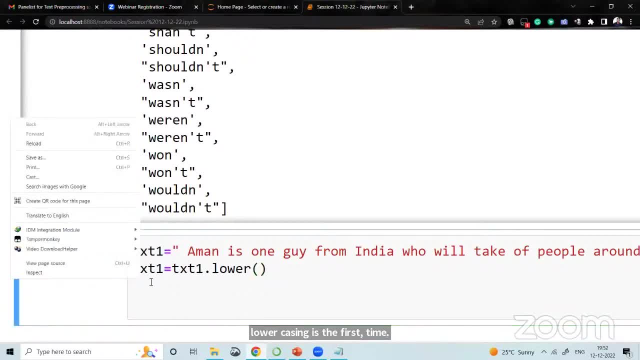 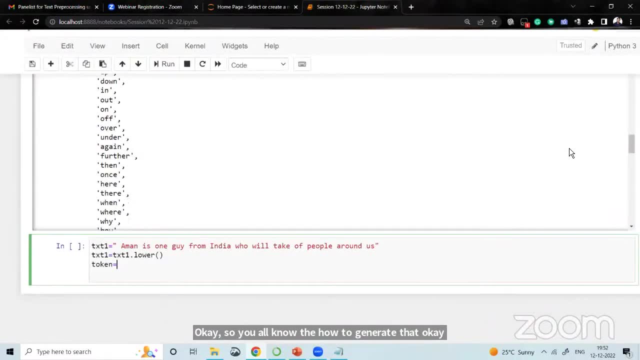 Second step is to do the tokenization. Okay, so I'm going to generate the tokens. Okay, so you all know the how to generate the token. We have this tokenizer, word tokenizer, So let me write here Directly. I'm writing here: 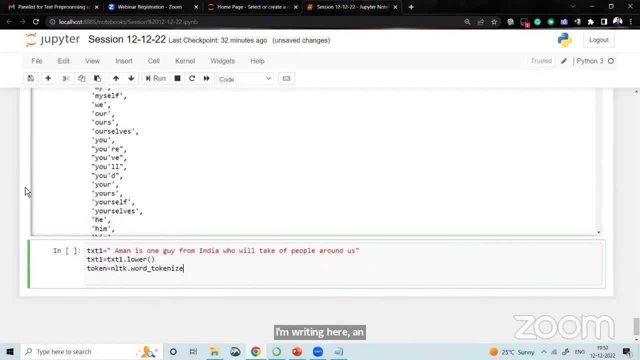 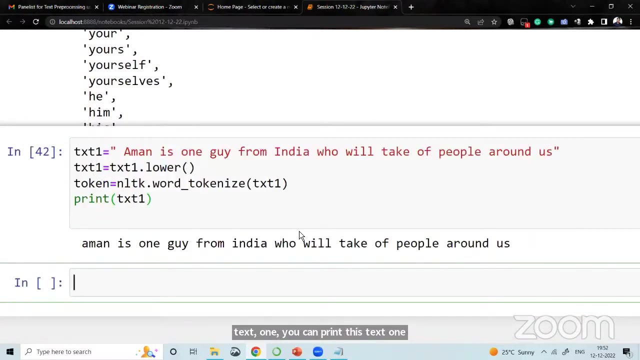 dot, word underscore: tokenize. okay, and you can pass the text one. okay, this is your text one. you can print this text one. print text one and uh, okay, sorry, not text one. i'm going to print the tokens, okay. so these all are the tokens, okay. so this is the list of words that we have now. 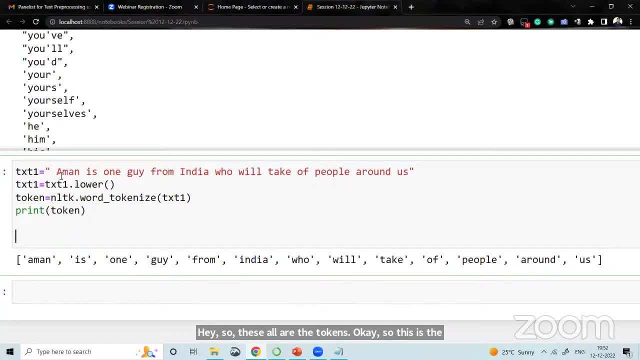 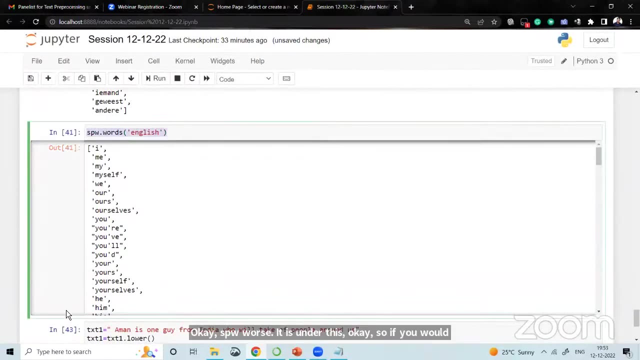 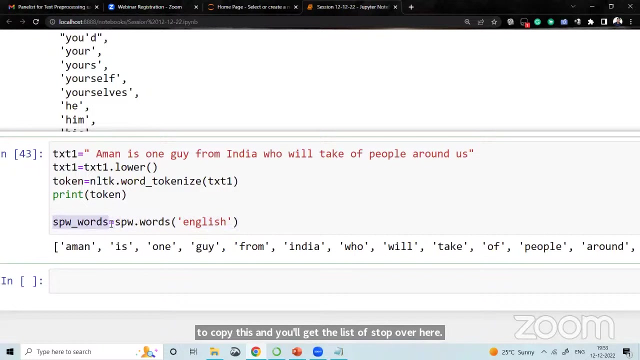 let's go for the removing the stop word. okay, so you all know the list of words. okay. so spw words. okay, spw words. it is under this, okay. so if you copy this and you'll get the list of stop word over here, okay, with this line, you get the list of stop word from the english language. okay. 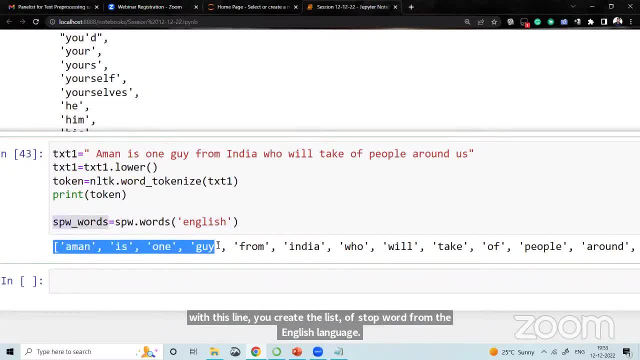 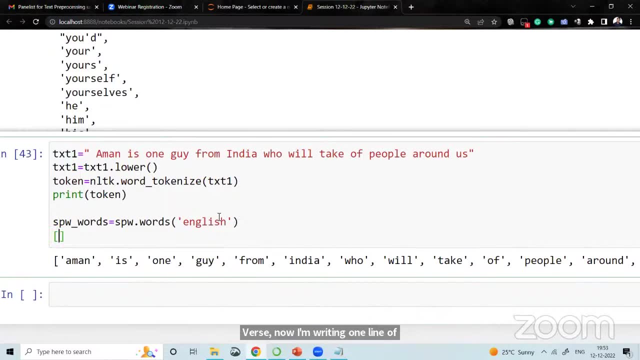 and you can compare your work, your list, with this and remove the stop word. now i'm writing one line of code, so w for w, w for w in. okay, so in my tokens, basically in tokens, and then write if w not in, not in this spw words. 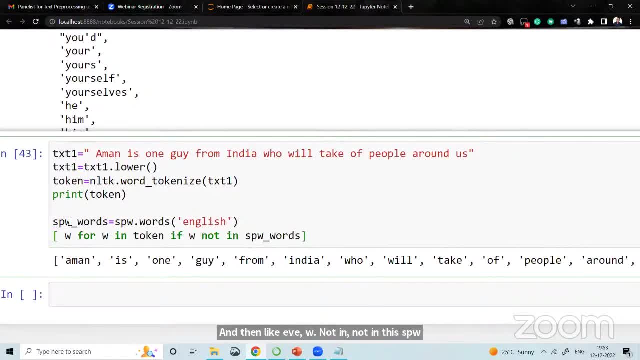 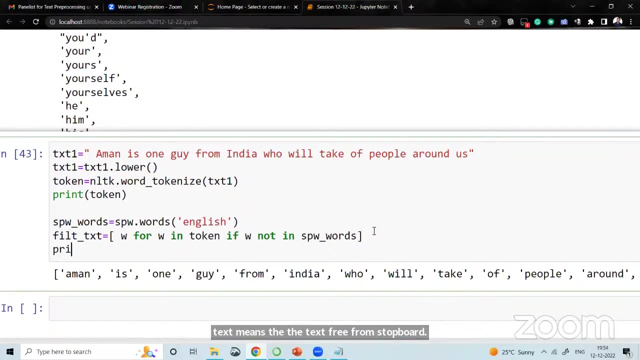 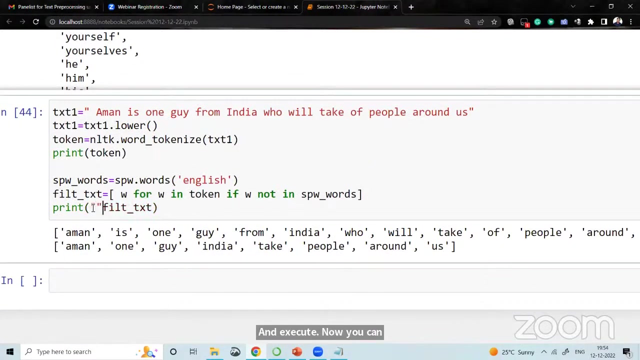 okay, and this is your filter code words. filter words means the, the words, uh, filter text i'm writing here. filter text means the, the text free from stop word. okay, and let me print it and execute. now you can find here. so this is my raw, raw text. let me write it properly: raw text. 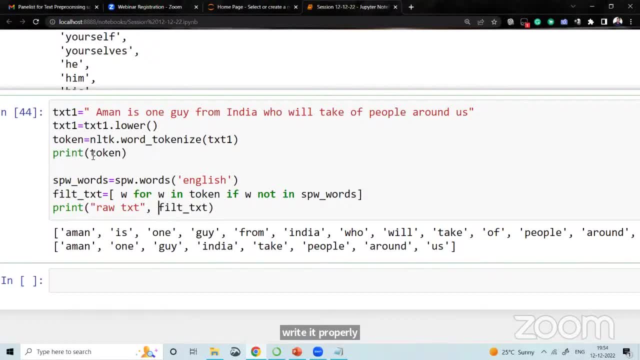 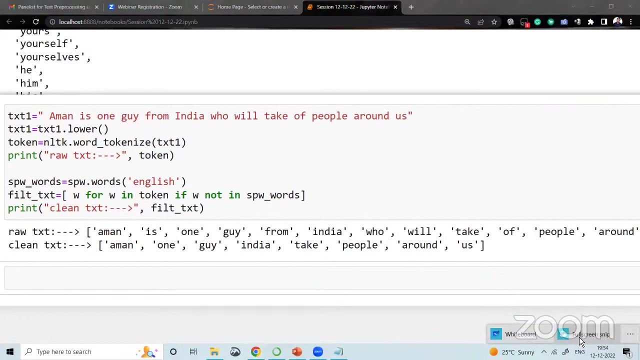 okay, and this is my. uh, no, no, this is my clean text, clean text after stockboard removalство and summary text, and this is my raw text. uh, okay, so you can find here we removed. Ok, so you can find here we removed. with this line of code, with this single line of code, we have removed the stop word from the. 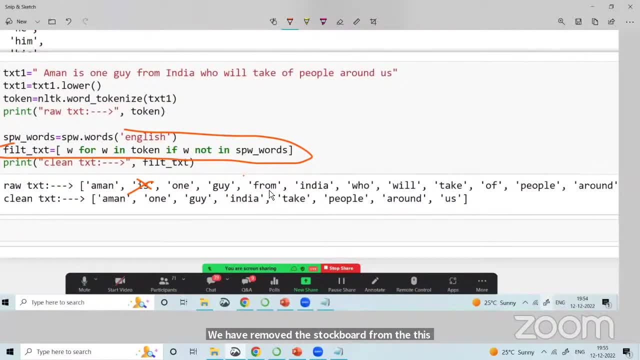 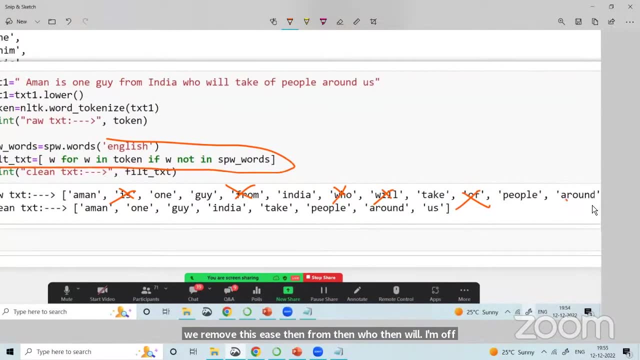 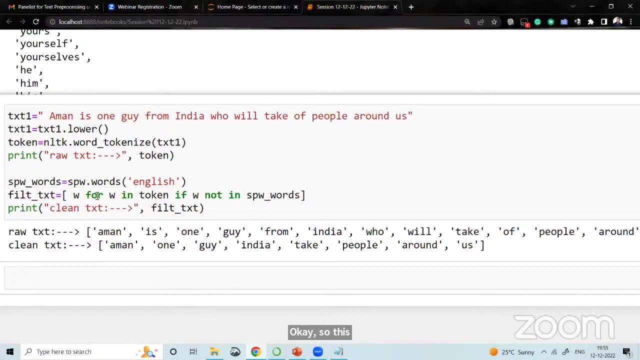 this text: okay, we remove this. is then from then. who then will? and of okay, and another okay. so this is my stop word, which we have removed from my short text. i hope the stop word removal is clear, okay. so this is how one can remove the stop word from the uh the text file now. next is: 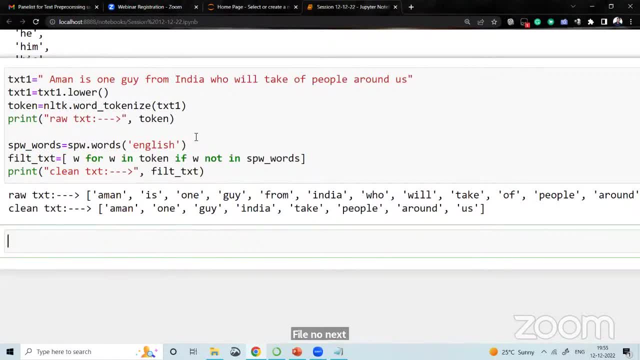 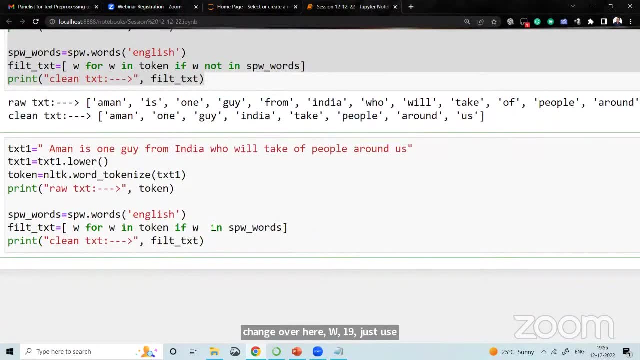 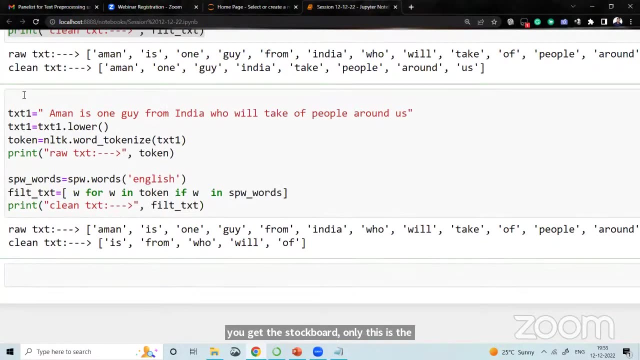 next you can. if you would like to print the stop word only okay, so just change over here. if w not in, just use only in. okay, so you get the stop word. only see over here. this is the code for getting the stop word. getting the stop word from: 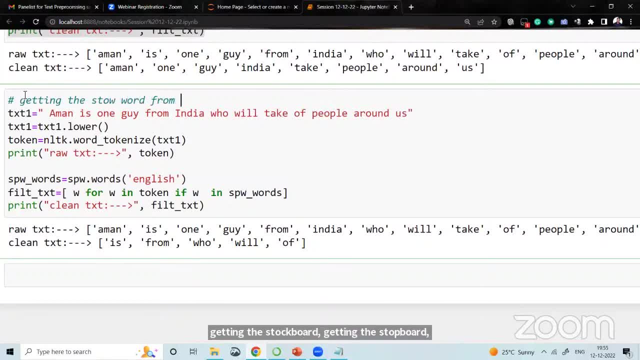 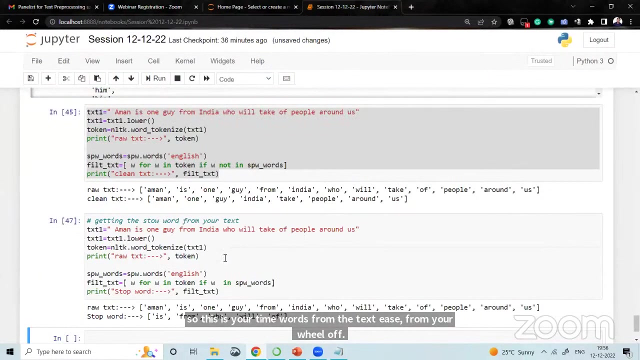 okay from your text. okay from your text. these many stop words. are there stop words? okay, so this is your stop words from the text. is from: who will off? okay, okay, only one change is required: instead of not in, i'm going to use in. okay, i'll use the. 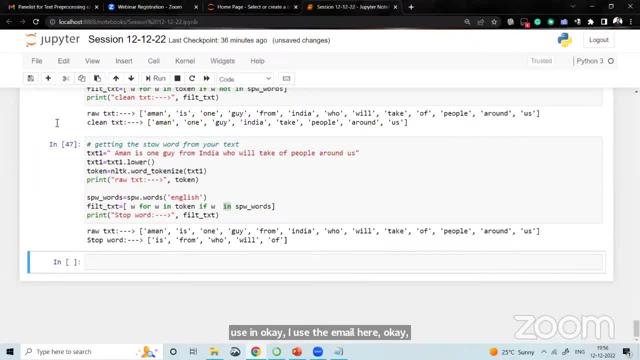 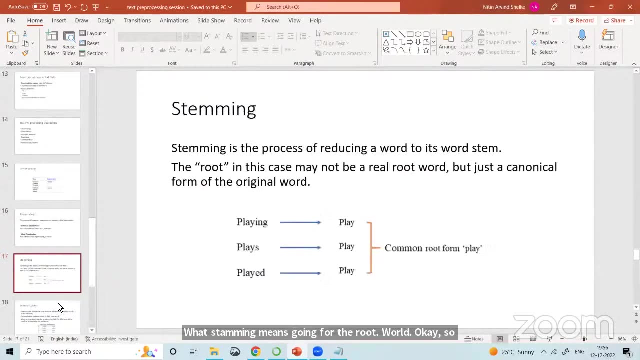 in over here. okay, so this is related with the stop word. now, next is your stemming. okay, so stemming means what? stemming means going for the root word. okay, so we are not interested in the. okay. so stemming means it is a process of reducing the word to its word stem. okay, so, for example, 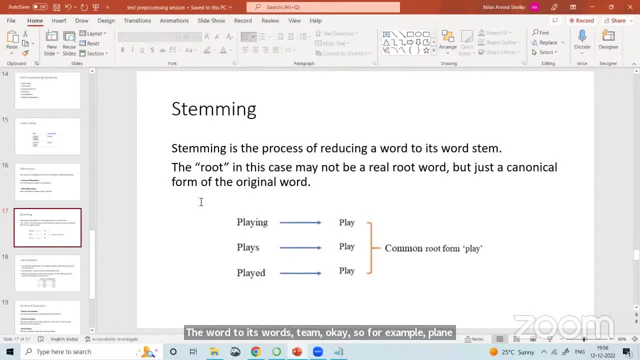 playing is one word, plays is another word and played is another word. okay, so all three words are same. okay, so to just to know the root word for this: okay, so, internally, when, when we give this data to the model, that time we cannot give it as it is. okay, so it will create the confusion because 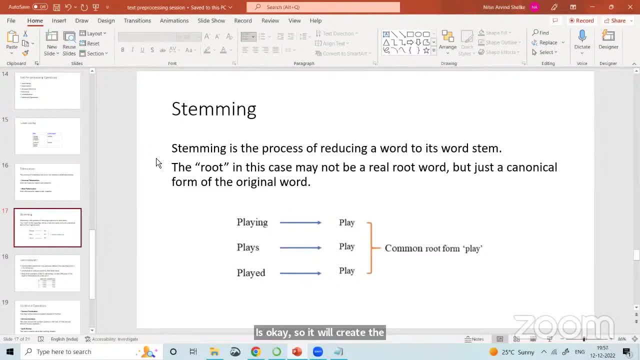 playing is having the different sense. okay, different sense in terms of vector, different word representation or different vector representation is for playing and different vector representation for plays, although both word are same. okay, and because of that your model will get confused in the future. so, to avoid this, we convert this word to the root word. okay, so your playing is get converted into the. 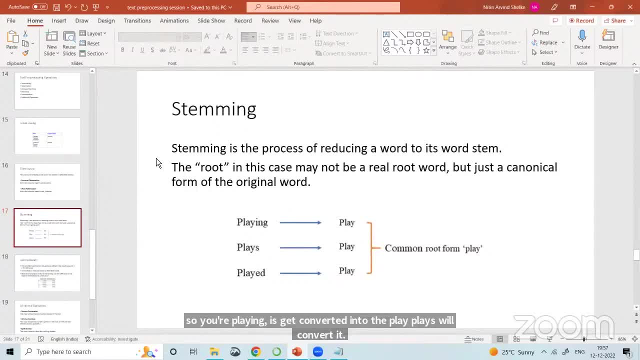 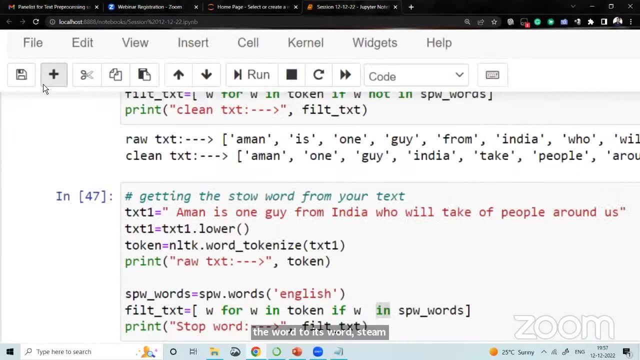 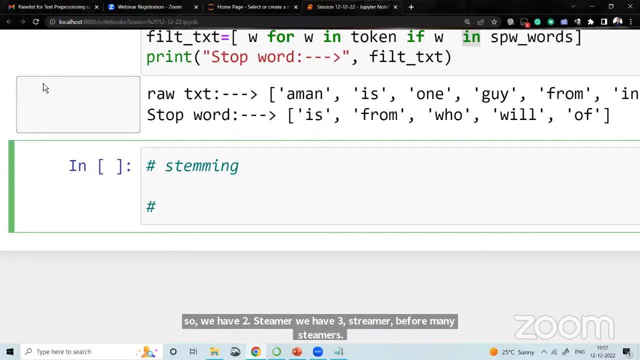 play plays will convert into the play. so stemming is the process of reducing the word to its word stem. okay, so we have two stemmer, we have three stemmer, many stemmers also, actually, but most only use porter streamer and Lancaster streamer. apart from that, if we have lansnowball steamer also, 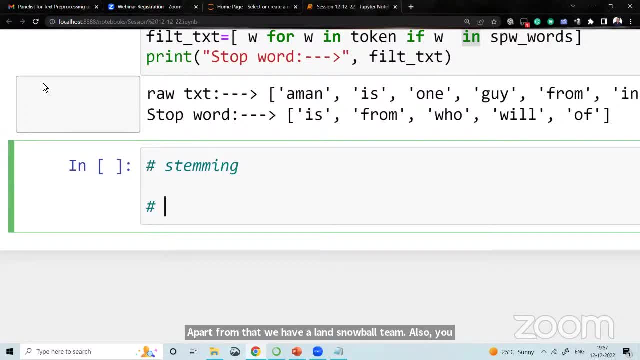 you can create your own steamers. one streamer means by the help of regular expression. you can create your own streamer also, like by adding EDIES, IOUS ING. okay, these are the words. at the last word you can write one regular expression, place some- uh- the prefixes and remove that one. okay, you get the root. 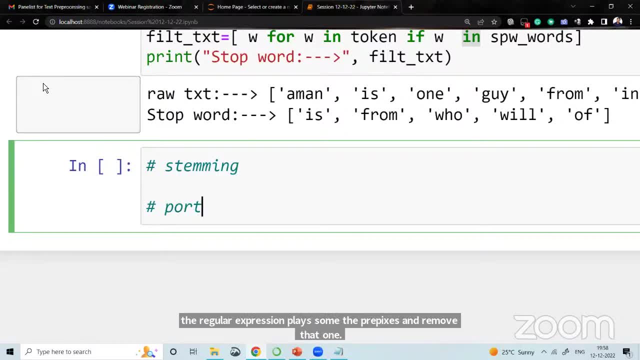 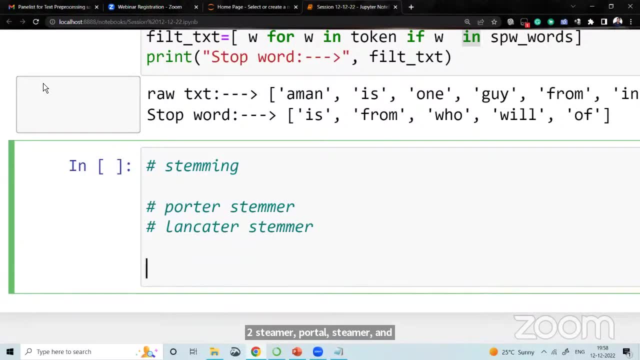 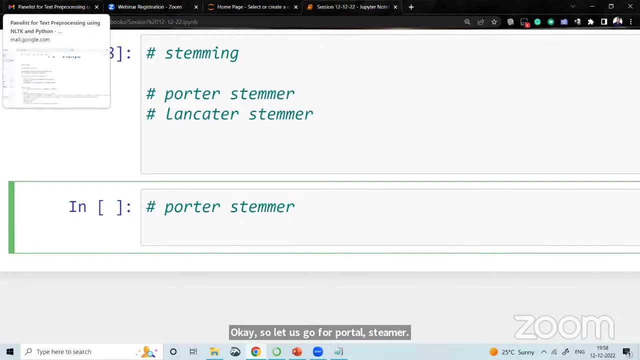 Here I am going to explain two steamers: portal steamer and then Lancaster steamer. So let us go for portal steamer. So portal steamer. let us check the words On list. I am considering word playing, then plays and played these three words. 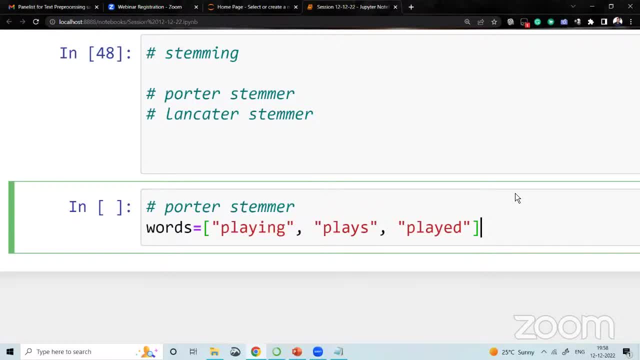 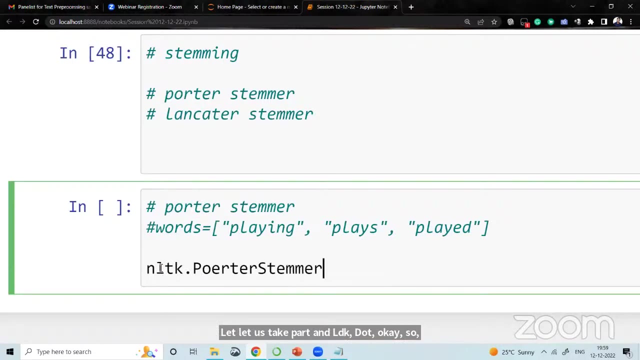 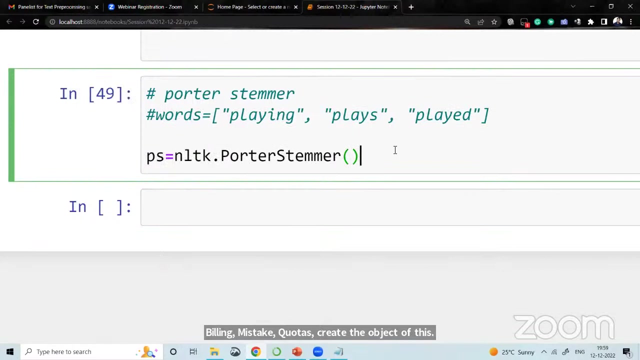 Let us stick for NLTK dot so you can directly go for NLTK NLTK dot portal. steamer spelling mistake portal. create the object of this. yes, let me check. Yeah, PS is the object of this portal, steamer class, and you can pass the word. 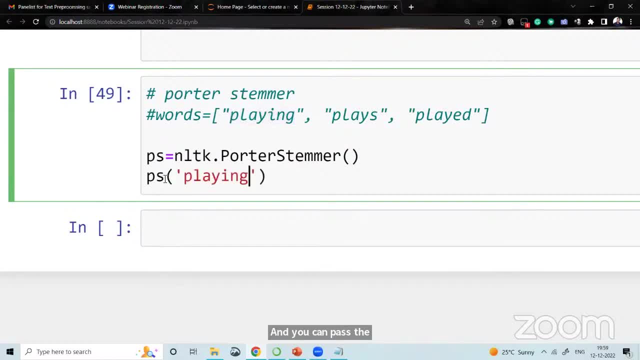 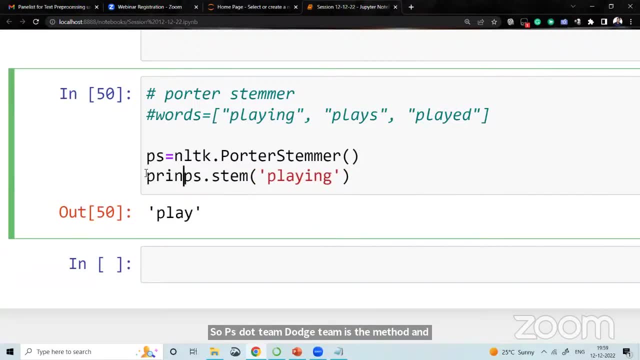 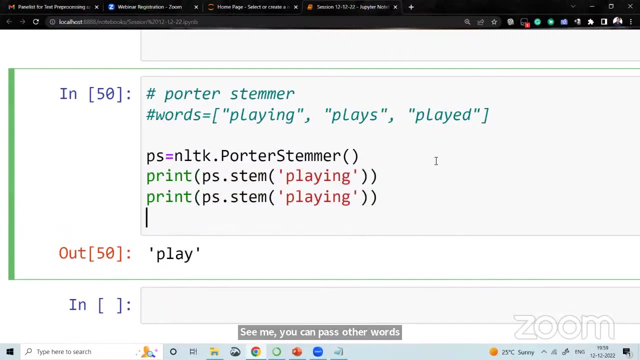 For example, I am passing the play. Okay, So PS, dot, steam, dot steam is the method and you'll get the play. Similarly, you can pass other words. This is your first, I'm passing it separately. plays, Then played, okay. 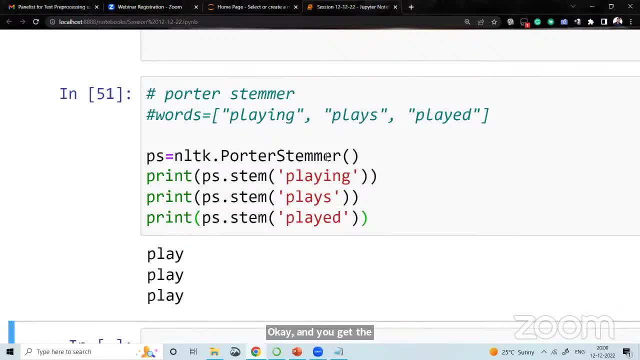 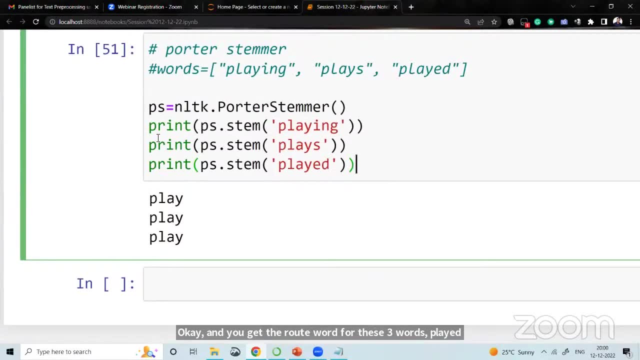 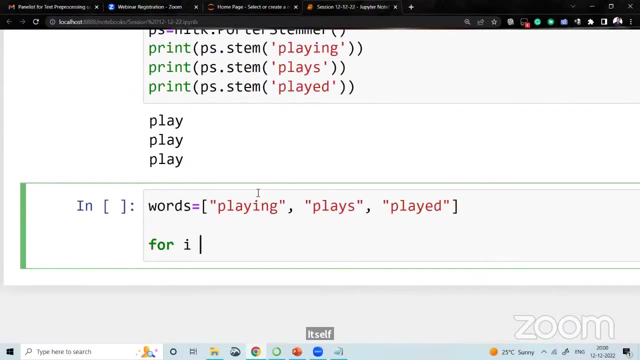 And you get the root word. So root word for these three words: play, play, play. Okay. If you would like to write it for the list itself, okay, Then take this list, write the loop, or, in your words: this is your list. 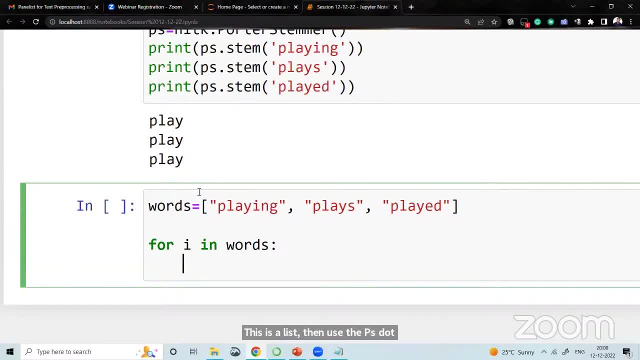 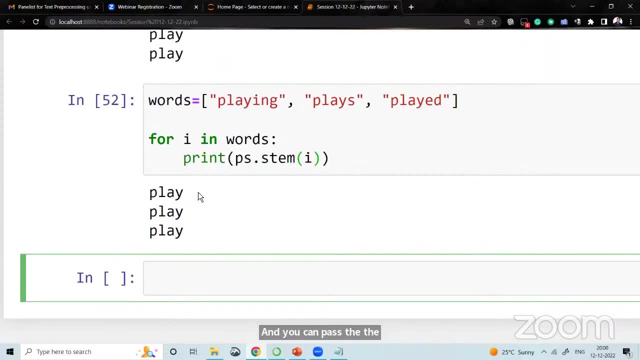 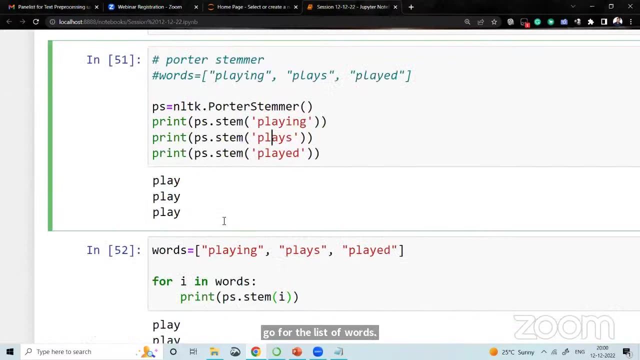 Then use the PS dot steam, print PS dot steam And you can pass the the I. Okay, So this is how you can go for the list of words Now. similarly, we have Lancaster steamer, Lancaster or different steamer. 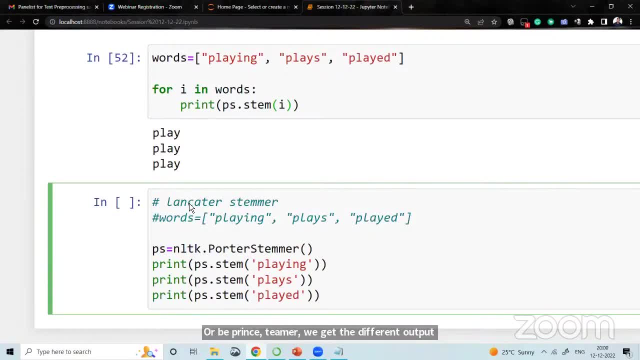 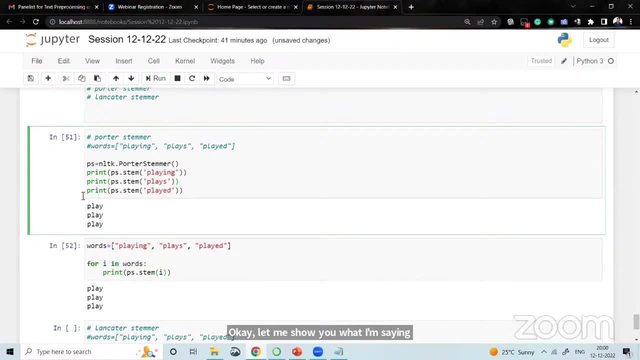 We get the different output, Okay. So it is not every time that you are getting the correct word. Okay, Let me show you what I'm saying. What do you mean by correct word? So, for example, I'm going to say the correct word. 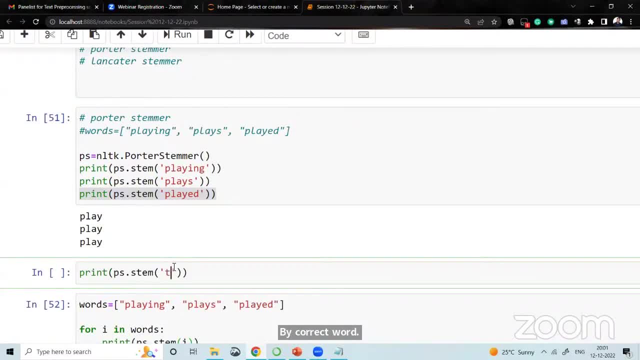 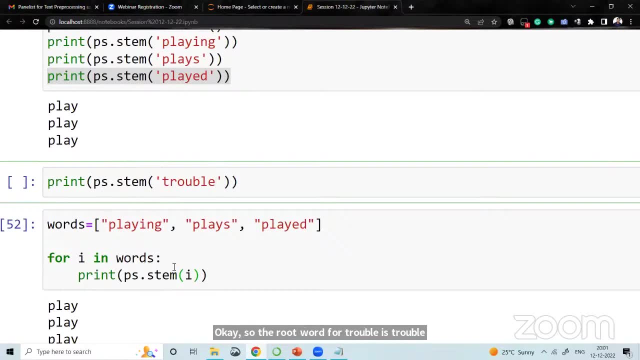 I'm going for the word like trouble, Okay, So the root word for trouble is trouble. Trouble itself. It is my root word, Okay, But when I'm going with the water steamer, I'm getting this wrong word. E R O U B? L. 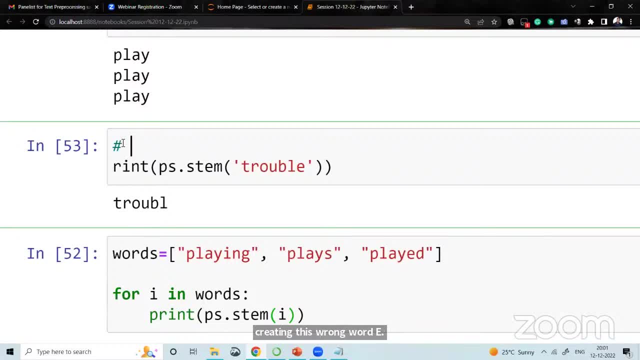 Okay, So here I'm getting the wrong output. Okay, So only because of what? under Porter steamer, we do not have any type of condition checking that, whether it is a correct word or not. Okay, It automatically remove the prefix. Okay. 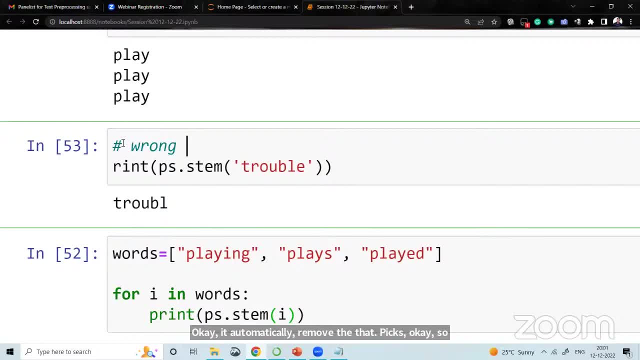 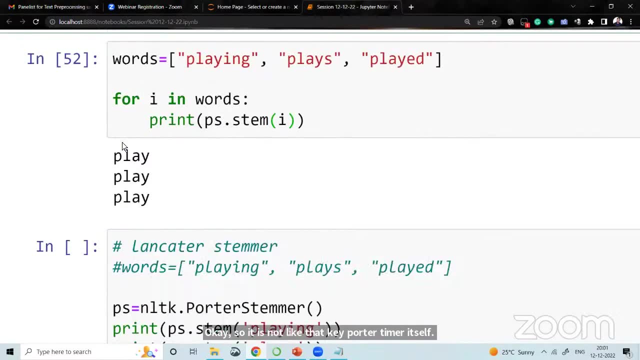 So because of that you are getting the wrong word, Okay. So it is not like that. in Porter steamer itself you are getting some wrong result In Lancaster steamer, sometimes Lancaster works well, sometimes Porter works well, Okay. So this is one thing. 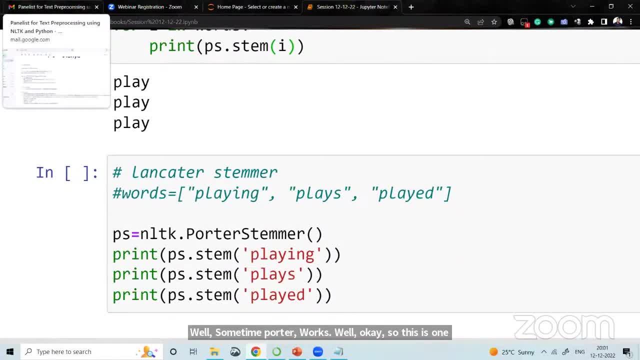 And that problem will get resolved when we go for the discussion, when we go for the lemmatization concept. Okay, Under the lemmatization, this problem will get resolved under the lemmatization. Lemmatization is also the way to get the root word, but every time you get the correct. 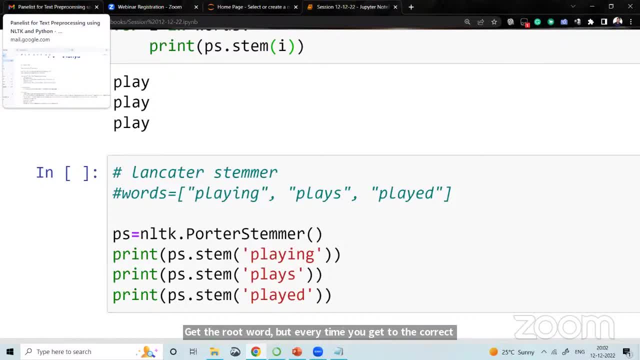 word. because there is one thing, the one extra headache, that uh the word is compared with the uh the dictionary, or in in uh in NLTK we call it as wordnet. Okay, That I will explain later. 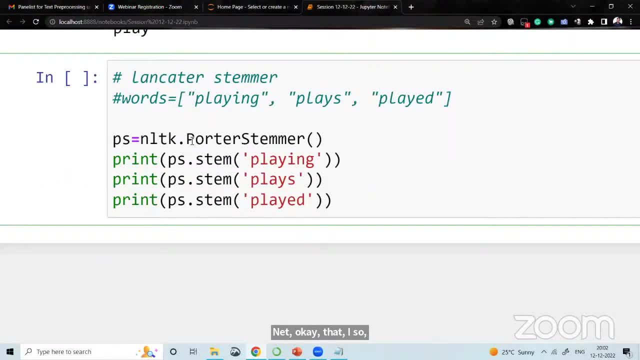 So, um, Lancaster, let me create the Lancaster steamer. Okay, Lancasters. okay, Spelling mistake: Lancaster, Okay, So LS, I'm considering LS over here, or Lancaster steamer. replace PS by LS, LS and LS. 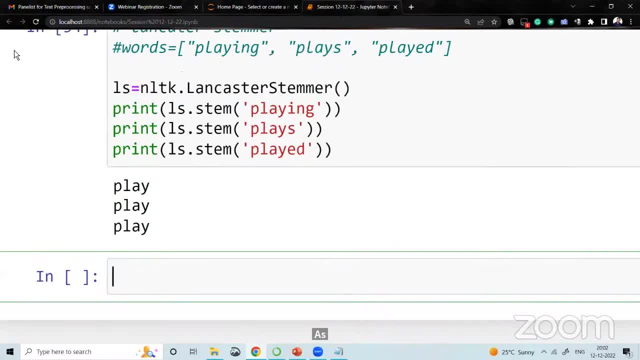 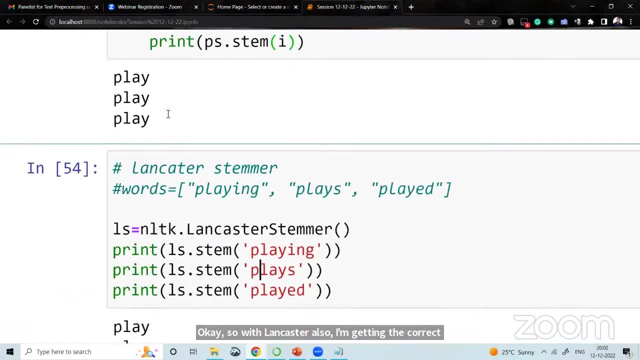 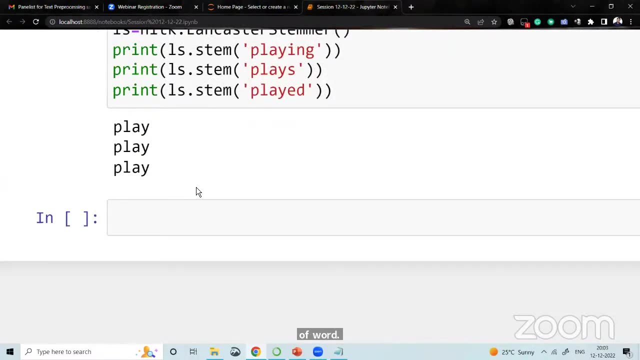 Similarly, you go for the snowball steamers- Okay. So with Lancaster also? uh, I'm getting the correct result for this, Okay, And you can try for this list of words, Okay. So every time it is not possible that we get the correct result. 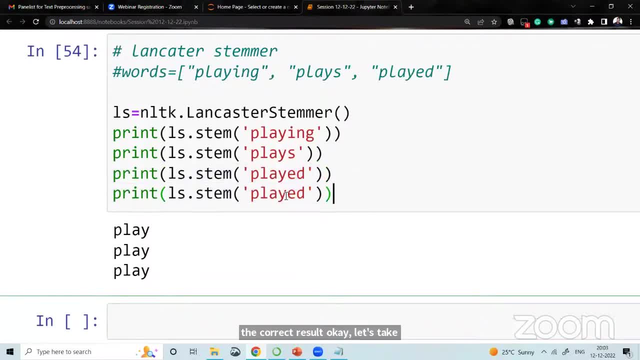 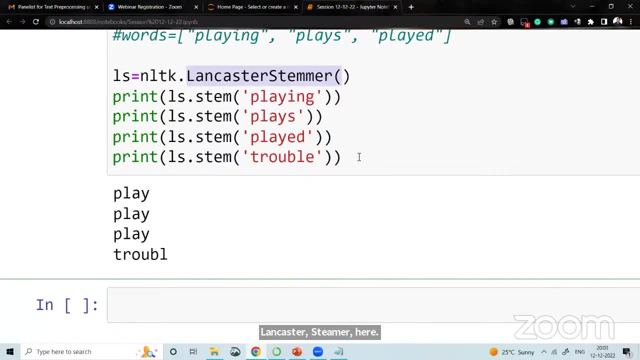 Okay, Let's take one more word for Lancaster steamer here Trouble. Okay, So you can find here when we, when we are going with the Lancaster steamer also, we are getting the wrong output for the trouble Wrong, wrong output. 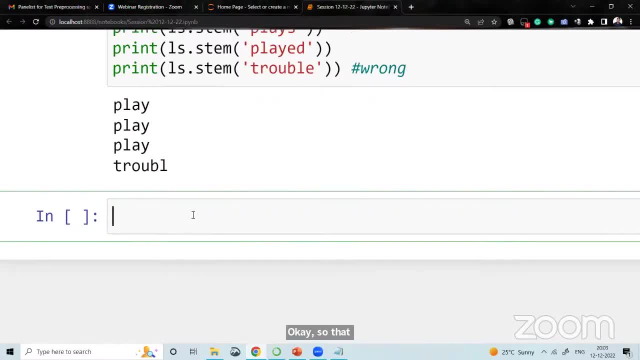 Okay, So that problem is now get resolved In the lemmatization concept. So under the lemmatization what we have lemmatization- we call it as a word- net lemmatizer that only remove the affixes. 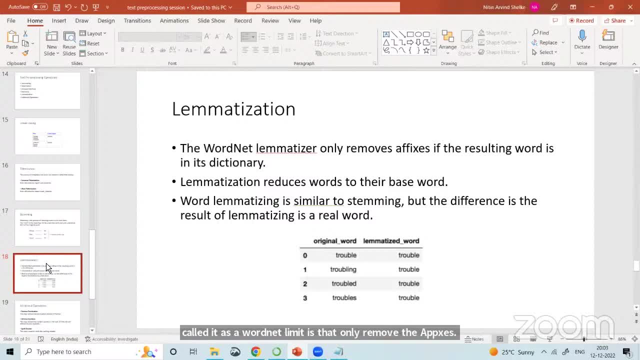 If the resulting word is in the dictionary. resulting word is in dictionary means it is a word net basically. So under the NLTK we have a word net purpose. there We have a set of standard words that we call it as a dictionary. 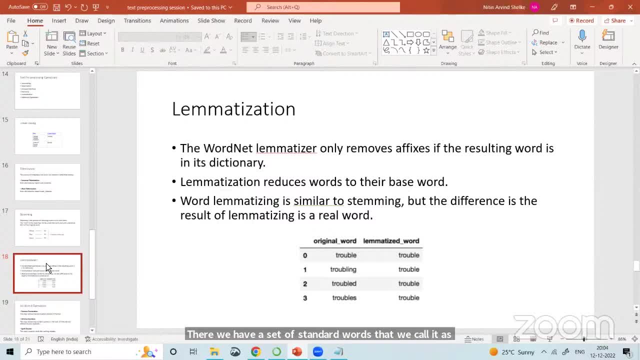 Lemmatization. Lemmatization reduce the word to their root word. It is similar to the stemming concept, but the difference is that the result of this lemmatization is only the real word. real word, You will not get the wrong word. 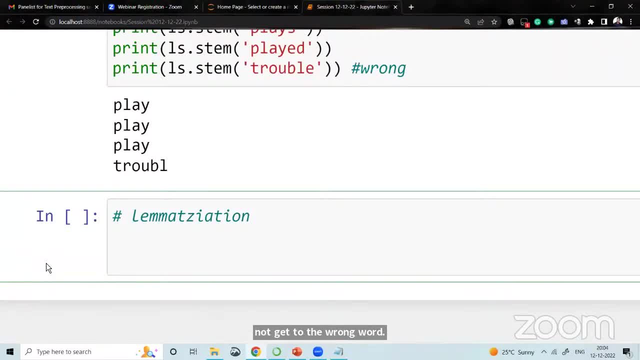 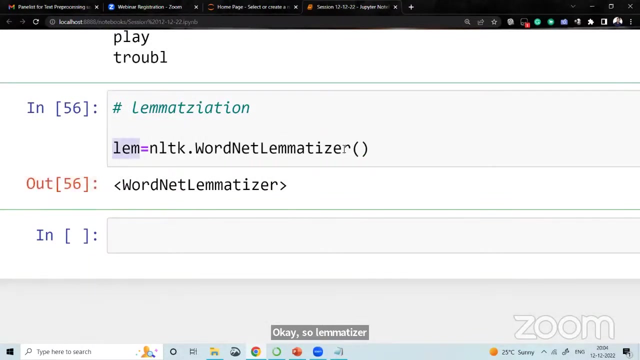 Okay, So, uh, how to go for the lemmatization? So again, NLTK dot, your word net lemmatizer. Okay So, let me write: word net lemmatizer: L E M dot lemmatize. 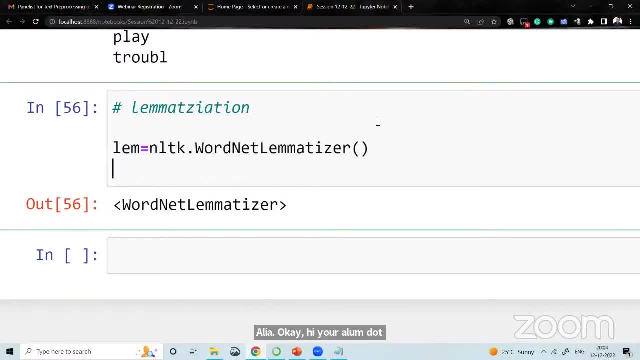 Okay, You are L E M dot lemmatize. Okay, Lemmatize is the method, L E M dot lemmatize And you can pass the word trouble Okay. So now you are getting the trouble. correct result. 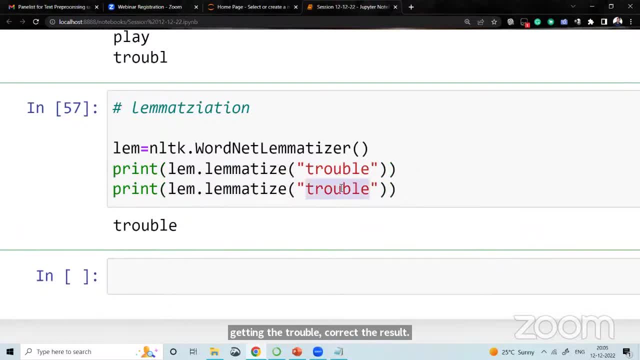 But the thing is that it is the disadvantage of using the lemmatization is that it is time consuming because one extra headache is there. okay, first it remove the affixes and then it compare with the word net. okay, so because of that you can find over here it will take some time. okay, so it will take some time. 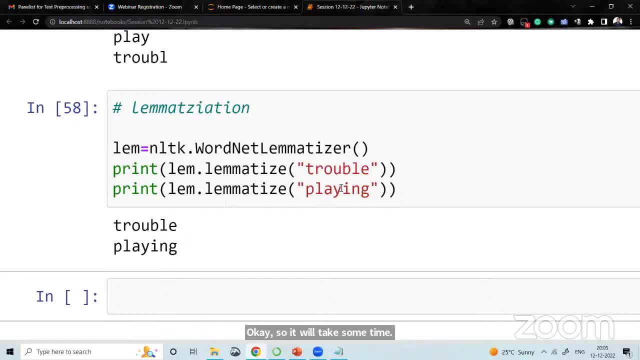 okay as this is, these are only two words. that's because of that you are not getting the time constraint over here, but internally it is. the disadvantage of lemmatization is that there is a extra headache of comparing the, the word, with the, the root word, the. 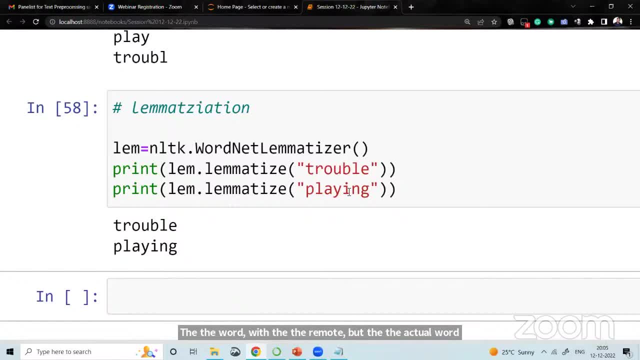 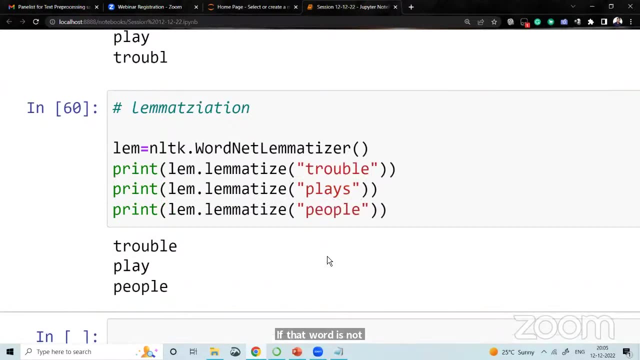 the actual word. okay, so let me write another one place or some word if that word is not defined in the dictionary: okay, then you will not get it. okay, so let me write another one place or some word if that word is not defined in the dictionary. like people: okay, for people also, we are getting the correct result. let me type here: people for. 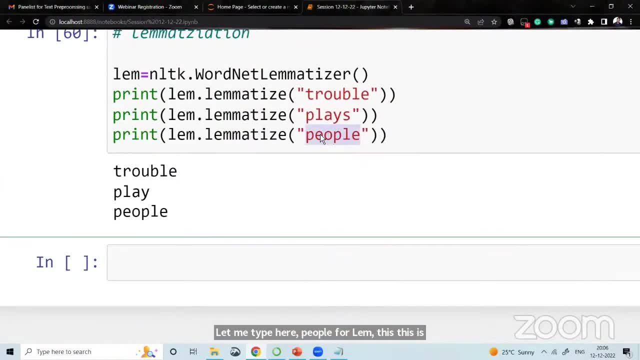 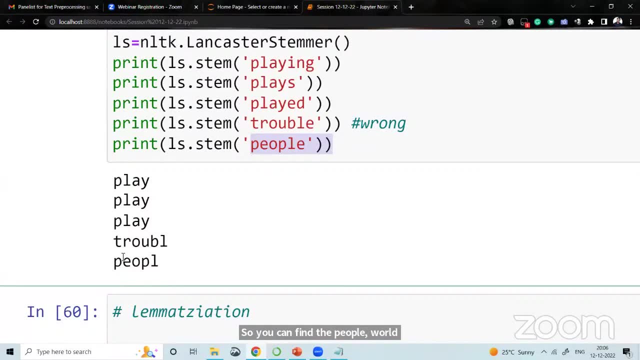 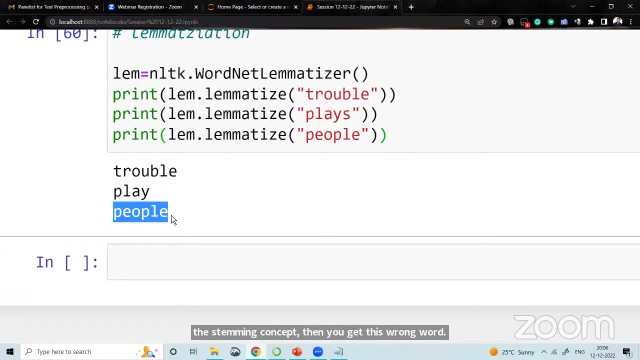 this is lancaster steamer and i'm typing the people over here so you can find the people word. when we are going with the stemming concept, then you get this wrong word- okay. but in lemmatization you will always get the correct word, okay. so this is what the concept. 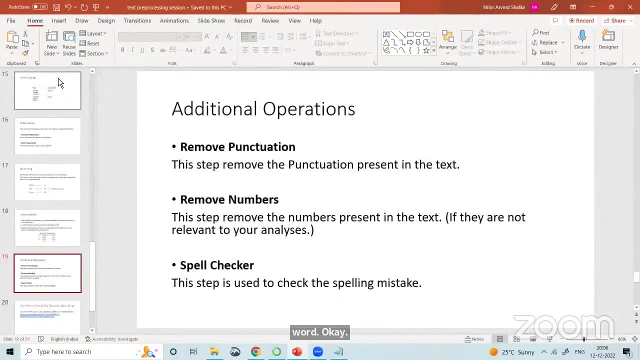 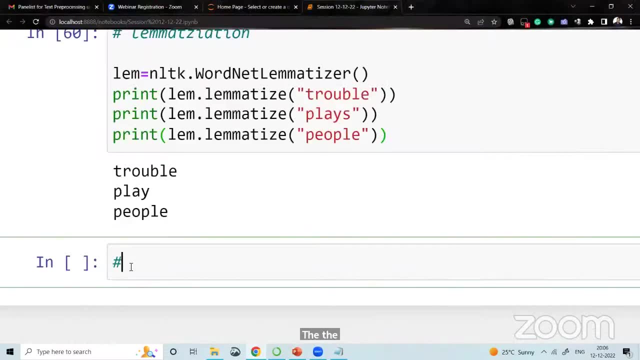 of lemmatization is. so let me write another. one place or some word is not defined in the dictionary. Now, last additional operations: the punctuation removal, the number removal and spell checkers. OK, so let me take the example for this. 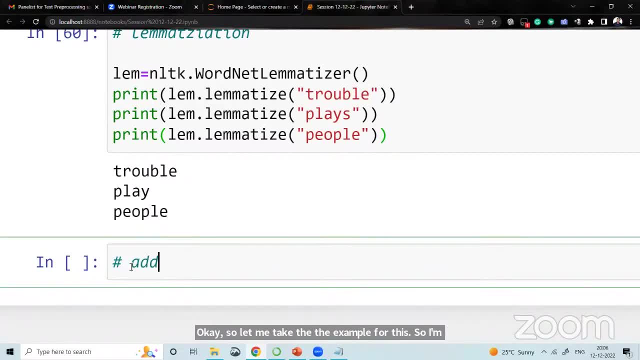 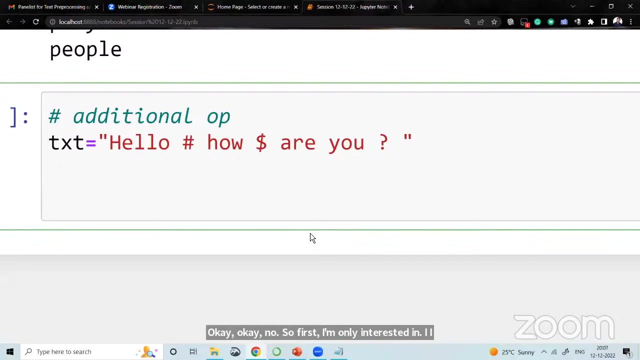 So I'm considering one text, additional operations. So txt, my sentence is like this: Hello hash, how are you? OK? question mark: OK, there are some special character I'm adding here and all that. OK now. so first I'm only interested in: I would like to remove the punctuation from this: 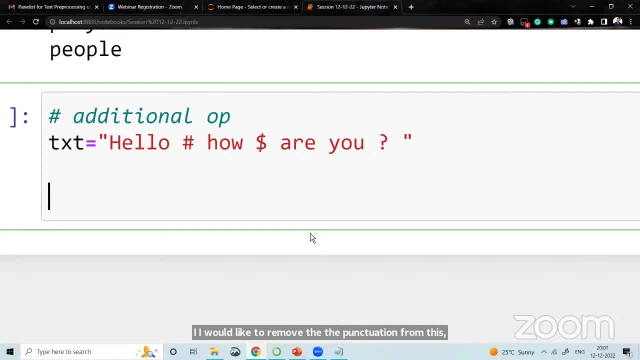 OK, so I'm interested in only alphabets. OK, so how to do this thing? So, to handle this, I'm writing the filter text equal to, And I'm writing here C for C, but in. and this is my text if you directly. go for the token first, 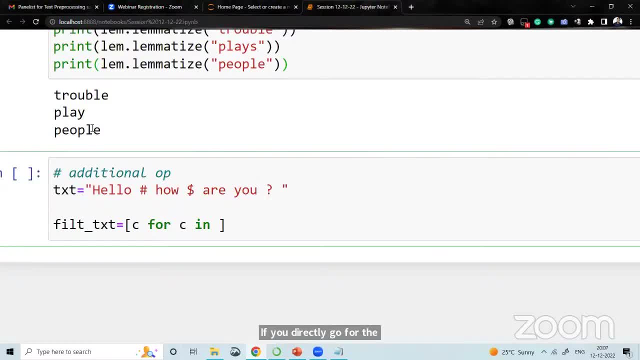 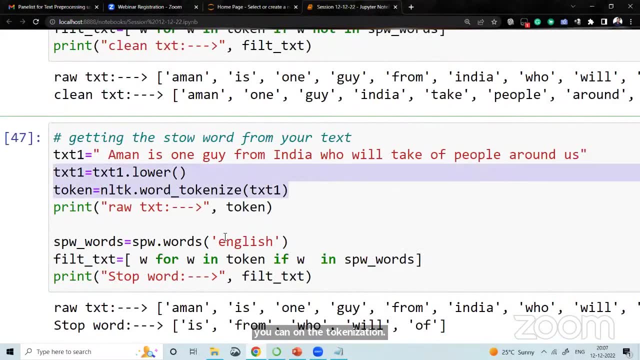 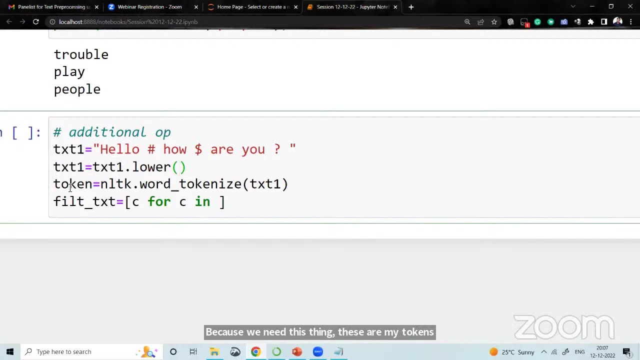 OK, so then you can go for the tokenization also, because we need this thing. These are my tokens: Txt1, I'm writing here txt1 tokens. So C for C in tokens If I'm writing here, if not, 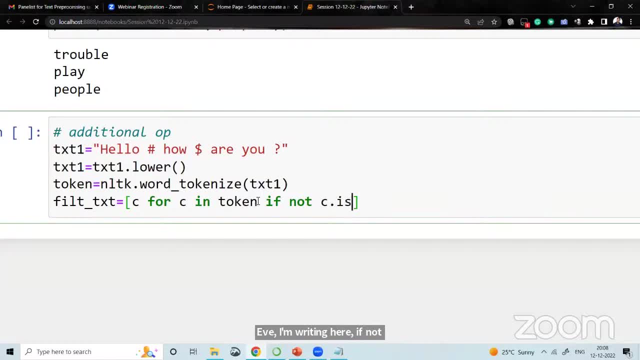 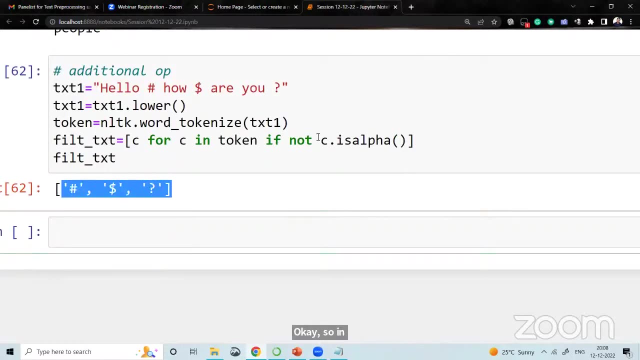 C dot is alpha. OK, OK, so this is what my special character, OK, but I want my text should be free from this. OK, so I'm writing here: if C dot is alpha, That means here I have removed this hash dollar symbol and question mark. 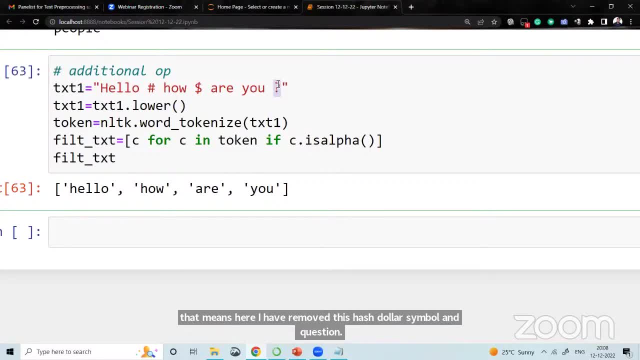 OK. so in most of most of the time, our text data contain this unnecessary punctuation. things OK like hash, pharma, dollar, OK. so these all are the punctuations or special characters which we, which we would like to remove. 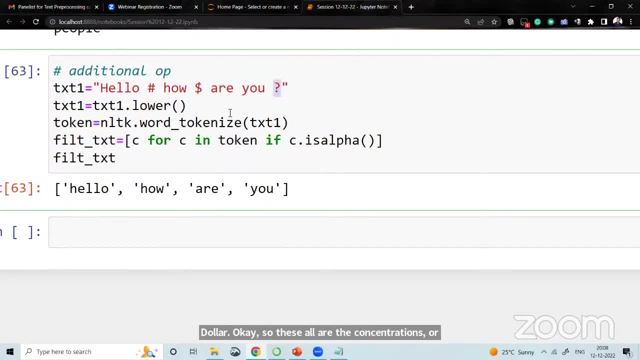 OK, OK, OK, We would like to remove from the text, so you can use this line of code to remove the, the punctuations. Similarly, so you can remove the numbers also. OK, so with this line of code you can remove punctuation and also numbers also. 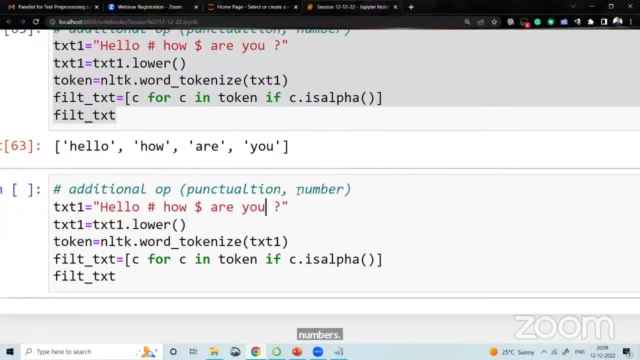 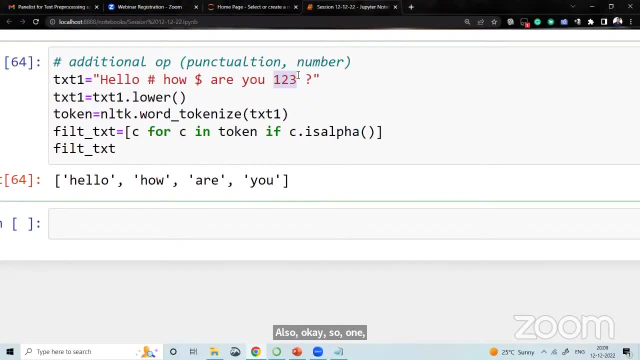 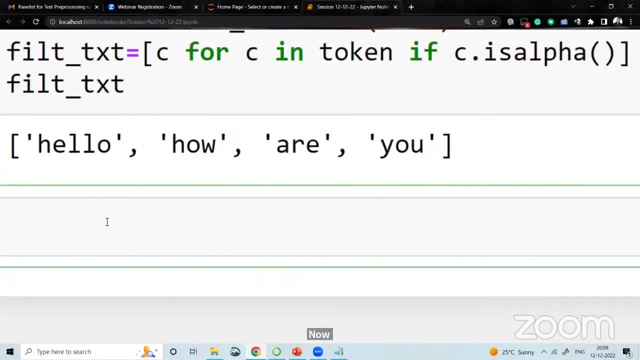 OK, let me write another example. I'm writing the numbers also, OK, so one, this one, two, three is also get removed because of this line. So I have written something else. OK, so I'm going to write another one. 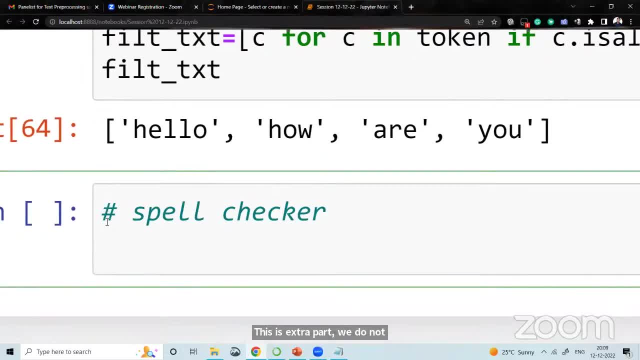 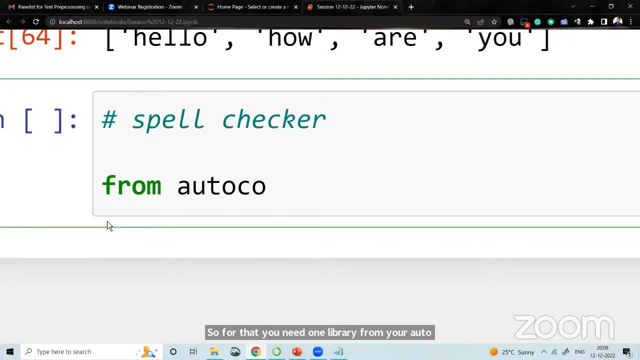 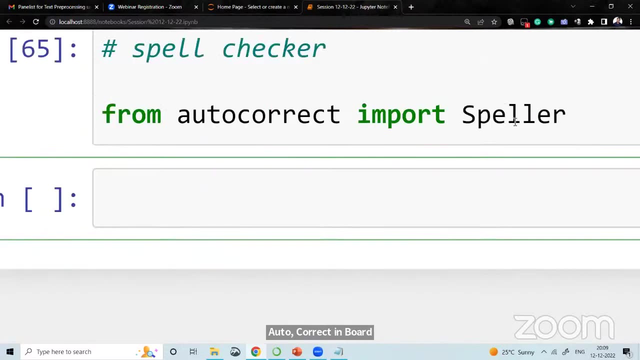 OK, so now I'm writing something else. OK, so this is the text. Now, next is very small thing, that is spell checker. This is the extra part. We do not use it regularly, spell checker, So for that you need one library from your auto, correct? 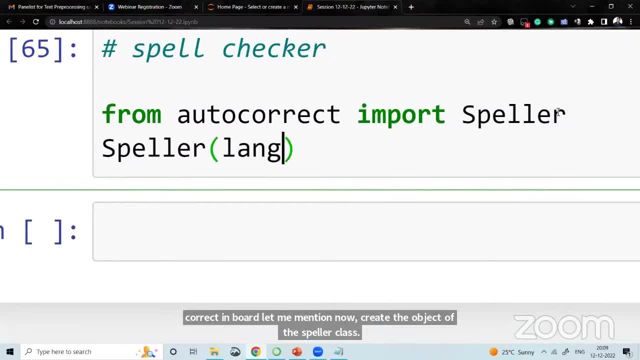 Auto correct import Speller class. Let me check. create the object of this Speller class. I đi tətələ tô həpələ keşide. I was trying to write it in English. You can use the English language. Language is equal to English and this is my object spell. 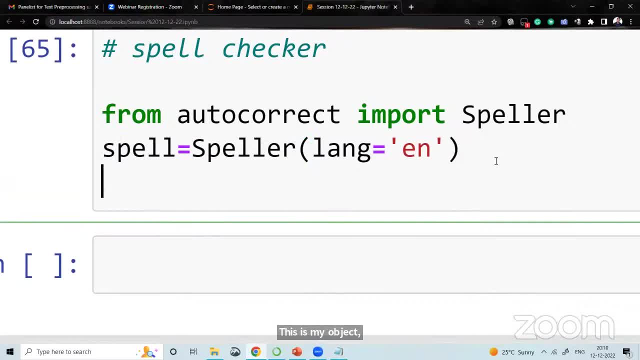 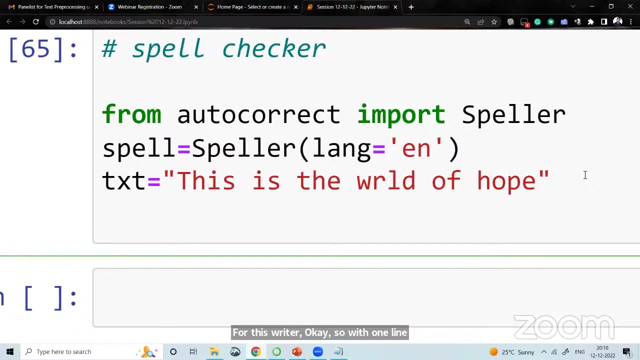 Now. then let's take the text I'm writing here. This is the world of WRLD, world of hope. Okay. now one word is wrong over here. The spelling is wrong for this: WRLD. Okay, so with one line of code you can correct this thing. So first go for the. 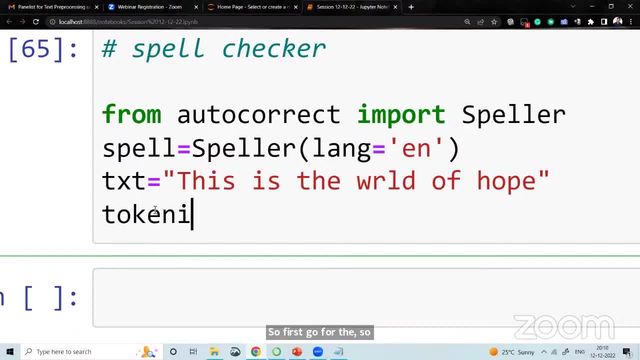 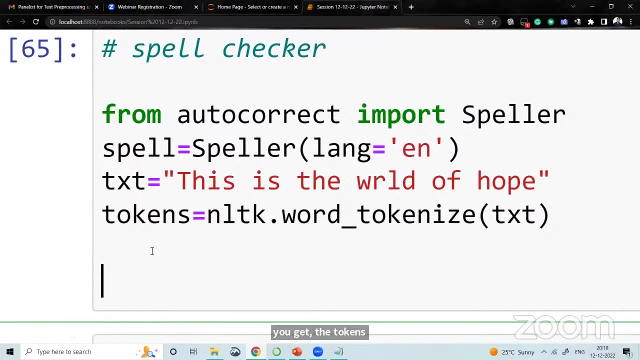 tokenization: Okay, tokens. NLTKword. underscore- tokenize: Okay, you all know how to go for the tokenization. and this is your text: Okay, you get the tokens, Then your spell, the correct spell. Okay, then you can write spell of your W. 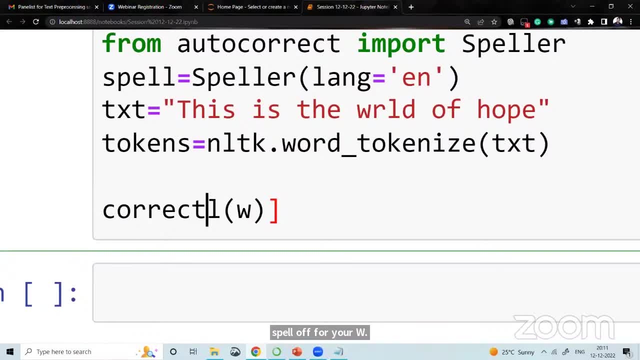 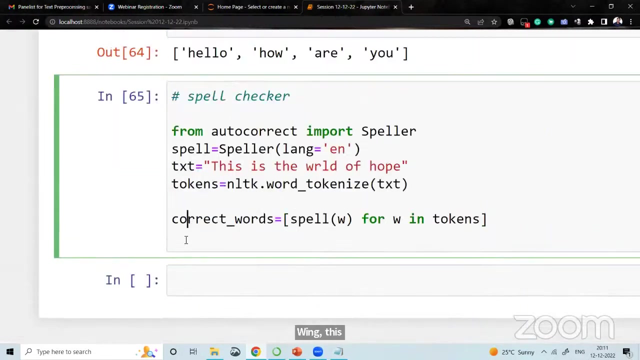 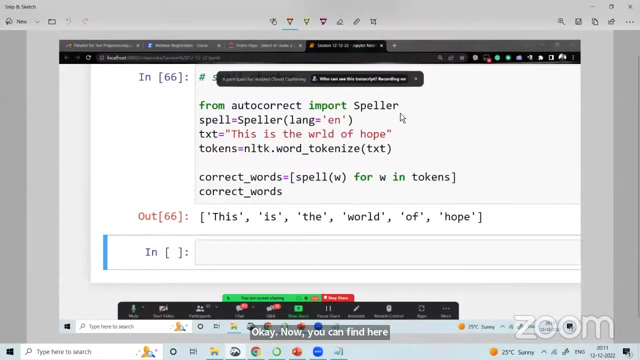 Let me write here correct word, Correct words. Spell of W- W in this tokens And print the correct words. Okay, now you can find here automatically with the help of this class We can correct. We have corrected this word. WRLD is now get converted into the WRLD. 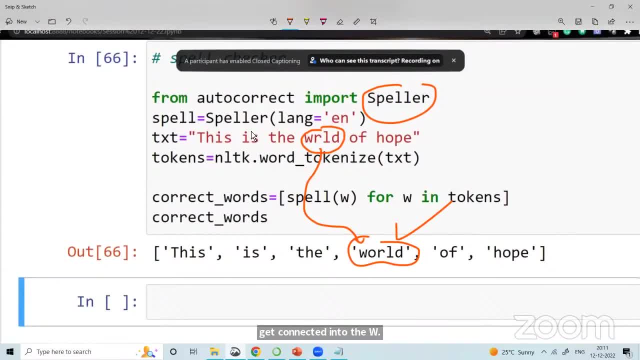 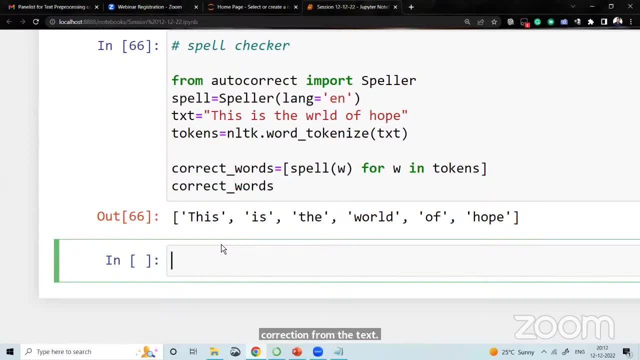 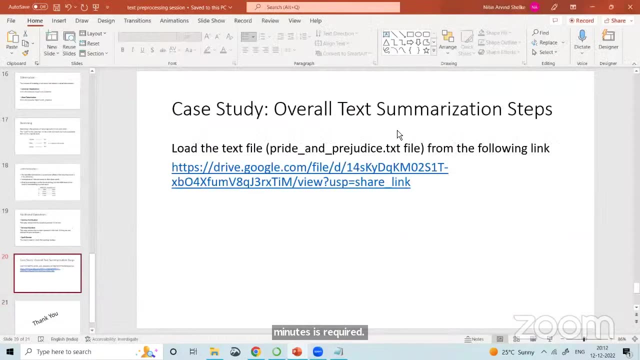 Okay, so this is how you can do the spell correction from the next. Now our last part is the test case. Okay, so 5 more min is required and just to complete this case study, Overall text, summarization text. so first you need to download this press text file after the class. 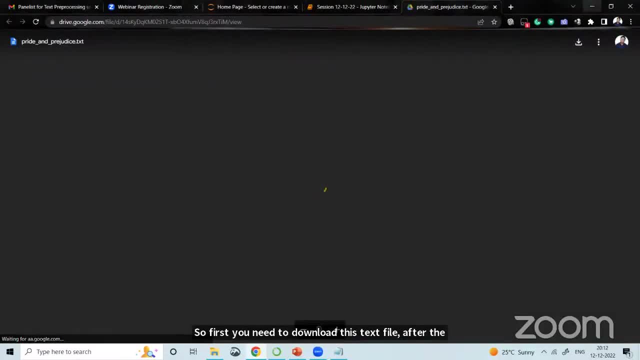 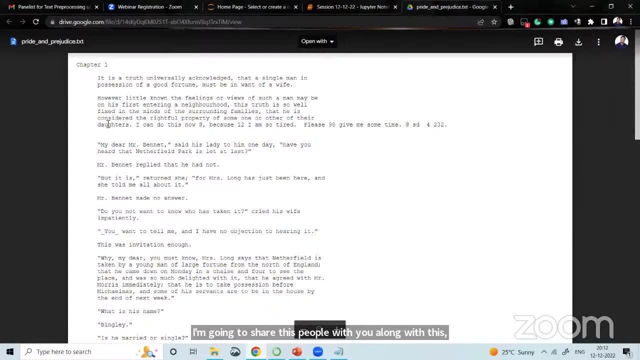 I'm going to share this PPT with you, along with this IP'ynv file, The PDF file. Okay, So this is my textbook. Alright, So basically, this is why enash has explained which one to my text you need to download. okay, after downloading it, just placed it into the root directory. 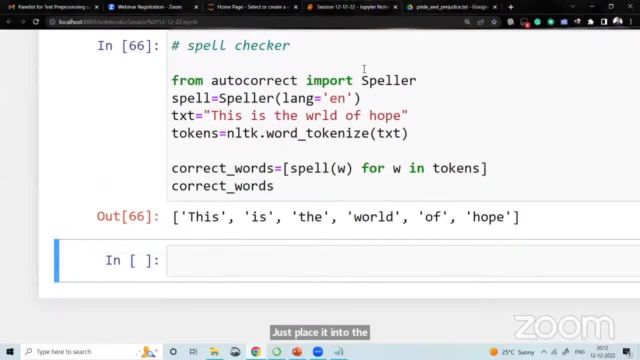 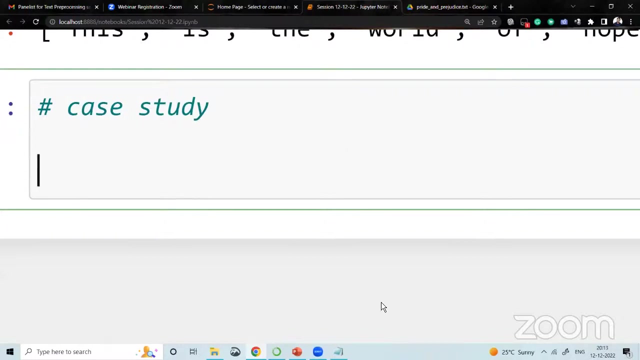 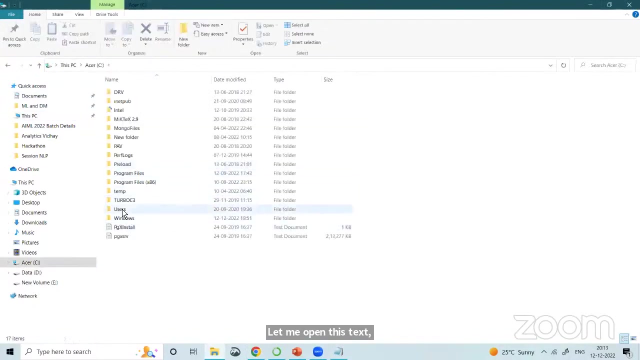 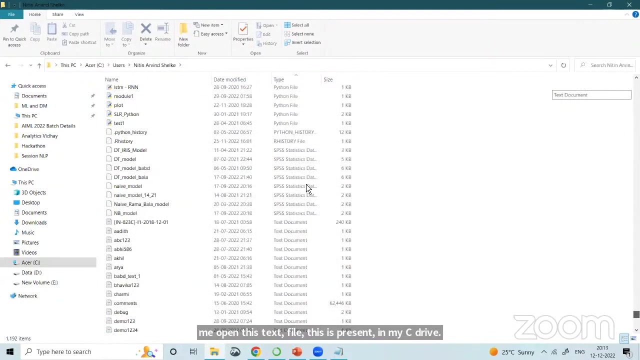 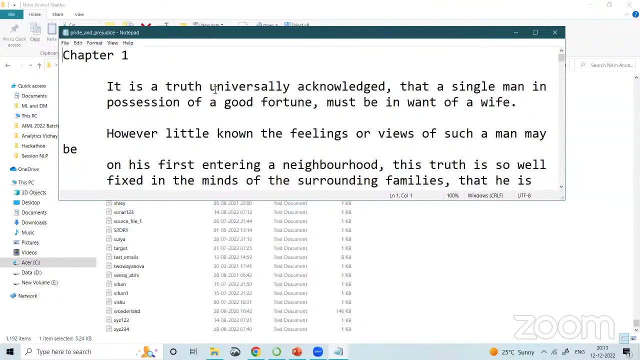 okay, just drag and drop into this root directory and then go for the the operations. okay, so this is the process that you need to perform. okay, so the case study. so let me open this text file. this is present in my c drive. okay, this is my text file. okay, and uh, i would like to perform all this text preprocessing. 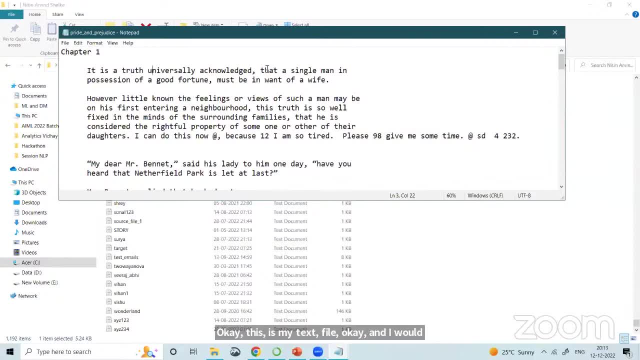 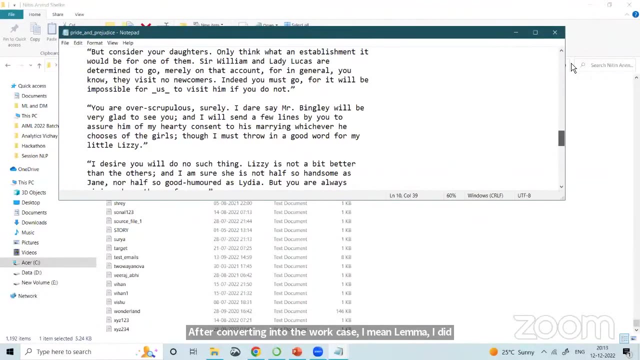 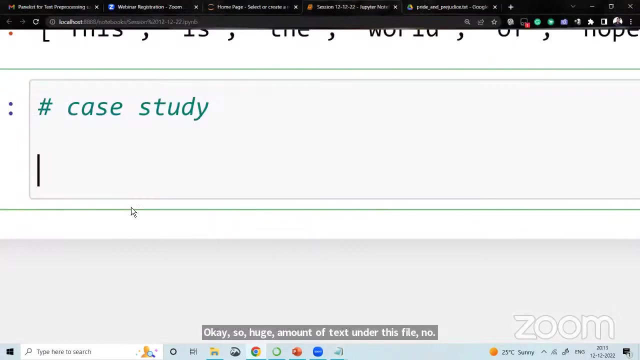 operations, that is, removing the special converter, converting into the lower case, i mean limitation, everything from this file. okay, so huge amount of text under this file now. okay, so this is my c drive, let us go for this. so what thing? i'm just creating the, so i need to type all these things. okay, it will take five to ten minutes more. pre-process. 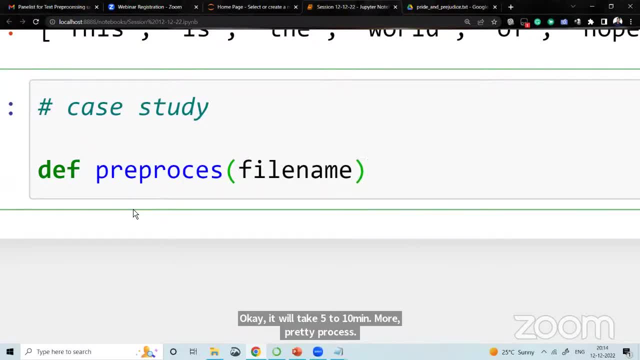 my file name. i'm creating one function under that i'm writing all the steps. okay, that will be easy then. uh, instead of writing the things in the separate manner, okay, let me take my file. okay, with the help of open function- this is the basic operation under the python- to open the file. so the file name. 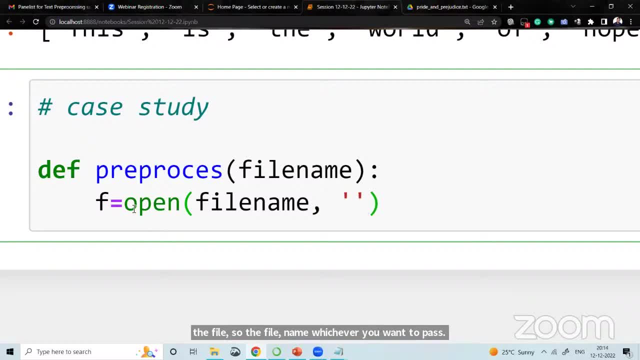 whichever you want to pass file name, you have to open it into the the mode. okay, i would like to open it into the read mode. i'm writing: the encoding format for this particular file is utf. this is optional. you can write utf-8 or something, okay, so i'm going to type the xf file into the file. 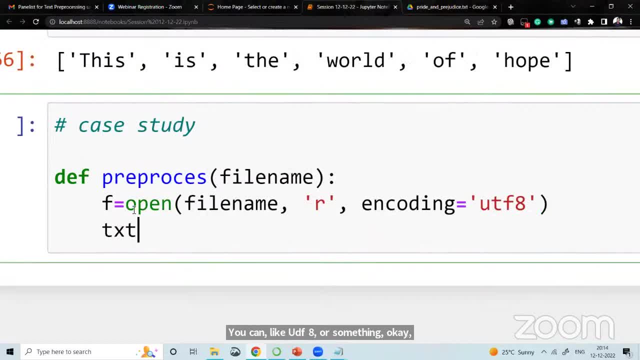 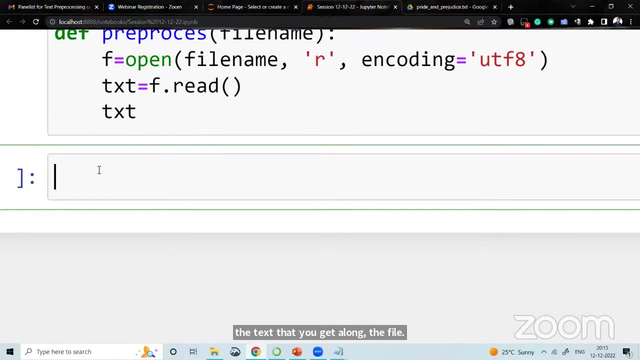 then read the file, appread. so this is basic python file handling. okay that we are doing it, and so this is the text that you get from the file. okay, let me execute this function. first the simple function, and i'm passing the the file name pre-process. 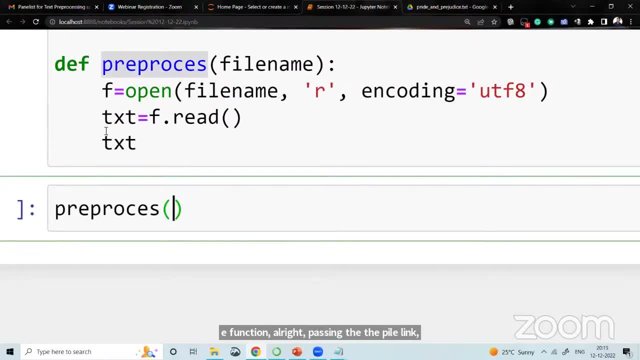 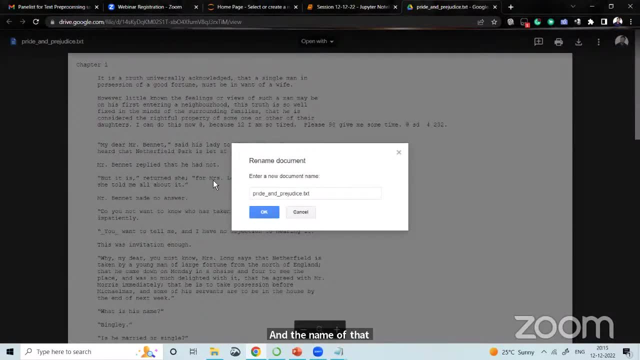 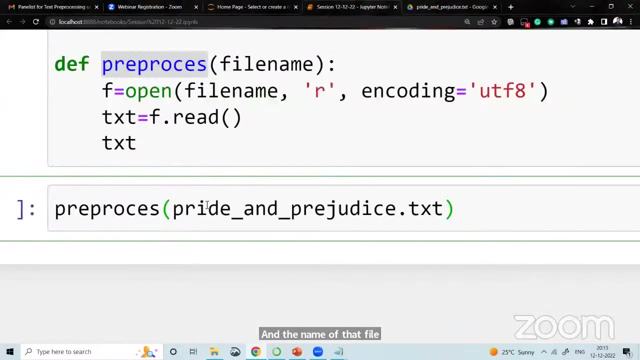 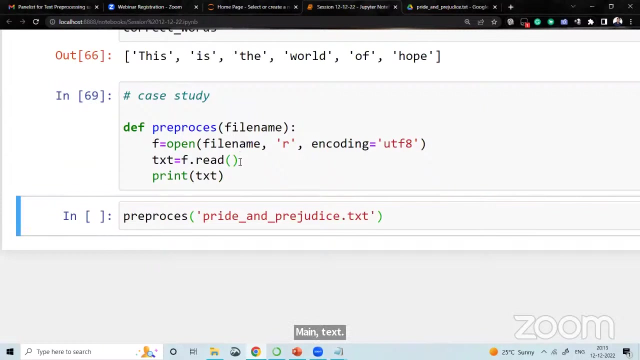 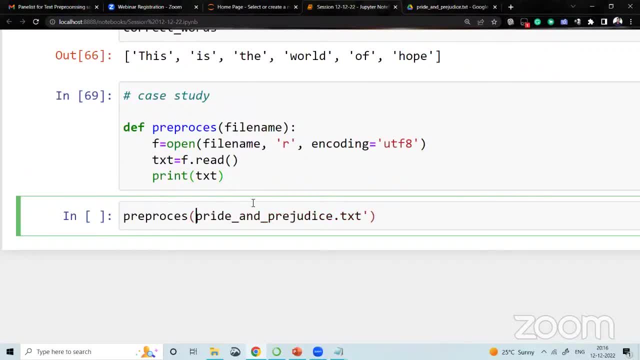 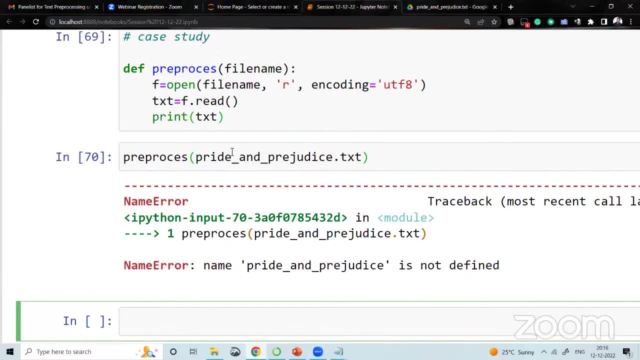 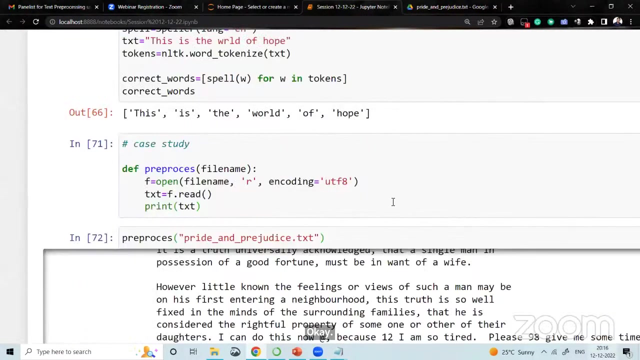 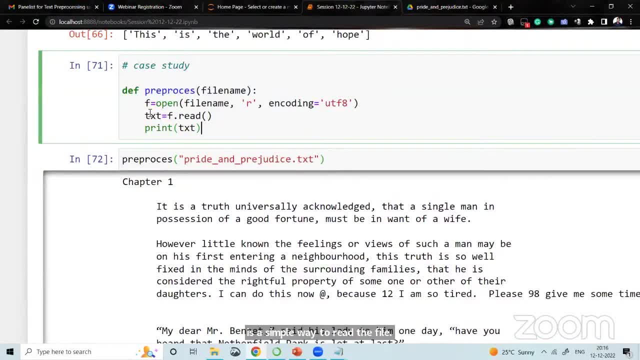 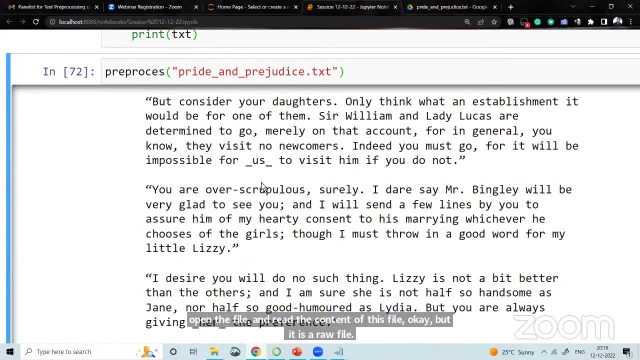 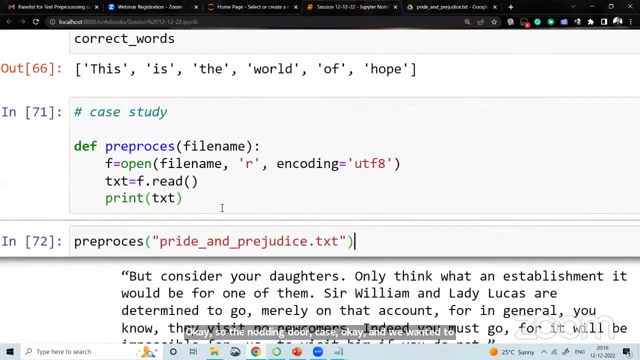 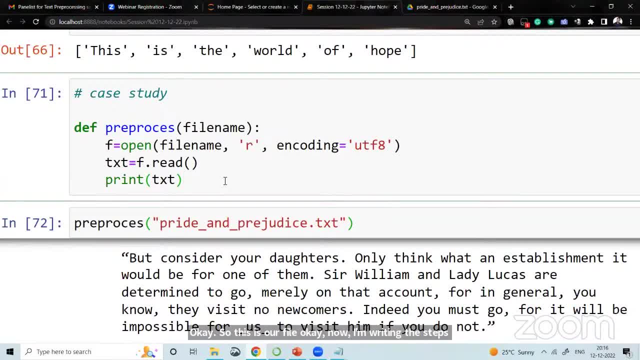 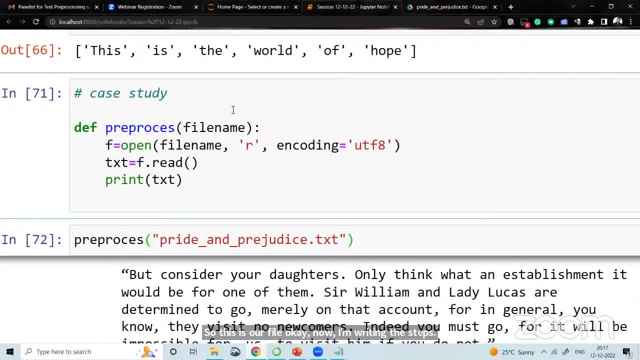 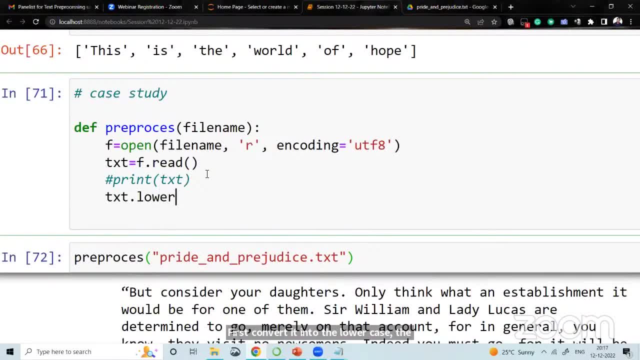 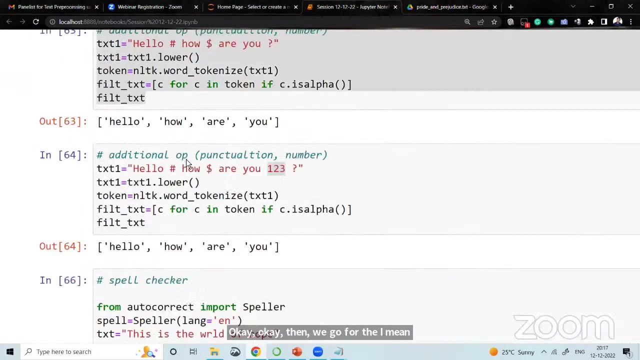 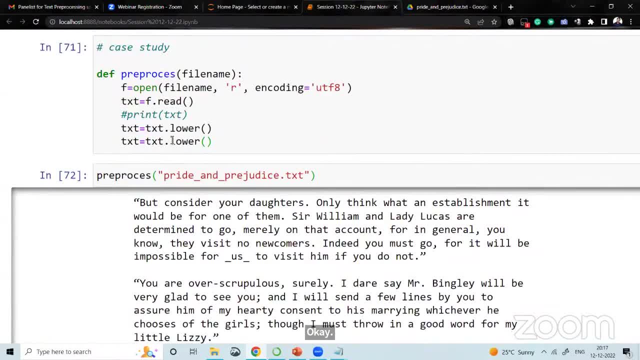 okay, so i'm writing this one here. i'm passing the, the filter text: punctuation- punctuation i am going to remove here and as i want to convert it into the, the text file, so i'm going to use the dot join method also: dot join okay now. so this is my filter text. 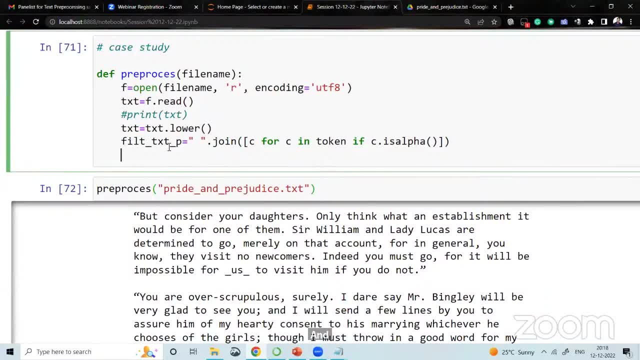 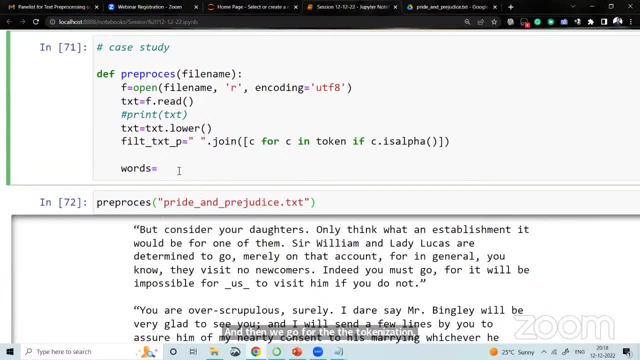 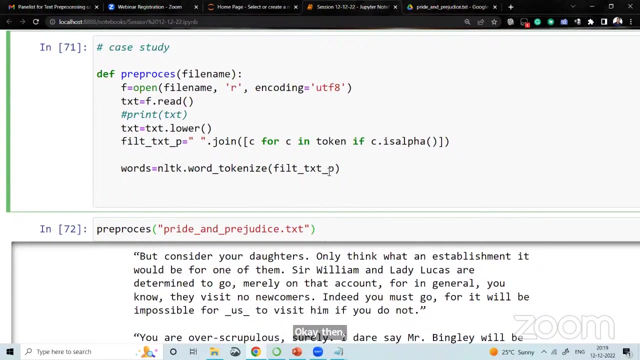 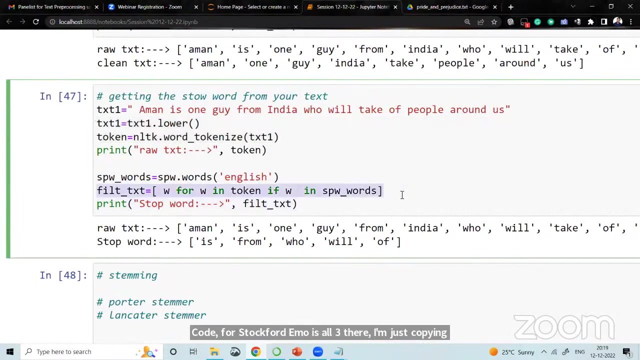 and then we go for the, the tokenization words: nltk, dot. word underscore tokenize. okay, word underscore tokenize and pass the filter text. okay, then stopword removal. code for stopword removal is already there. i'm just copying and pasting out there. okay, this is the code for the smartphone removal, one line of code. 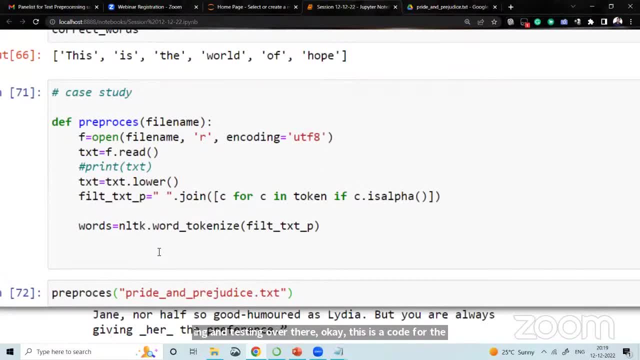 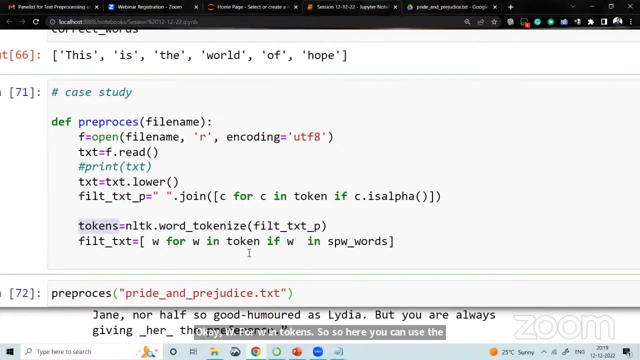 so i'm just going to copy and pasting out the code. okay, so i'm just going to copy and pasting out the code. okay, w4win tokens. so so here you can use the tokens. okay, and then steamer, okay. so, similarly, you can go for the steamer. similarly, you can go for this. 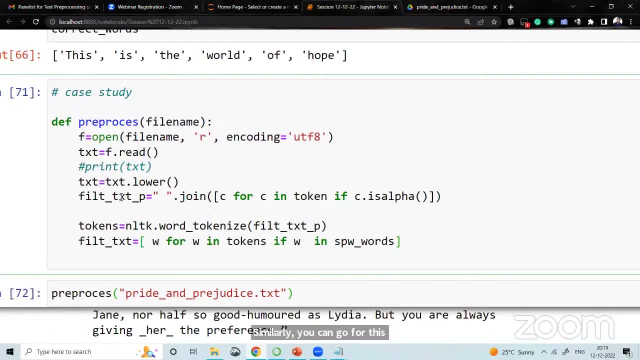 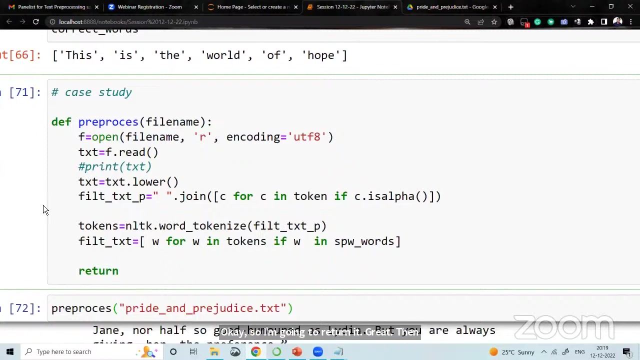 lemmatization also now. right now i'm just printing these three things: okay, the the text after remove the punctuation and then filter text. uh, after doing the uh stopword removal. okay, so let me complete this one. okay, so i'm going to return it written. so first i would like to return the normal text. 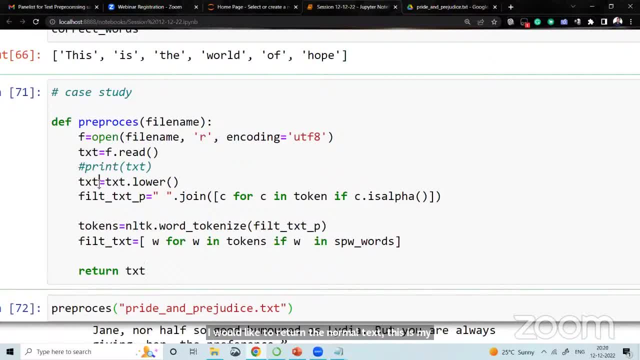 this is my normal text. this is my lowercase text. okay, lowercase text. then my tokens. okay, then my filter text. filter text means after removing the stock code. okay, so these four thing i'm going to uh filter it out, right, uh, similarly, you can go for the streaming lemmatization concept. 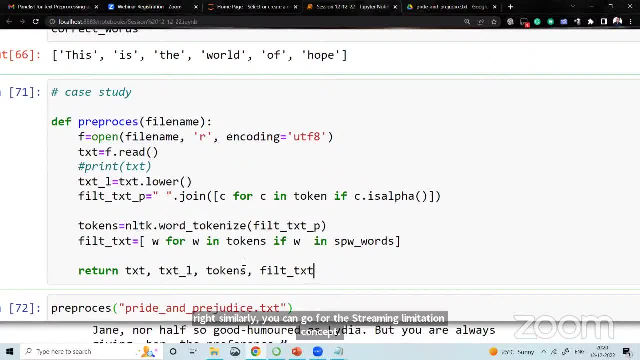 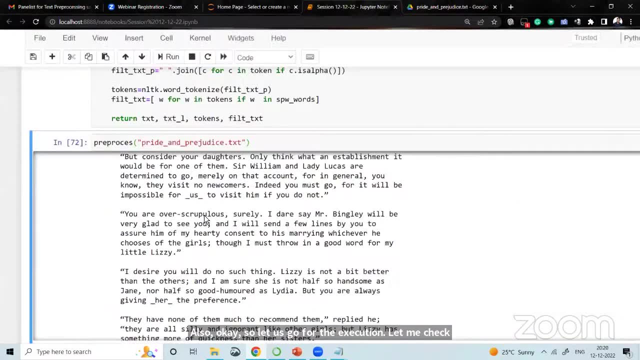 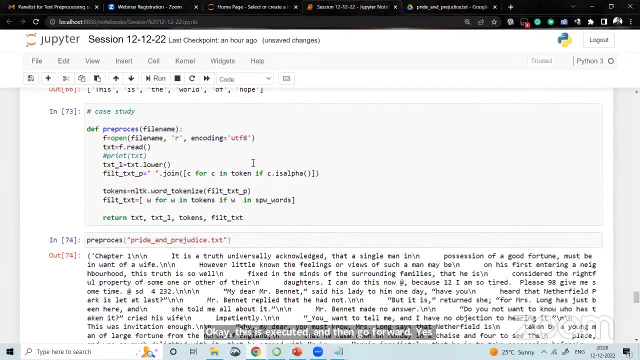 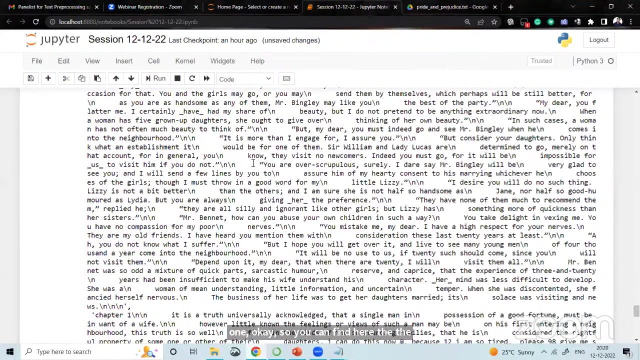 also okay. so, uh, let us go for the execution. let me check tokens and all, okay, this is executed. and then go for the yes one by one. okay, so you can find here the, the result that i'm getting the first initially, i'm getting the raw result. then 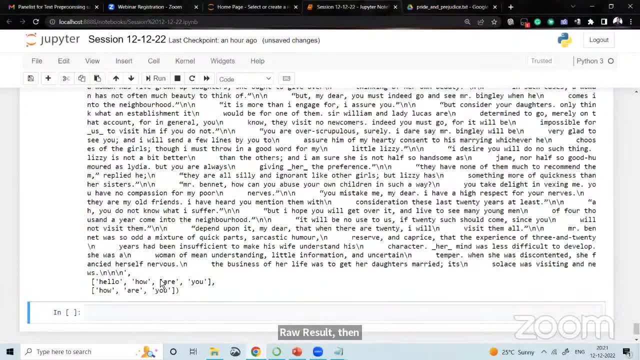 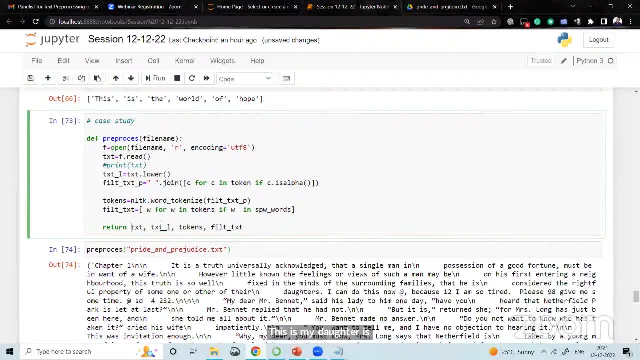 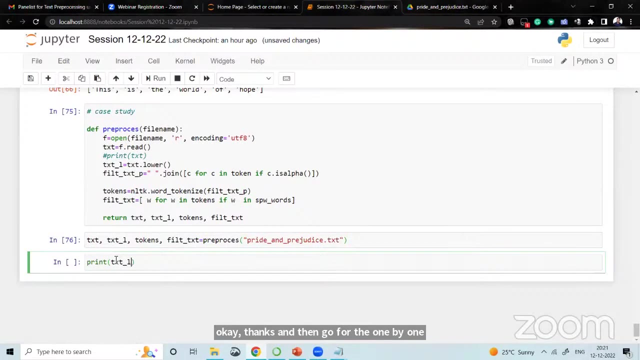 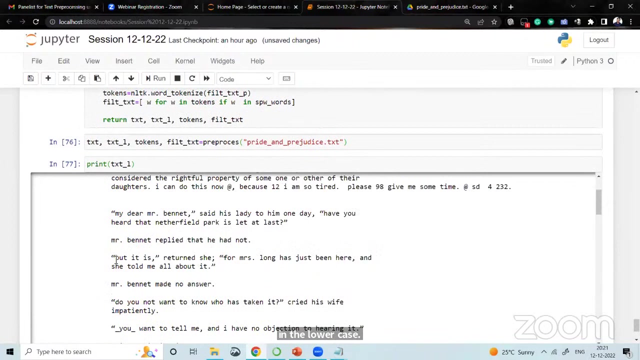 this is my raw result. this is actual text. um, I'm going to store it into this. it is stored like this: okay, filter text and then go for the one by one. this is tht underscore lower. all the text is in the lower case. okay, you can check. all the text is in now lower case. 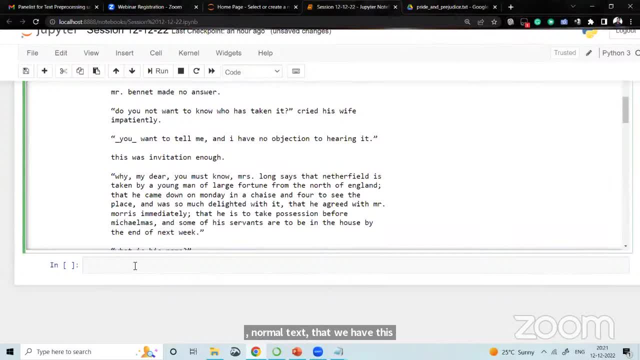 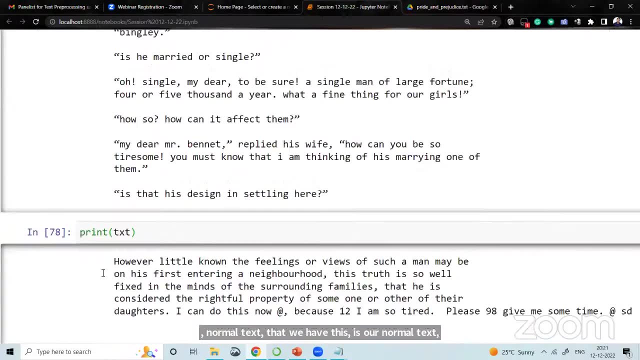 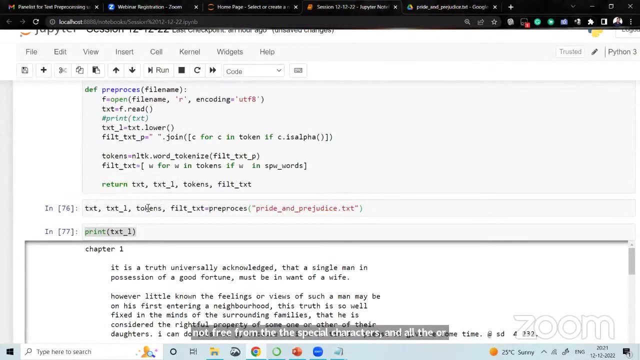 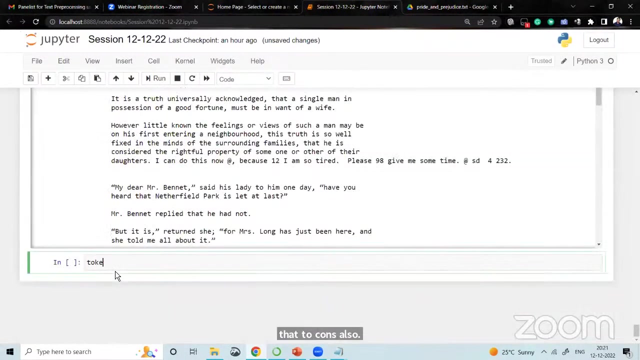 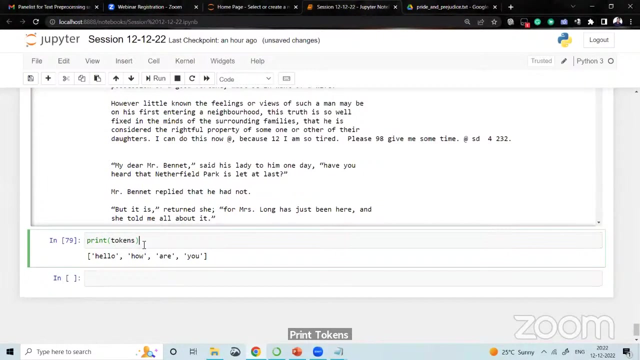 normal text that we have. this is our normal text. okay, this is our normal text means normal text means not free from the, the special characters and all not in the lower case, also okay. and also you can print the tokens also. print tokens, okay, sorry, uh, okay, okay. 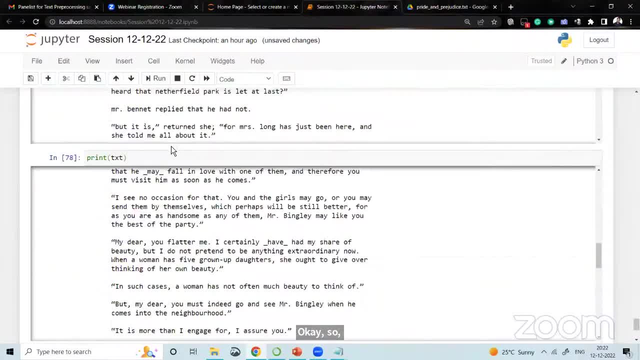 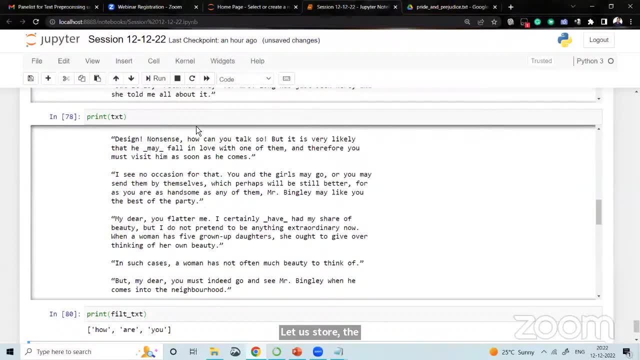 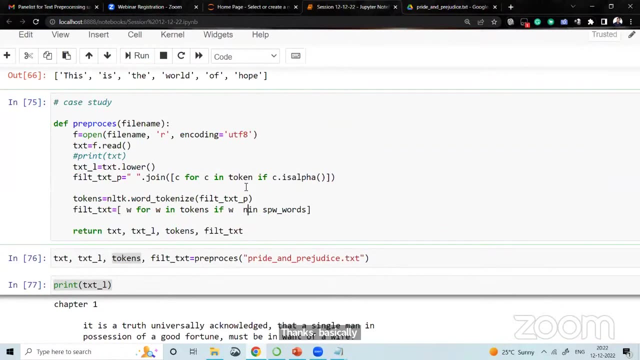 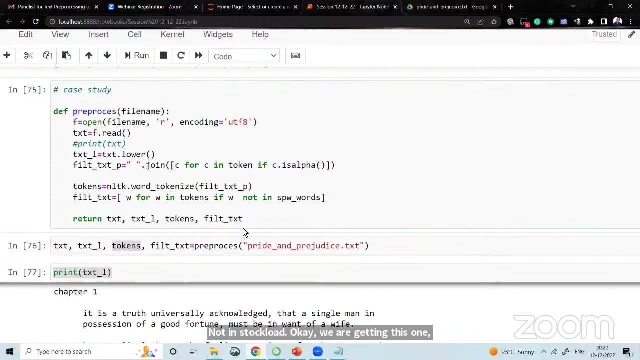 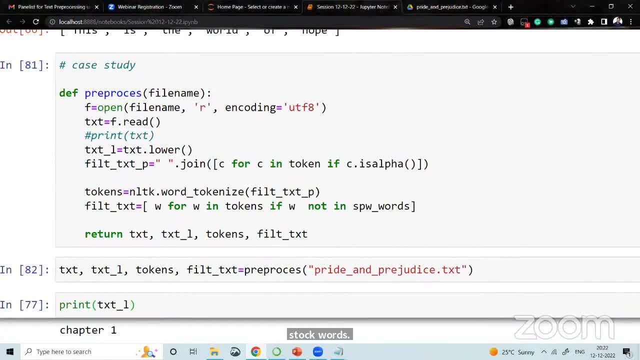 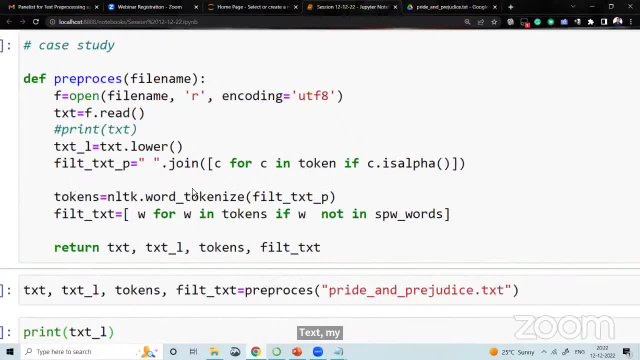 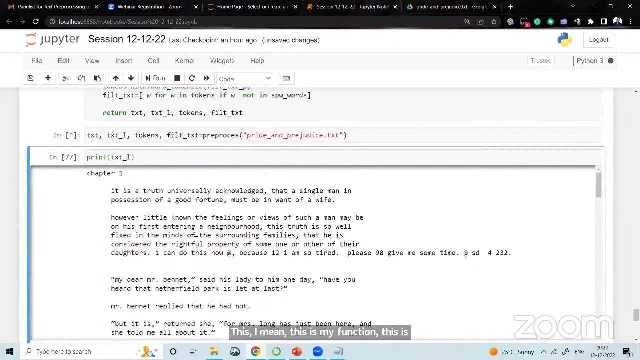 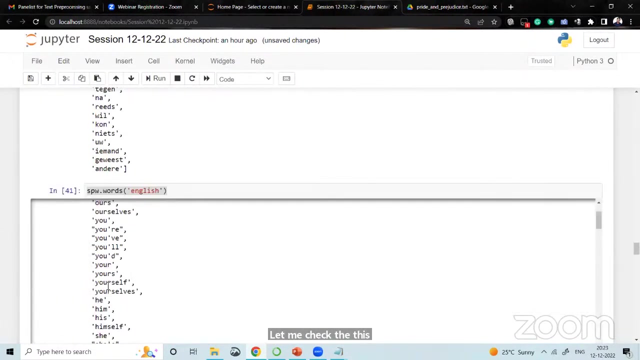 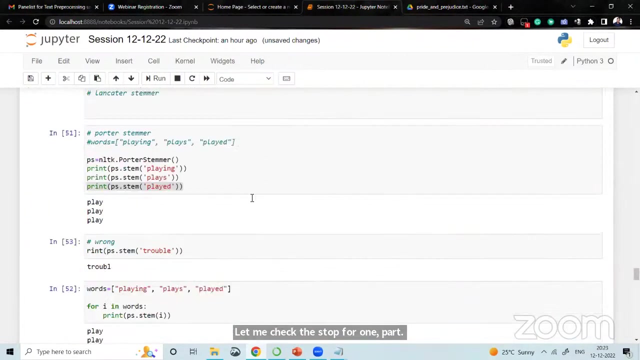 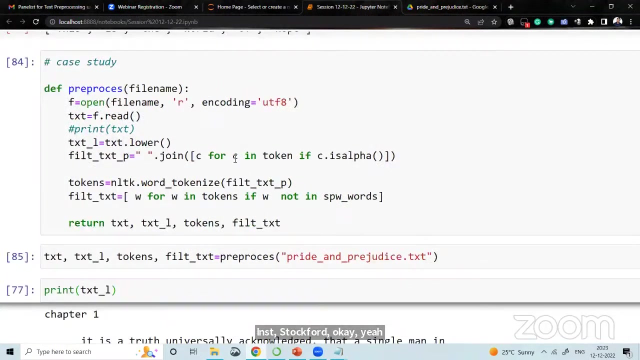 actually it is considering the past text, my past text. it is considering- so let me figure it out- this file name. this is my function, this is my reprocessing. let me check the stop word. one part in stop word. okay, yeah, see for see in tokens. okay, this is i, i'm just. 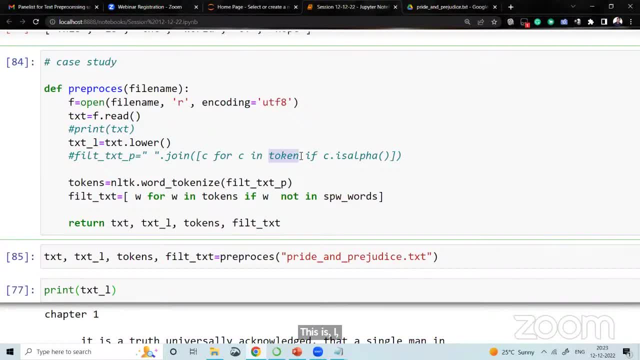 commenting out this: okay, uh, because this token is on, we have considering the previous token, okay, so that's why i'm just going for the normal text. okay, this is our normal text. this is my text after lower casing, and then filter out the text after aiming the stop word. okay, these three. 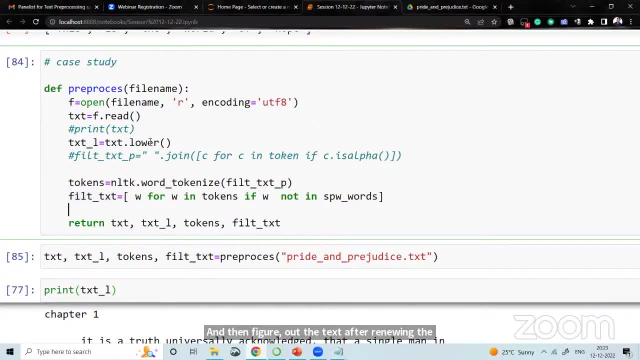 things i would like to print over here. similarly, you can go for others: normal text, dot, lower nltk, dot. word underscore, tokenized and pass this one. okay. um, i commented out this one first. okay, now i think we'll get the correct output filter text text: l token. we do not. let us go for this now. okay, this is our normal text. 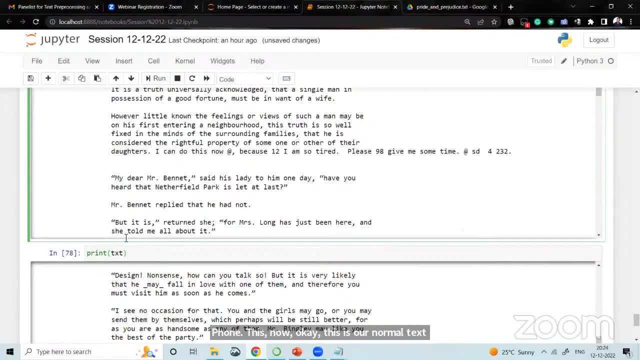 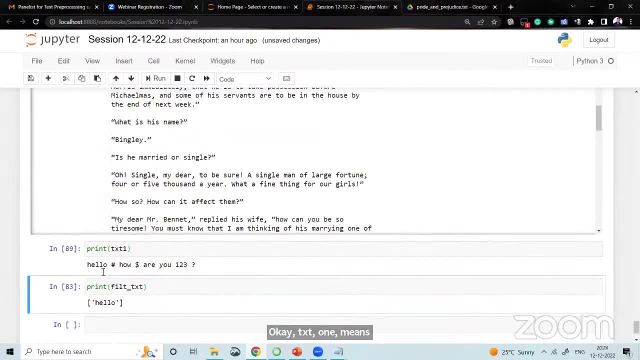 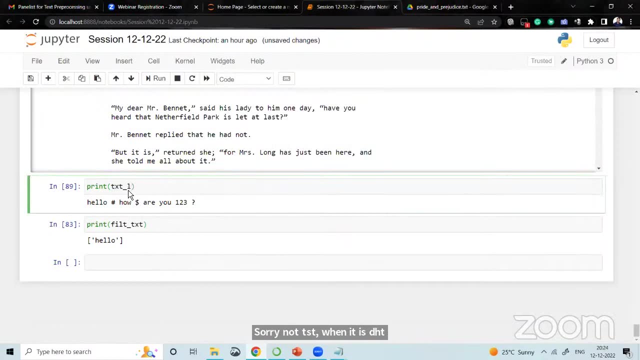 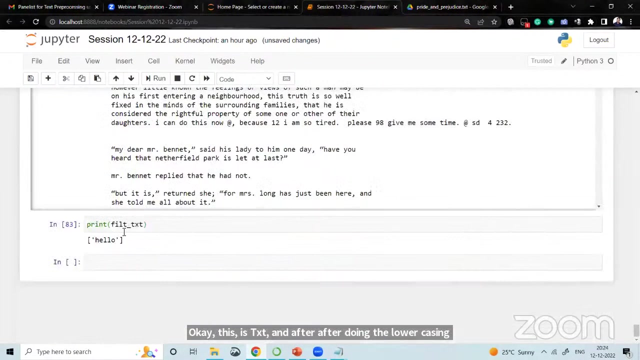 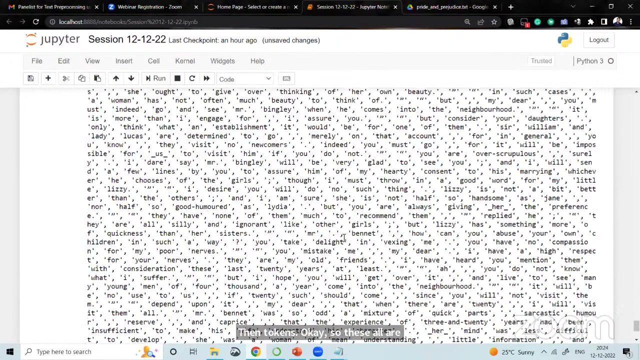 then we go for the txt one. okay, txt one means sorry, not txt one, it is txt. underscore l: okay, this is txt. and after in, after doing the lower casing, and then tokens, then tokens. okay, so these all are my tokens from the the, my text file. okay, now it is working okay. 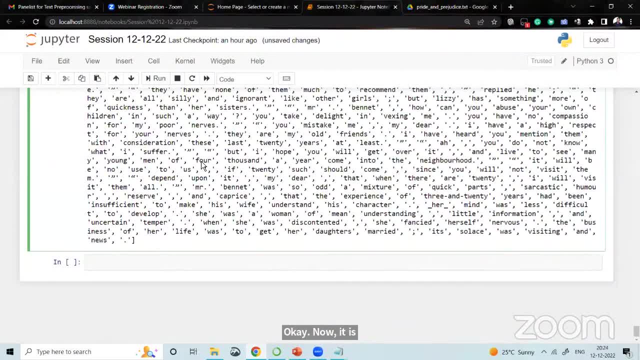 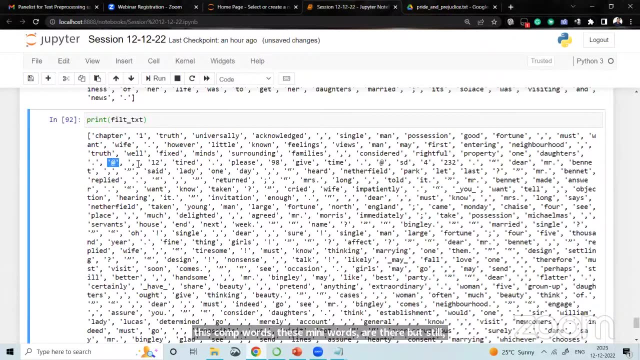 and then, finally, we have filter text. okay, so the filter text means that is, after removing the stop words, okay, after removing the stop words, these minimal words, after removing the stop words, these minimal words, words are there, but still we have these things. okay, that we can remove. okay, so how to remove? 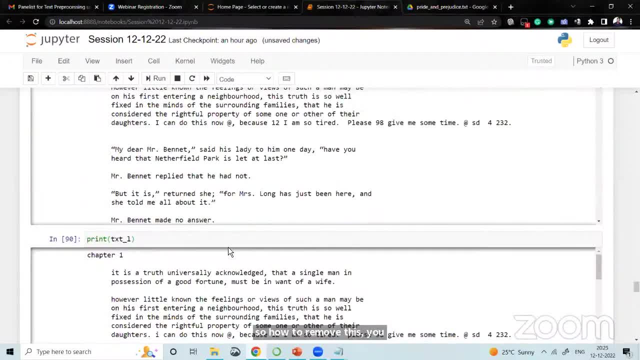 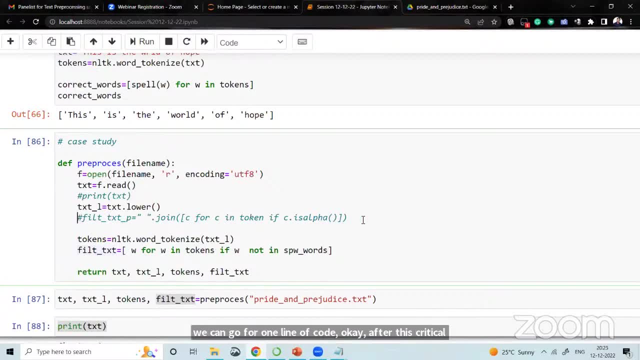 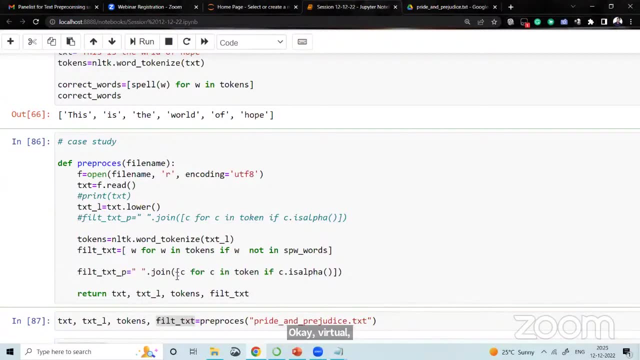 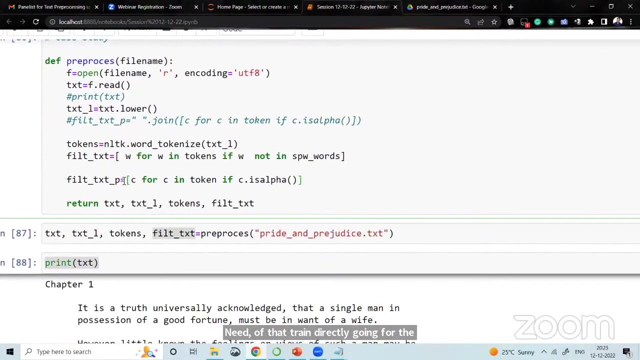 this. you need to write one line of code for this. to remove this, we can go for one line of code. okay, after this filter text, you can write this: okay, filter text p, then dot joins- uh, no need of dot join directly, going for the list of word itself. and here you can write and print: 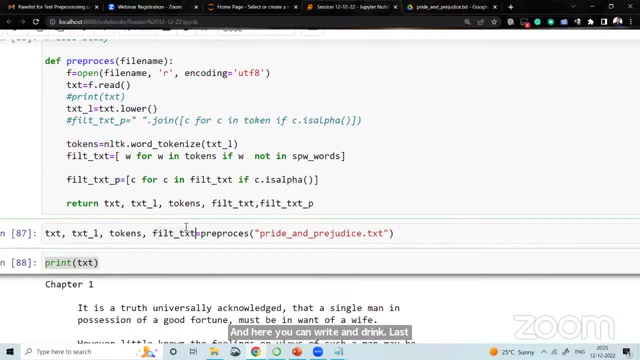 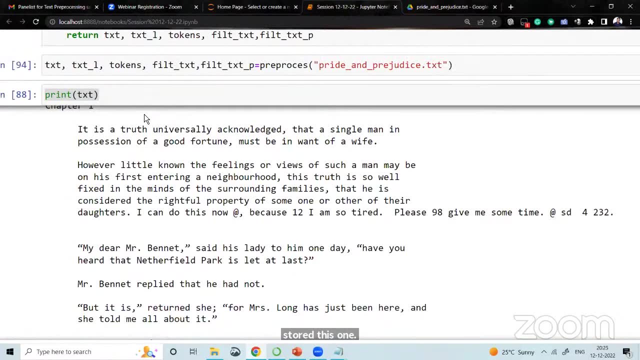 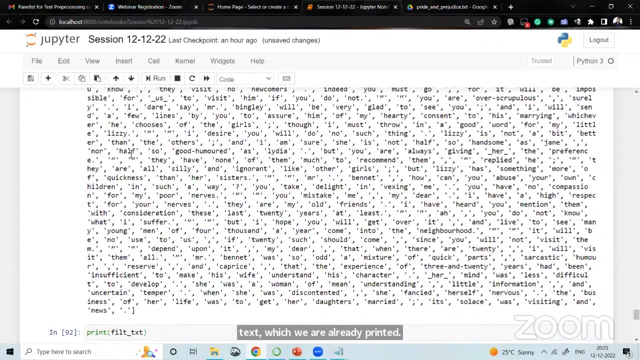 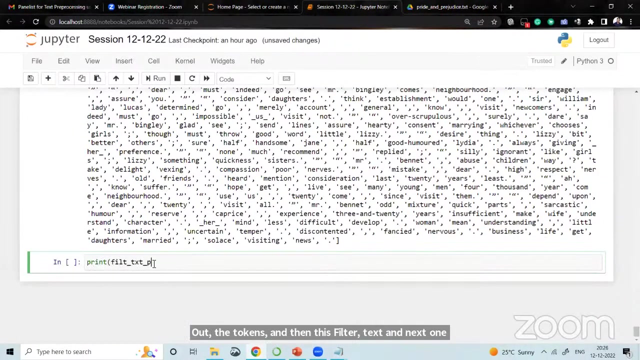 lastly this one and store this one. okay, now we execute. execute, so this is your normal text, which we have already printed out, the tokens, and then this filter text, and next one is filter text p, after removing the punctuation: filter text: after removing the punctuation. now this is: 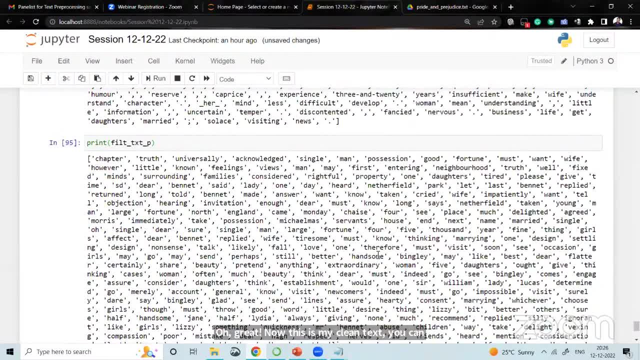 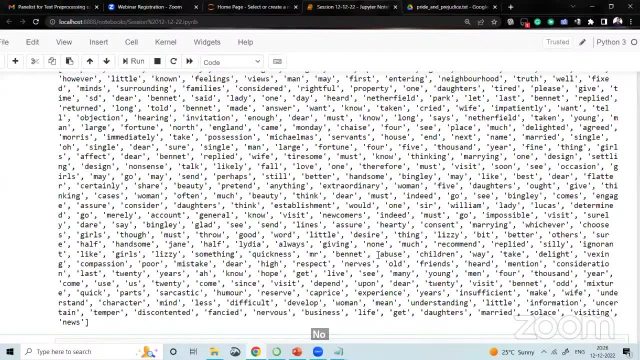 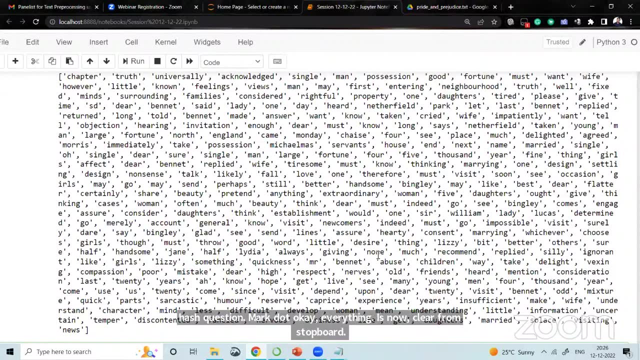 my clean text. you can see over here. no special character is over there. no hash question mark dot. okay, everything is now clear from stock word. all the text is in the lower case: okay words. already we have organized similarly. you can add the steaming code: lemonization. 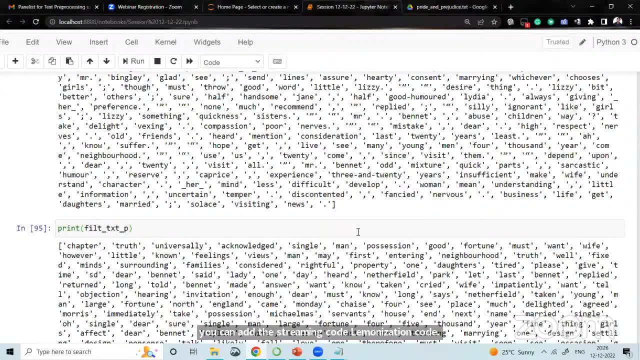 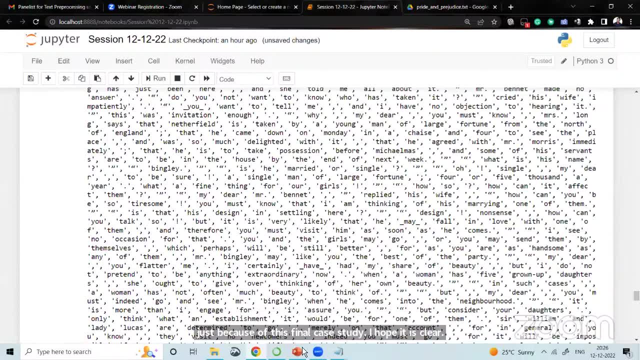 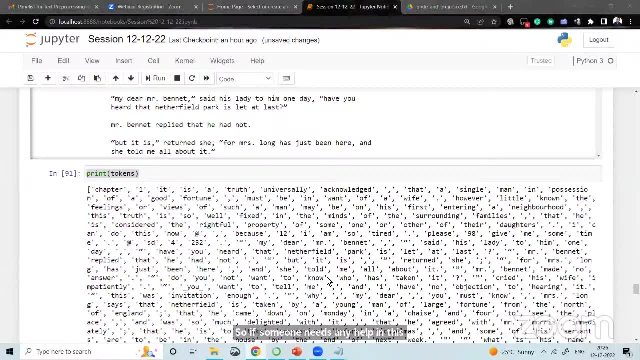 code. okay, i hope it is clear. i have taken 10 minutes more just because of this final case study. i hope it is clear. if you are having any doubt, you can ask me. okay, i am going to share my email id also if someone needs any help in this nlp. so let me share the okay. 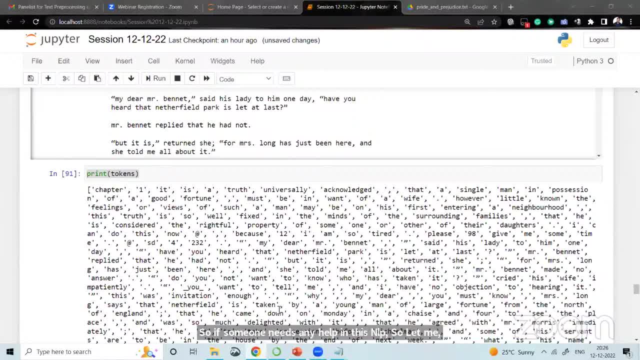 i think i'm going to share my email id also, if someone needs any help in this nlp. so let me share the. okay, i think i'm. let me share the. okay, i think i'm not having any access of typing. Let me check it And just get it: Netenahelkecom. So under 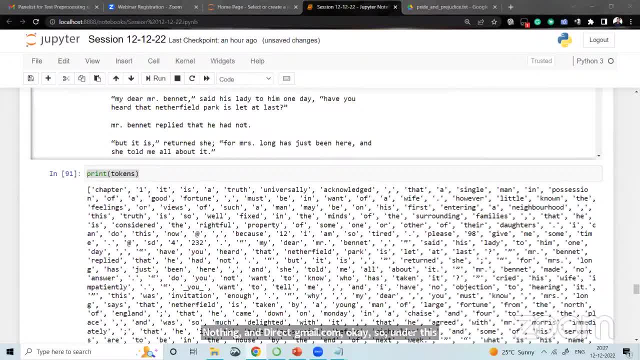 this session we have covered the text preprocessing part that is required for the NLP project. We discussed how to convert the text into the lowercase, how to remove the stop words, doing the tokenization, performing the steaming lemmatization, removing the punctuations. 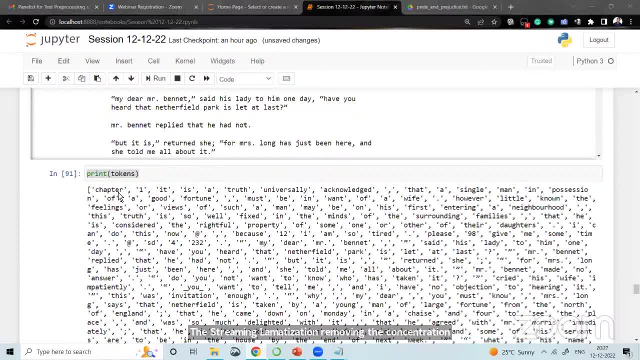 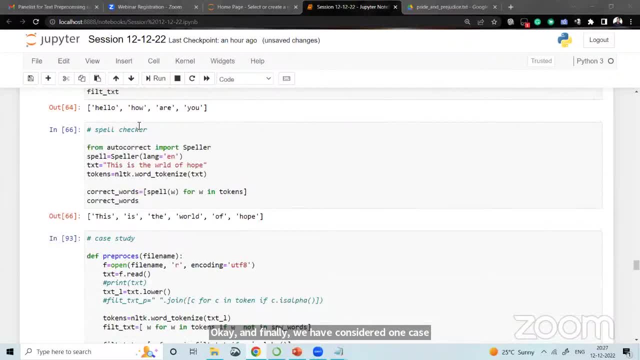 digits from the actual text And finally, we have considered one case studies from the text file. So there are many things under this, because I'm getting the questions, Let's see So many other things are also there, Like you can extract the data from website. 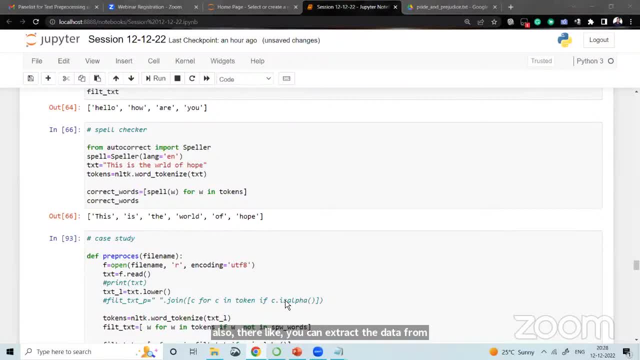 using URL, open and then go for this text. preprocessing operations also, But because of the time constraint I'm not going to take that particular part. Maybe in the next session I'm going to cover the web scrapping and the feature extractions tools like global. 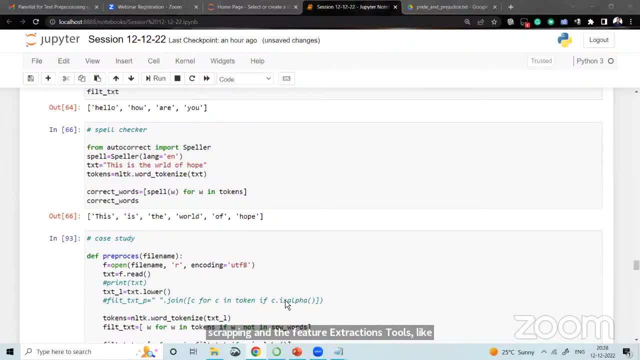 Go fast text word net your fast text and the bird part also. Some questions are there. What is lemmatization? Lemmatization is for the getting the root word. Okay, Just to, as I told you, playing, played, and plays is having a different meaning When we give this data. 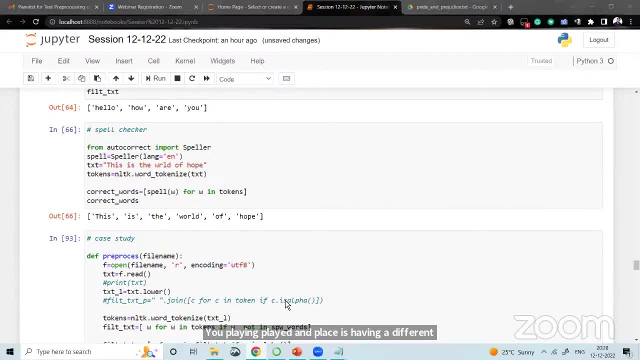 to your model. okay, the different vector is get generated and all three words are taken it as separately, Although all the three word is having the same meaning. okay, so for that purpose you need to go for the root word, for any root word, for example, 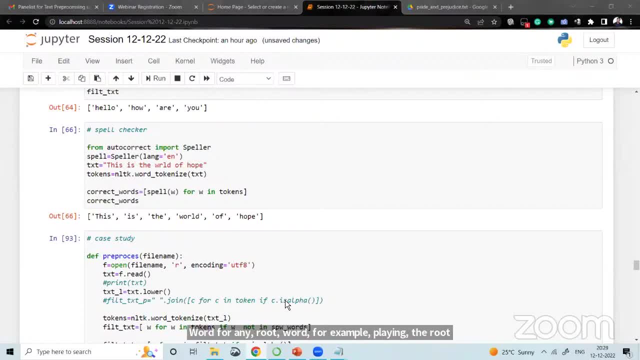 playing. the root word for playing is play, played. it is play, okay. so for that we have two option: one is streaming and another one is lemmatization. okay, so i hope everything is clear. yes, yes, thank you. before we proceed to answer your questions, i think i would like to request the attendants. 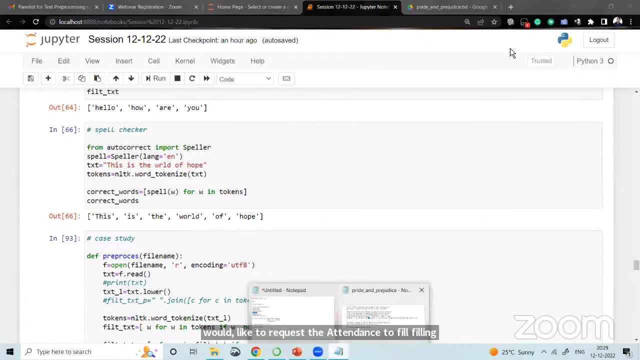 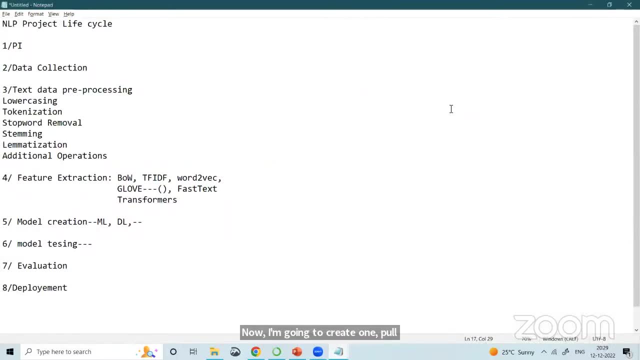 to fill. fill in the poll about feedback, as it helps us to conduct more such sessions. now i am going to create the one poll. now you can take the questions some people ask in the qa sections. yes, so there are different questions. uh, like transformer and transformer is again. 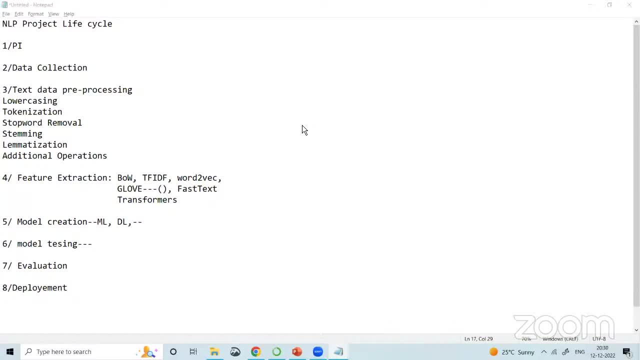 basically, we use it for converting the. there are the different use. okay, like: uh, we can use the transformers in different projects nowadays, in summarization, in sentiment analysis, we are taking the questions in different ways. okay, and then we can use the transformers in different ways. the help of this transformer, okay. so bird, are there the several versions of birds? roberta. 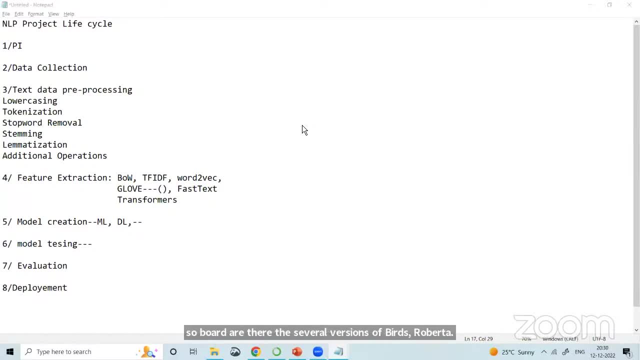 we can consider that we do not require the the basic feature extractions like bag of words or tf id of things. so some questions related with the notebook. yes, i'm going to share the notebook. so what if the word is having the abbreviations? so spell give the correct spelling. yeah, it is not. 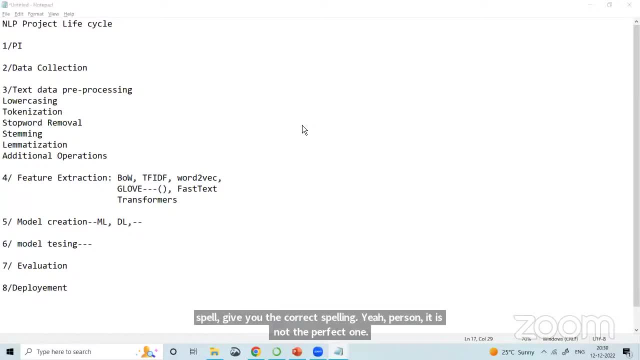 the perfect one. okay, sometime with spell class you have not get the correct result. also, it is as similar to your uh steamer, porter steamer and the lancaster streamer. every time you cannot accept the correct thing, okay, you need to modify that particular class or you have to create your. 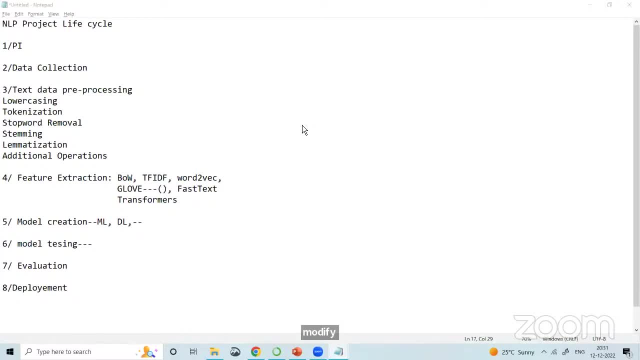 own. uh, how do you check the loading time and the speed of nlp execution? so nlp execution means the- and i don't know what you are asking- nlp related project. you are saying then, yes, if you do the proper pre-processing then you can improve the, the computational time that is required for the model training recording. yes, recording is there. 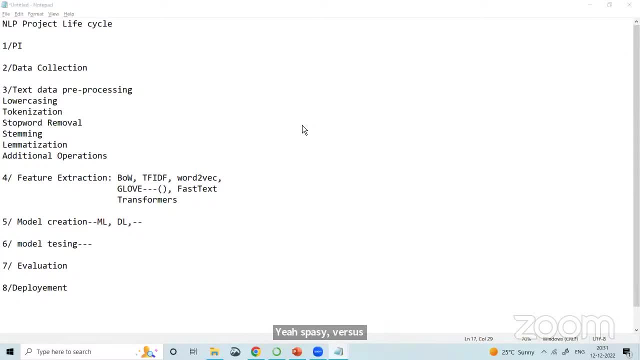 yes, spacy versus nltk. spacy is also the another library by which you can handle the the nlp related task. okay, but nowadays nltk is the most commonly used library. okay, so you can connect with the linkedin also. okay, i'm getting the request over the linkedin also. so if you face any issue or any doubt, you can just 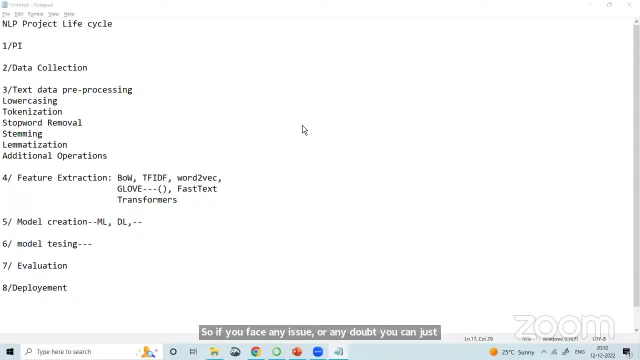 message me, okay, if i get i have already. okay, great, alien. is the number of words over here? okay? so when we talked about the alien for the nltk, then it is for the uh, the, the words normal, python, uh. if you apply, then it is character. yes, i think that much is sufficient already. uh.